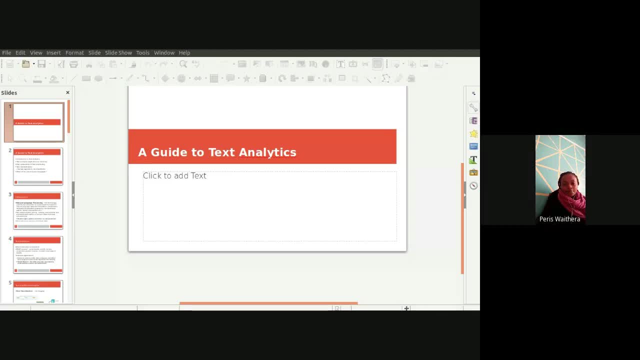 session immediately. Dr Lillian Manzari is a lecturer in the Department of Computer Science and Technology. She is a lecturer in the Department of Computer Science and Technology. Her research interests are in text analytics, Knowledge Extraction, Applications of Artificial Intelligence and NLP for Under-resourced. 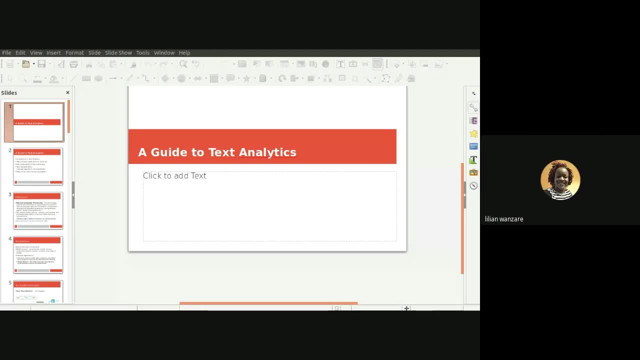 Thank you, Peris. Hi everyone, I hope you can all hear me As Peris has given a brief introduction. our main highlight today is just to try to kind of wrap our heads around the issue of text analytics, or some people call it text processing, others call it text mining. but really, how do we go about processing texts? okay, 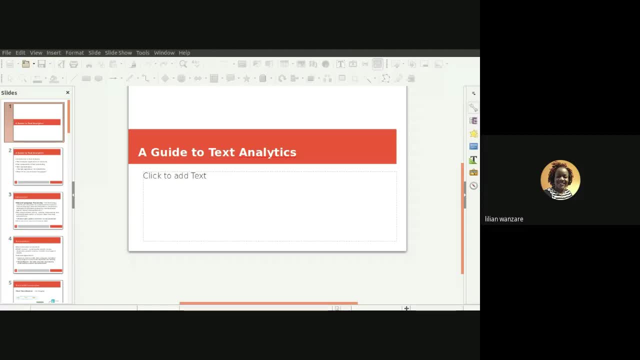 And it assumes some background more or less, especially in the tutorial session or in the practical session, some knowledge of programming or Python. I try to give simple examples and more complex examples to kind of balance between the different groups. I'm not sure of everyone's background, but at any point, if you have a question, 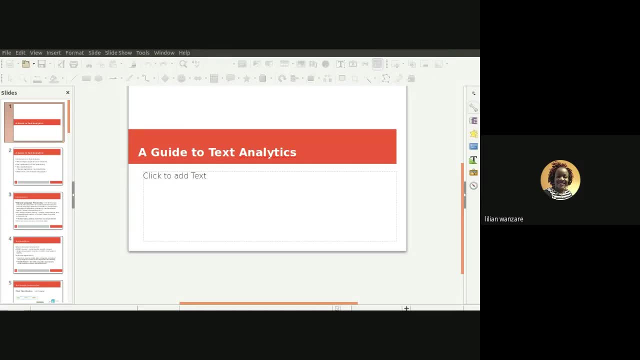 you can just send a chat and then I'll see how I can assist you. okay, So we can just start A guide to text analytics, just as Peris has said, we'll look at some introduction, more or less trying to understand what is text analytics. 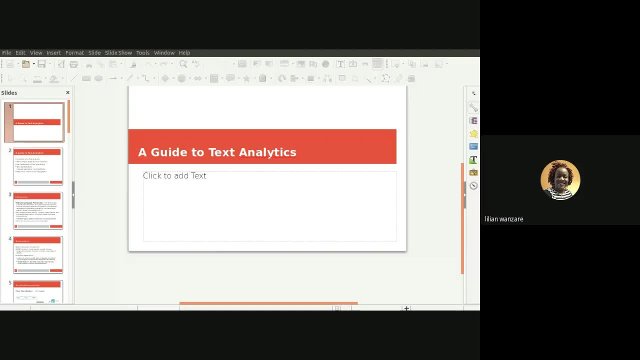 and then I'll go into deeper examples of some techniques that are used in text processing as our applications in business, and I'll give some practical, practical examples that you can try out later on. They'll be all based in Python, Okay. 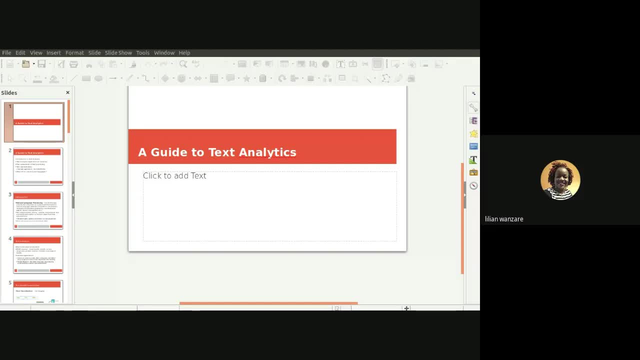 To start, I'd like to take a step back and kind of first of all explain what we mean by natural language processing, because that is really the overarching theme I want to talk about today. The natural language processing is about how do we build? 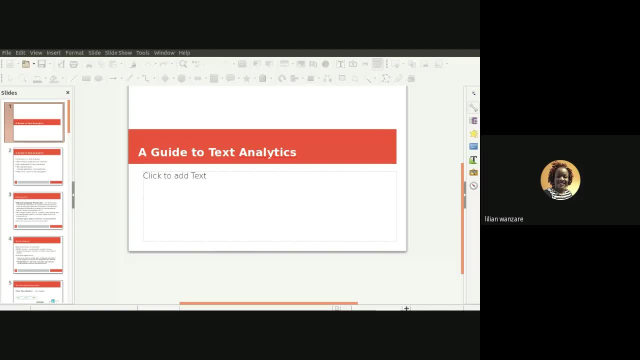 intelligent machines or computers that are able to understand human language. The motivation behind this is: as humans, we communicate dominantly by speaking to one another. yeah, It would be nice to be able to, you know, speak to our machines, speak to your phone, your laptop, your whatever other. 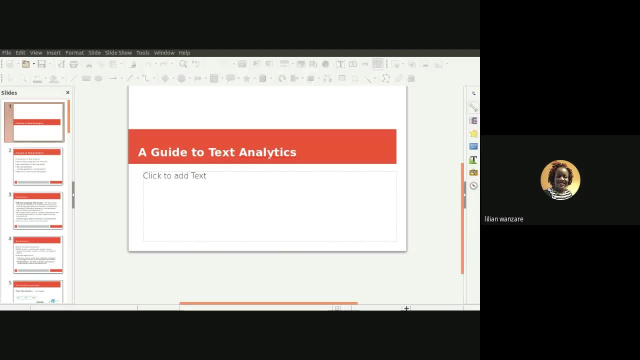 machine that you may have, okay. So think about things like you know, machine translation techniques. think about how you ask Google for something, whether it's information retrieval and question answering. Think about chatbots. you know those are compositional agents. 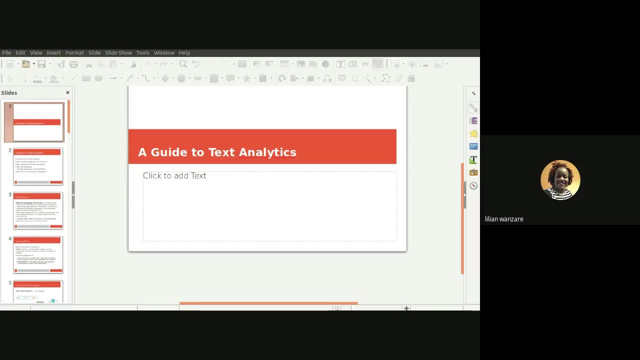 Think about things like converting, you know, speech to text and text to speech. That is kind of speech recognition. That is really the overarching idea of natural language processing. But if you nail down to text analytics it takes a more. I would say. 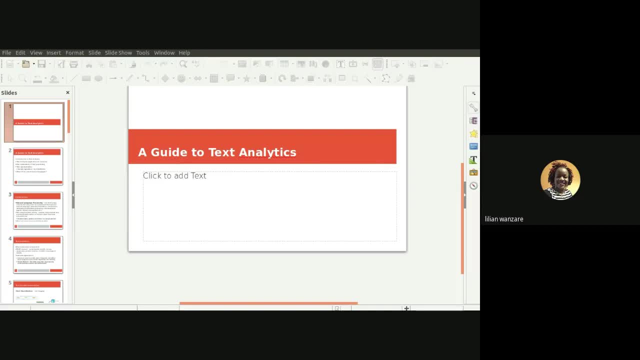 business-oriented kind of side, like more application-oriented. okay, Then really, just how do you make you know unstructured text more useful? How do you reveal patterns from text? How do you reveal insights from from text? you know What can we learn from existing text? okay, 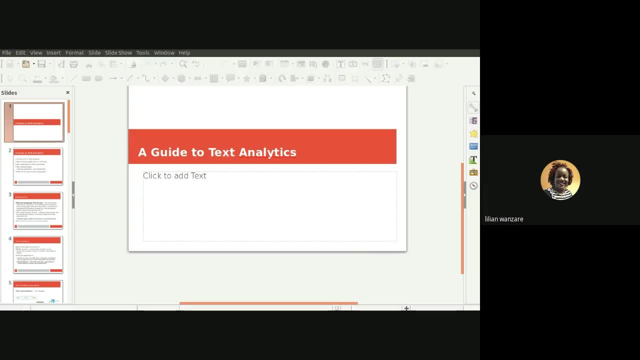 And, as you all know, there are, like, numerous sources of textual data. If it was a classroom, I would ask to name a few. okay, Like, what are some of the sources of data that you know? you know, People write on social media, you know. 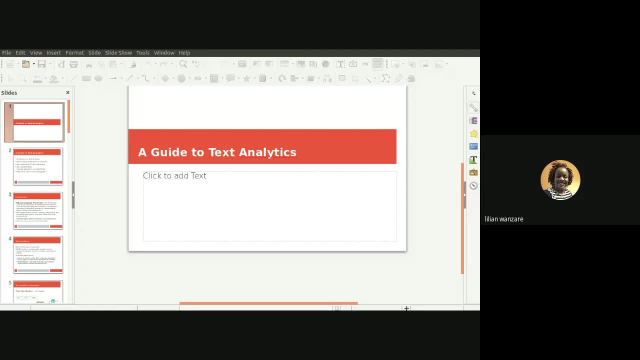 you send SMS, you chat on WhatsApp, you chat on, you send emails, you know you send complaints and reviews to companies. yeah, So all these are sources of textual data, And the main question that business people ask themselves is: what is this value of raw data? 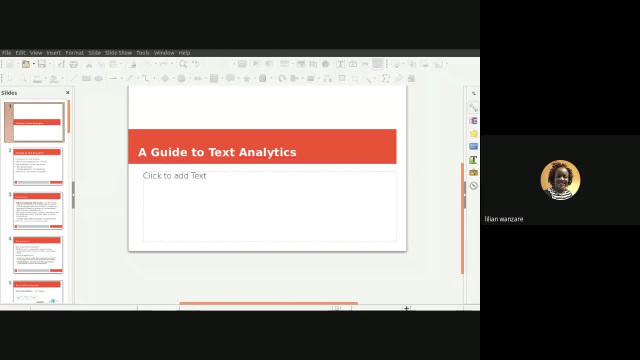 Okay, When they received a million. when Safaricom, for instance, receives you know a million texts, how do they go about going through them? you know, Hiring someone to read them doesn't really make sense. yeah, If you are kind of. 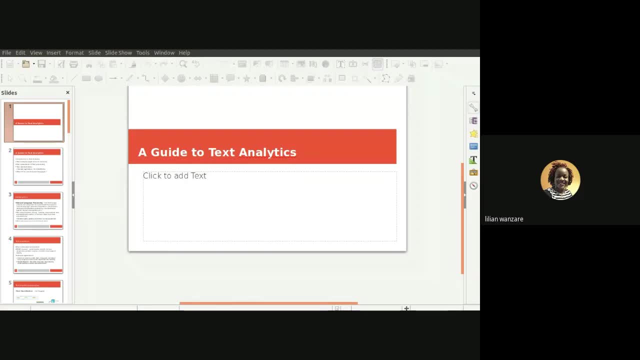 somebody selling your product online? yeah, And people send you chats. how do you siphon through all these millions of chats and get to understand what are they talking about? What are their issues, What are their complaints? you know What is it that they're talking about. For example, think about this: 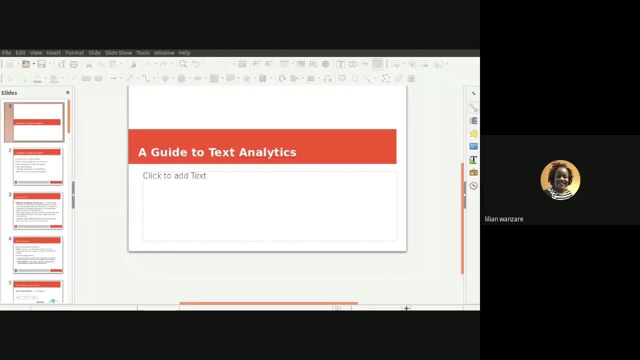 ticketing system for emails. yeah, How can you automatically categorize that this email or this issue is about, for instance, for Safaricom? my phone is not. my network is unstable. It's unstable at some particular place. How can we channel that ticket to the right water department? 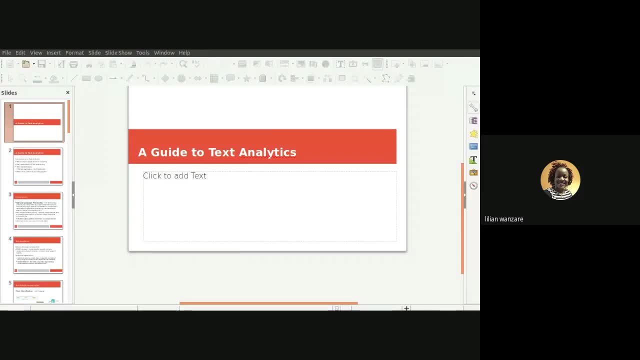 Another email could be. you know, my M-Pesa has, I don't know, blocked. How can I channel it to the next water correct department, Because they have millions of subscribers, Therefore they expect millions of water issues. How can they automatically channel this? 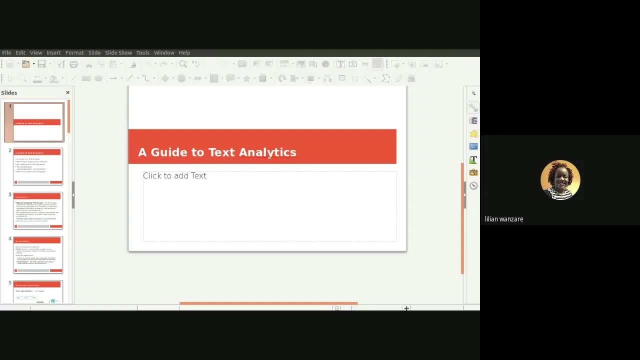 information to the right water department, For an example, if you're doing market research for your product. you're selling products online and people give reviews. you want to understand what are their sentiments. Do they like your products or do they hate your products, For instance? yeah, So really there's a lot of. 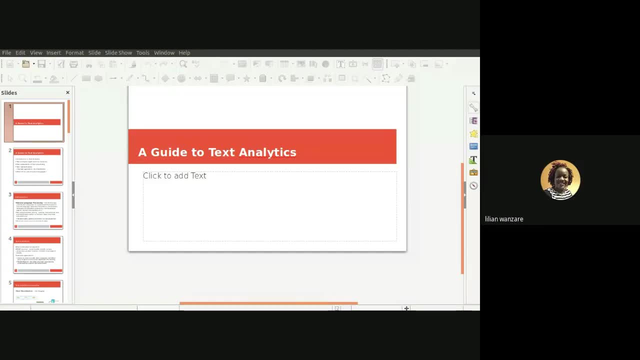 information that can be gathered around texts that can help us to really make more informed- I could say, business decisions. That is really the background of where tech analytics comes from. How can we be able to get really insights to make us help us make more informed decisions when it comes to? 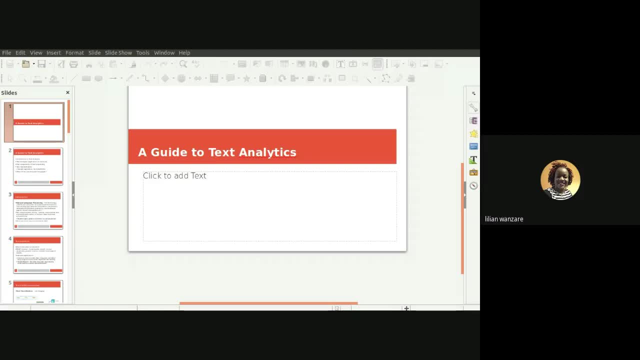 our business, okay, Okay. so I'll just quickly move to some examples. So I kind of focused more around classification of text. So really, what this means is, for example, what I was talking about here. if we try to understand what is. 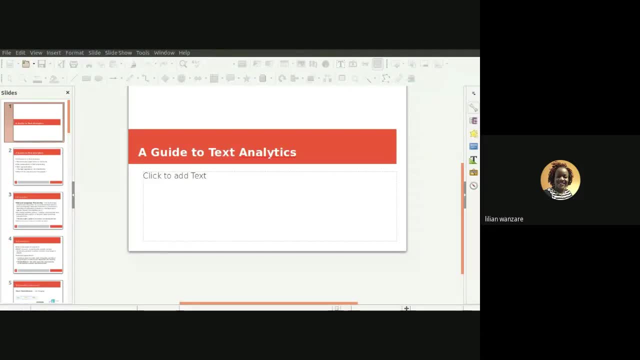 my customers opinion or sentiments. okay, My experience so far is fantastic. That is good. So, really, that issue is labeled as what it's: a positive review or is it a neutral review, or is it a negative word review? okay, so it's really taking a particular text, data and 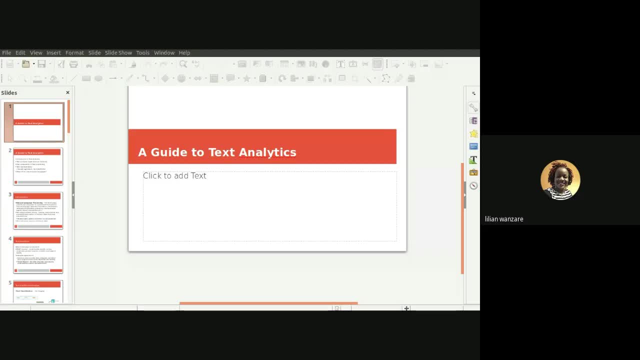 giving it a tag or more than one tags that represent the main issue in that word text that you're trying to classify. think, for example, if you are looking for what a publisher for instance: yeah, you get many articles, but you want to automatically know before, automatically classify those articles and articles. 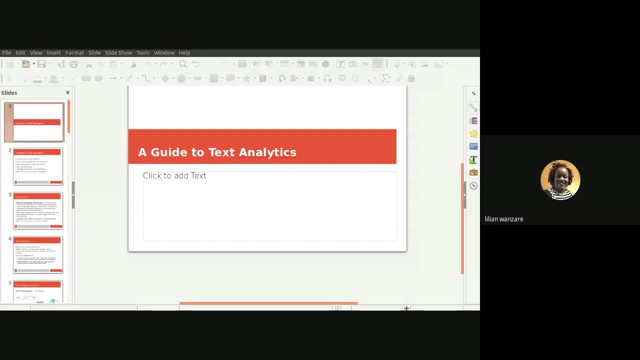 that come into your publishing firm. are they about technology? are they about sports? they have entertainment. that means you're trying to give it a tag automatically. so when somebody sends you an article to your publishing firm, then automatically it's given a tag and that is sent to the right person who can. 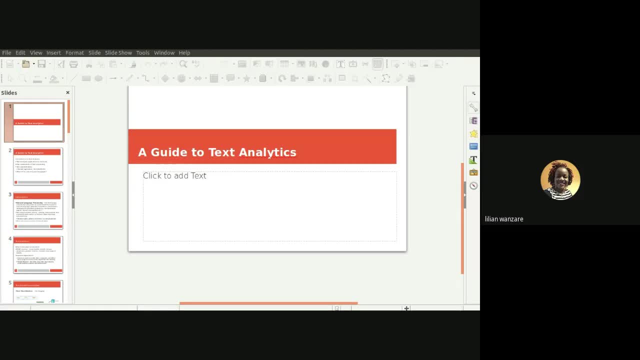 review that. for instance, that piece of what article? yeah, so you are giving a tag to a text. okay, the same way our emails work. when emails come in, they either go to your inbox or go to spam. already, if an email is spam, it's given a tag of spam. that is why it sends to the 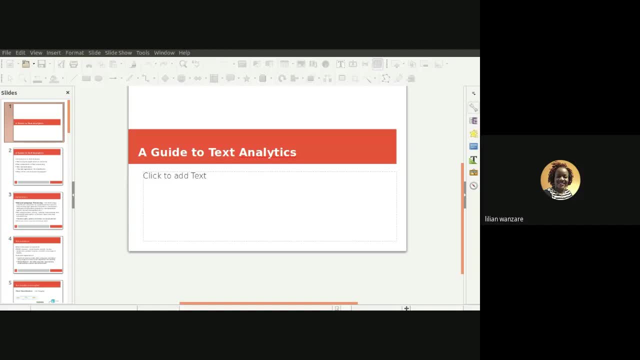 spam folder. it is a good email. it's given a tag of not spam and that is why it is sent to the inbox. so classification is really about tagging texts with the appropriate tag that represents more or less the content or the issue at hand. yeah, so you can see there are various applications to it and a form of. 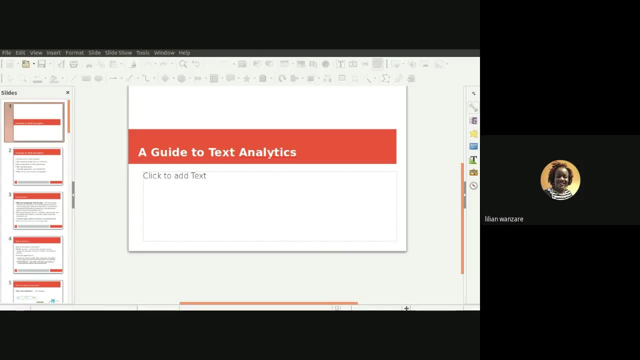 classification is what we normally use in conversational agents. people call them chatbots. yeah, they are able to converse with you, for instance. yeah, in the example I've given, someone is really asking: how much did I spend on uber in September? now the system has to understand the intention. what is the intention of the? 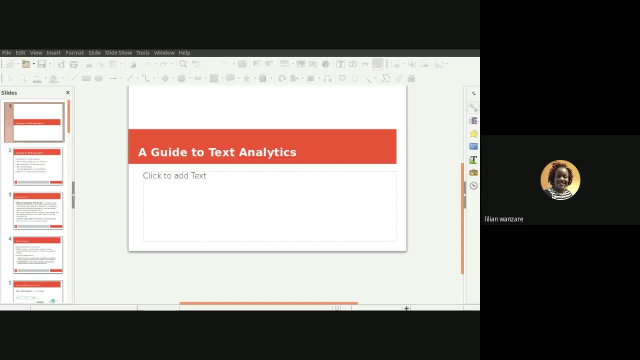 is it that the user is asking that they can provide the right word to answer. this is called intent classification. yeah, or an example can also be if you have a, a chatbot, that tries to answer. you know, frequently answered questions. okay, somebody asks, for example, uh, i don't know which. 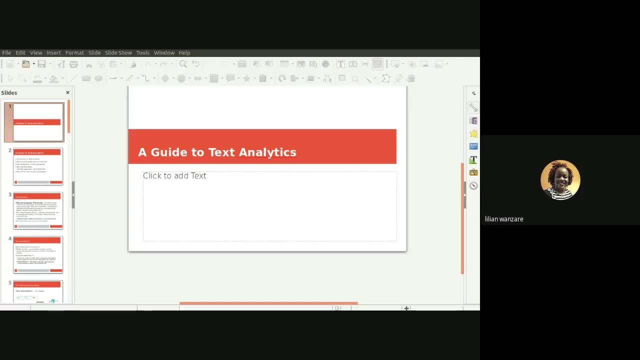 bank upside bank. yeah, somebody asks, okay, how to open an account, then you have to understand the intention of that question such that they bought response with the correct answer after knowing the intention. okay, so automatically discovering the intention behind the text, so a kind of text classification, which is called engine, and it's really, really used a lot right now when you're. 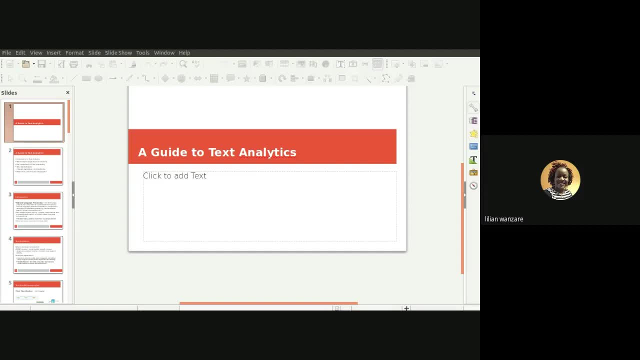 building what are called the conversational agents, or what we call the chatbots. now i like to give some business applications that i'm currently working on. this is just to help you understand, you appreciate text analytics and then in the next, uh, 15 minutes or so, we'll go deeper now into 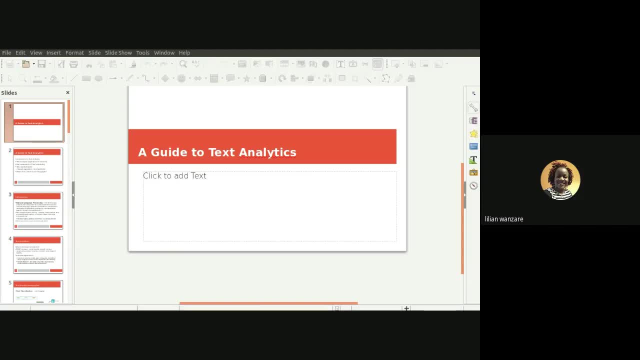 really, how are these? how can these be? what achieved? okay, so right now, let's really just try to understand in general what exactly it is. so i'm working on a, a project right now that employs text analytics, so what they want to do is be able to extract informative 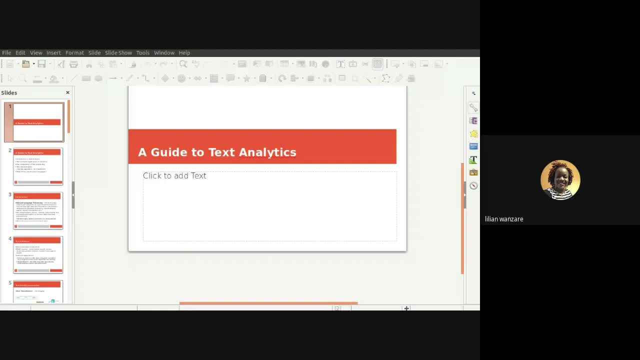 information from, for example, m-pesa or bank statements. yeah, for them to make meaningful decisions. so imagine that you have such a bank statement. okay, on the red circle part is the descriptions of whatever transactions that you do, on the right side, as they either the amount of money you spend on withdrawing or on deposits. okay, it is not enough to just 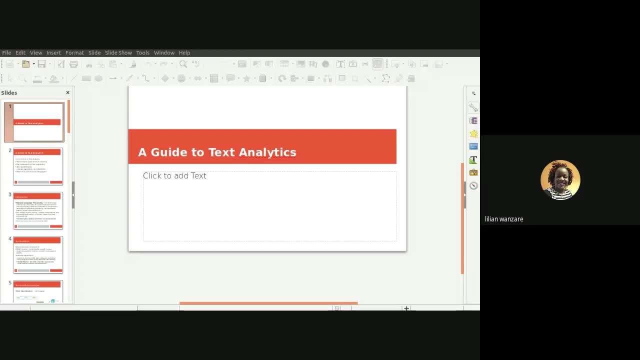 know how much you spent on withdrawals and how much you spent on water deposits. it's very important to know what were you using that withdrawal for and what are you using that. where was the deposit coming from? okay, so, for instance, i find that most of these banks, insurance companies. they provide some kind of loans or insurance. yeah, 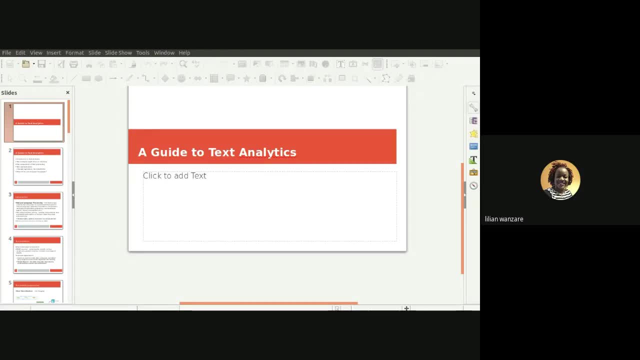 they want to be able to segment users into risk levels. okay, these are more risky users. these are, you know, not so risky users and they use this information. if somebody is, you can see from their transactions. yeah, for instance, this person um kind of purchases from the supermarket a lot and they have a kind, they are a kind of income in awards apparel and they just 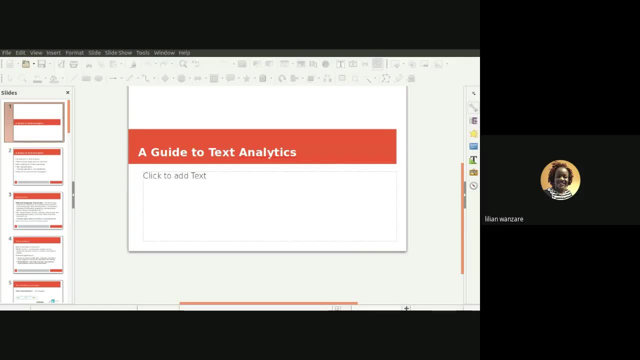 spend on supermarkets. why do you categorize them? if somebody else gets police, for instance, and immediately bets with it, what is the risk level of that person? if somebody gets their money and pays mortgages, what is the risk level of that kind of words people is if? if somebody? 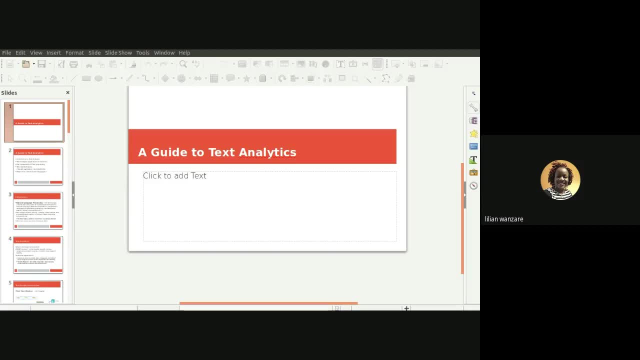 borrows from one bank to pay a loan from another bank. okay, so maybe you borrow from ambassador to pay a loan in case you be, for instance- what is the kind of risk level- this kind of people. so the project aims to extract information from the description part of banks. 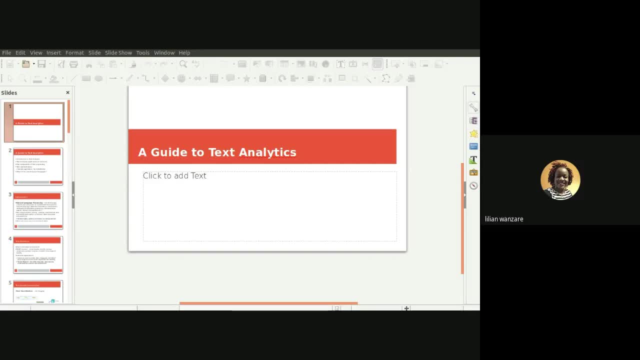 and the ambassador statements, to be able to group people into risk level words classes, and we employ a lot of these text processing techniques that i'm going to give you more information about. yeah, so right now, uh, the value of data is high, and not just numerical data, especially the value of 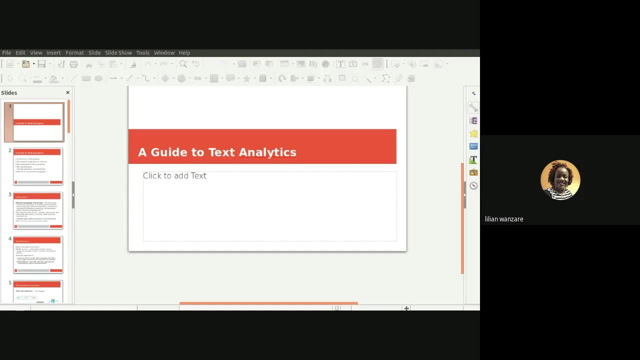 textual data. yeah, and there is more and more and more companies and businesses are looking at how i'm able to make use of our text tool data and not just a, like you know the ordinary, you know a numerical that other people are used to uh processing, okay, so kind of that is an example of 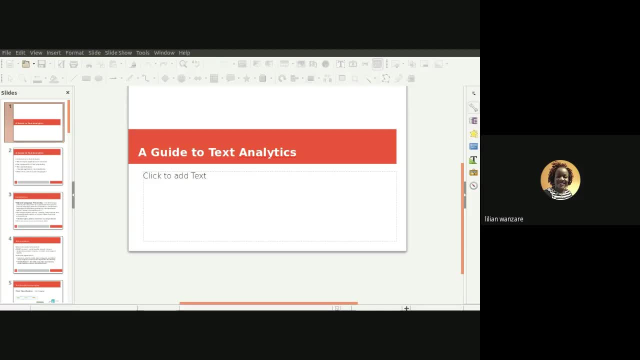 something that i'm working on now. a second example that i'm working on right now is the issue of extracting. you know, customer understanding, customer emails, okay, but what this client wants exactly is, if they get an issue like, for instance, i paid for a subscription but i still have ads and a free version, they want you to split. 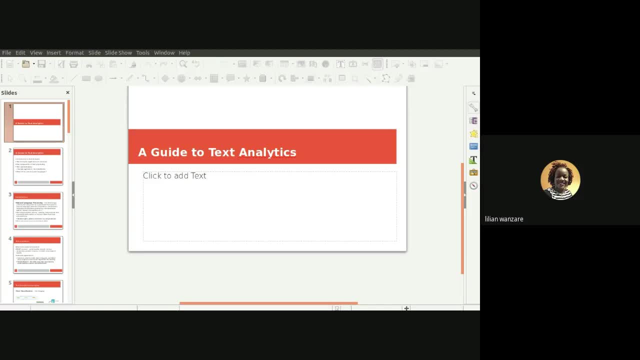 that sentence into various- i'll call them phrases or classes. that represents many, the various things that are being addressed in that statement. or it can be a very complex and long sentence. so, for instance, they want: for every email that comes in you simplify to the base issues. 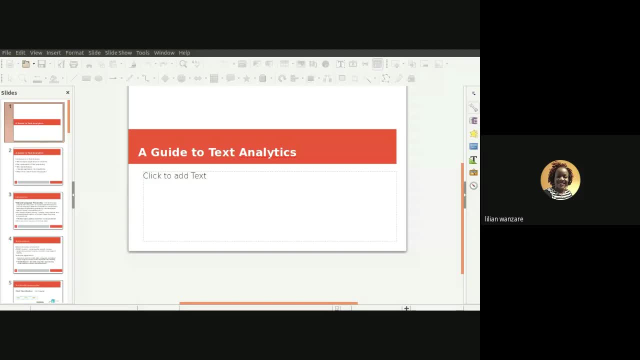 i have paid for a subscription, i have ads, i have a free account, okay, so really, that that they're able to find the simplest of issues that a user is trying to to raise, and each of these issues is being tagged: okay, it's an issue about subscription. 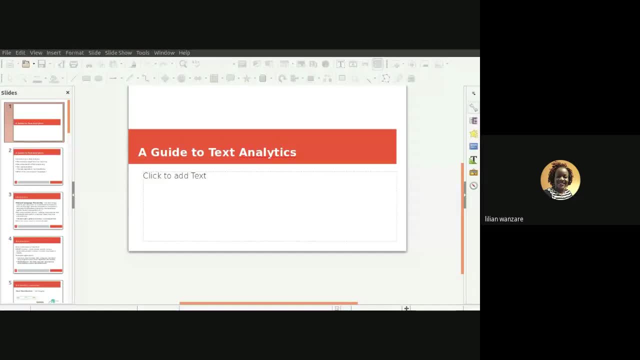 issue about ads, issue about free account, you know. so they really want to understand the smallest issue that the customer is is: uh, is raising yeah, and really these are the kind of challenges, because you can imagine there'll be spelling errors. you know people will be using wrong. 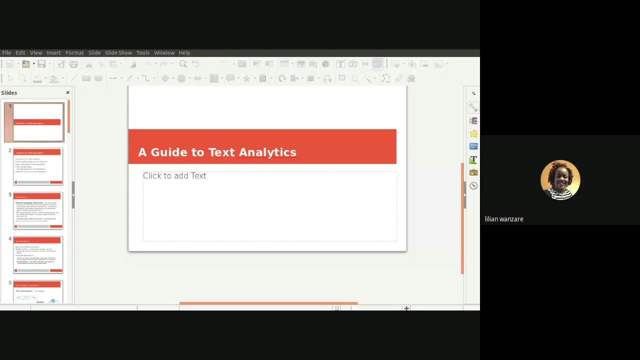 punctuations and people are not native english speakers. they've been speaking, you know translated english. okay, now how are you able to process all this kind of text to be able to understand what the customer is talking about out? so i hope i have enticed you enough to kind of appreciate what is it exactly when you talk? 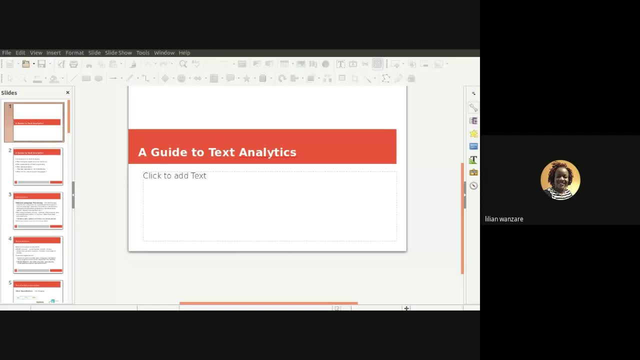 about text analytics and what kind of applications people do when it comes to text analytics. okay, after that, if anyone has a comment or question before we look at really the kind of techniques that are being used to achieve that kind of applications, okay, if there's anything you can. 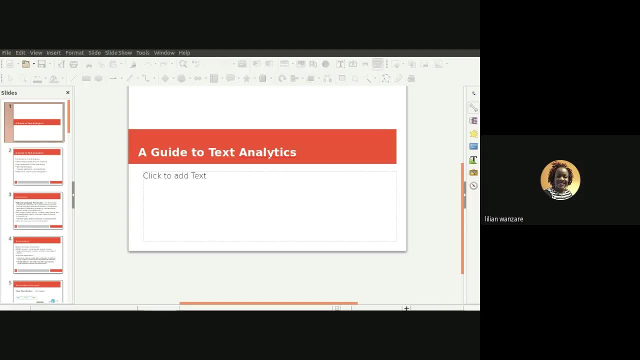 just send uh chat. i wanted to be very interactive, be able to see if we are together or not. okay, so if there's none, i'll just start on some examples of components or techniques that are used to achieve text analytics. the basic thing that you have to do first is to split your sentences. okay, if you have a long document, you. 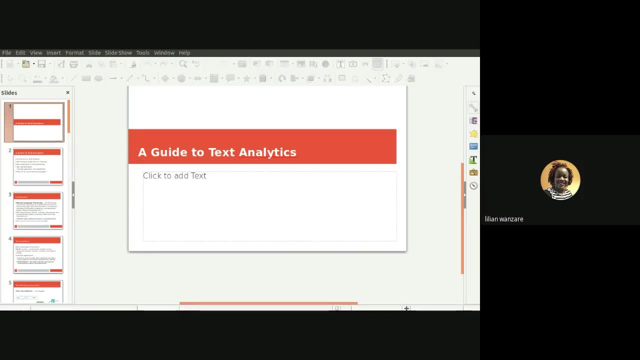 want to understand what is, what are my boundaries of each sentence, because most of this application makes use of sentence level analysis. yeah, so the first thing is how do we split our document into sentences, taking care of punctuations, taking care of abbreviation, taking care of, you know, long? 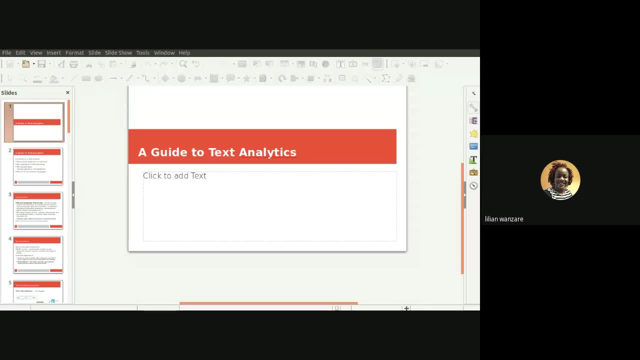 nested sentences, for instance, if it is a conversation. okay, how are you able to split that into the respective sentences? so i will show you in the few minutes on how you do that programmatically. okay, so the first thing people normally do is just, you know, split sentences. so 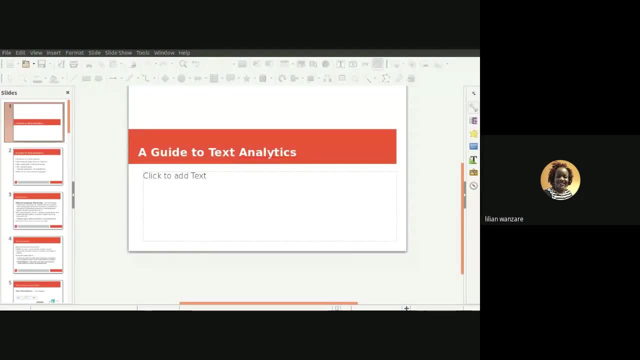 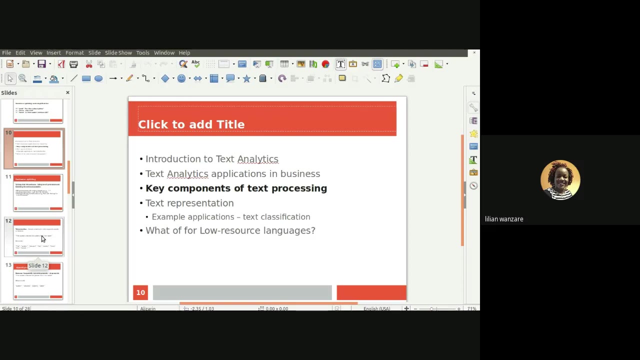 now you have from your document, you have sentences. okay, the next thing i want to do is what we call tokenization. you want to break this sentence into separate individual words, so let me start from here. okay, i hope, when it comes to the business application, more or less we 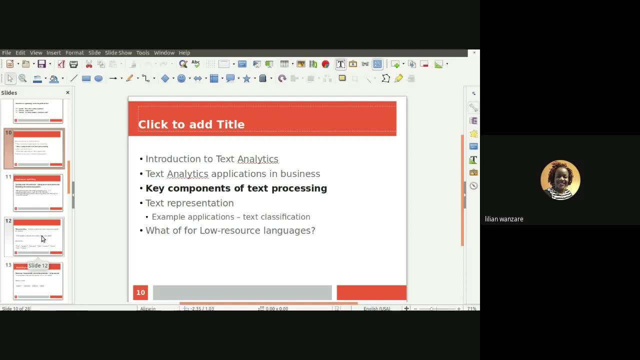 have understood the kind of- uh, its application more or less than the general application, kind of it's application in business. okay, so i was talking about thank you. you're talking about the various components of text processing. yeah, and the first thing i said was about sentence splitting. yeah, 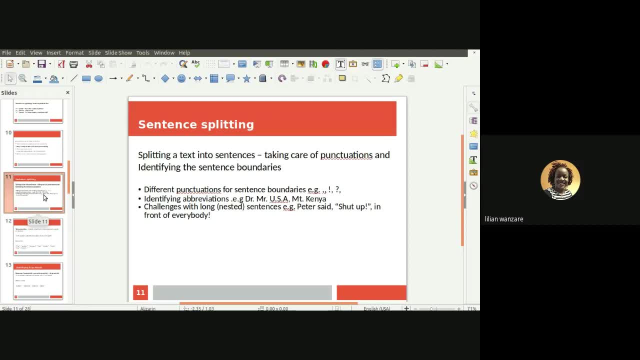 okay, trying to split your document into respective sentences. okay, you can give fluctuations and all the other stuff. after you have your sentence and split, you have to do what is called organization. you are now breaking your sentence into individual words or individual words tokens. so the example i have there: the waiter cleared the plates from the 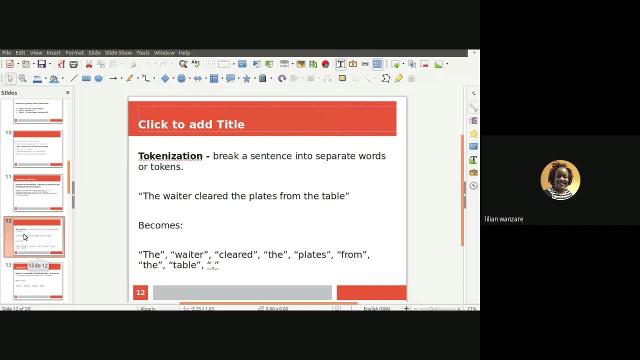 table. now it becomes every single, you know, letter is separate from the other, though is separate. waiter is separate, clear, this is separate. yeah, because they're trying to really piece down to the, to the individual words in your sentence. that is a tool that can be able to- uh, to do. 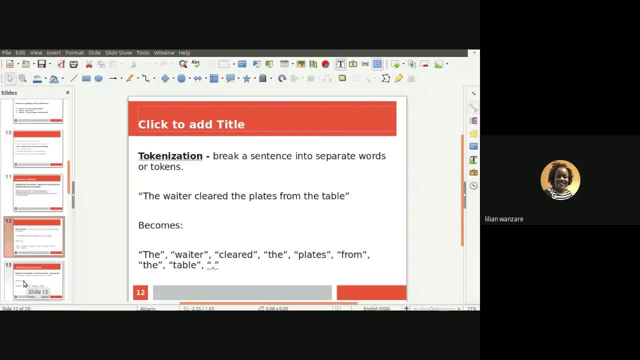 when it comes to text analytics. okay, another thing that you want to do is you want to know, okay, what are the content words of my sentence. yeah, because not only what the sentence contribute to the meaning of the sentence. some are there for syntactic, linguistic reasons. yeah, 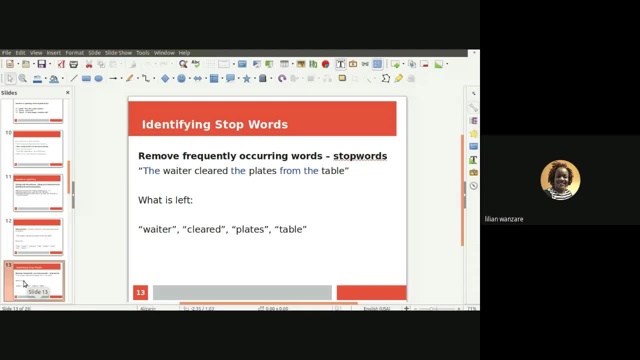 not really for content. so, for instance, if you remove those words that always occur in almost all sentences, they are called stop words. so when you remove them from this, from a sentence, you only remain with the core content ones. so in our case, the blue ones are there: stop. 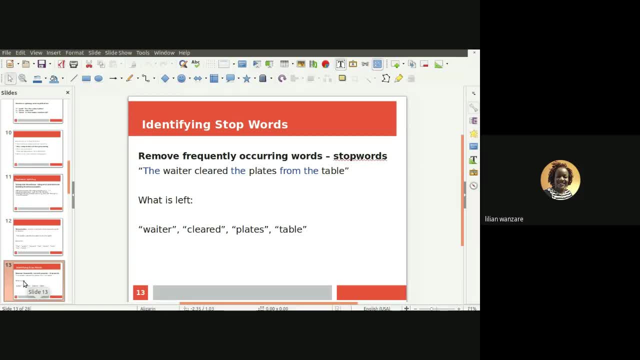 words. so you're only left with waiter cleared plates table. look at the content words of your sentence. what you have done? you have removed the stop words, where the stop words are what you call the frequently occurring um words. okay, that occur in almost every sentence. they don't. 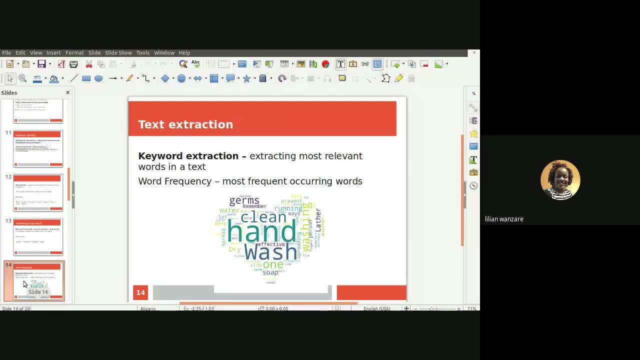 contribute to the meaning of the sentence. now what this enables us to do. for instance, if now you want to look at what are the keywords of your text, you just take the most frequent, the most frequent words after removing the stop words, so that becomes your the relevant words. or 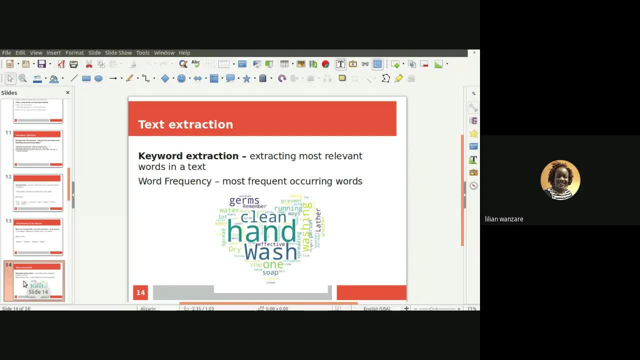 the keywords of your text. okay, so now other people build what is called the word word clouds. okay, they just strip down their text, remove the stop words and then they count how many times the different words occur. okay, and then you're. what you left with is what are the most frequent words? those 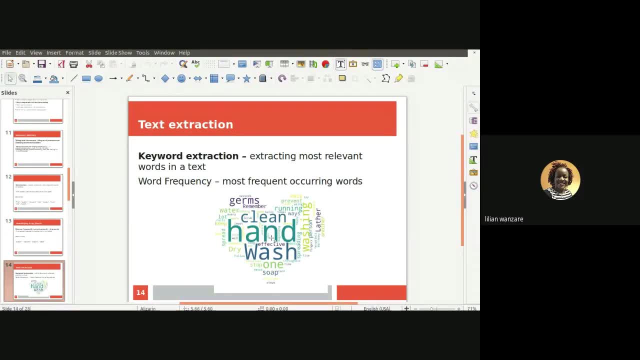 form part of your the keywords of a particular word document, so we'll leave that for now. do a simple example how to be able to to do this um programmatically. okay, now, if you notice already, um, you find that uh words are always inflected. okay, inflection means um, like a word has suffixes. 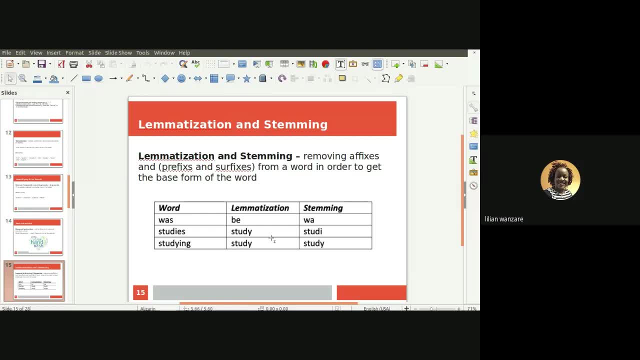 and affixes. yeah, what you want to do is, if you really want to know what are the words, then it is better to reduce those words to their base. okay, so that you, instead of counting, for instance, studies, studying differently, you want to count them as one word. 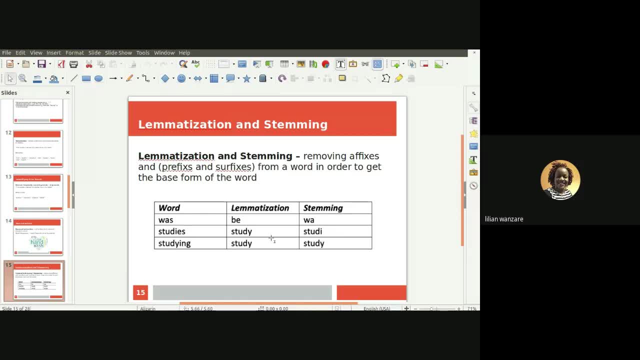 so you can use what is called lemmatization or stemming. they are related but not, uh, exactly identical. okay, that helps you to reduce a word from its inflected form to its base form right now. if you do that, you're able to actually now get the actual count of the words. 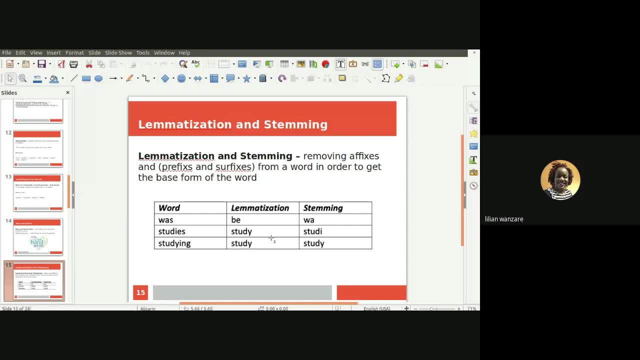 that exist in your document, the unique words- after you get rid of them so you can use your inflections. okay, you do that by doing what is called the materialization. so by now you're broken down, our document. it's no longer just a document. it was. 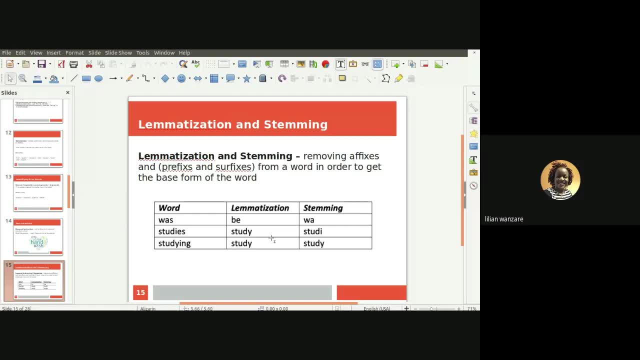 left from document to sentences, to tokens. now to lemmatized words, like now they need to the actual words that are talked about. so, for instance, was is the word? if you limit it, it becomes p. if you stem it, it becomes what? stemming is always an approximation study for difficult. 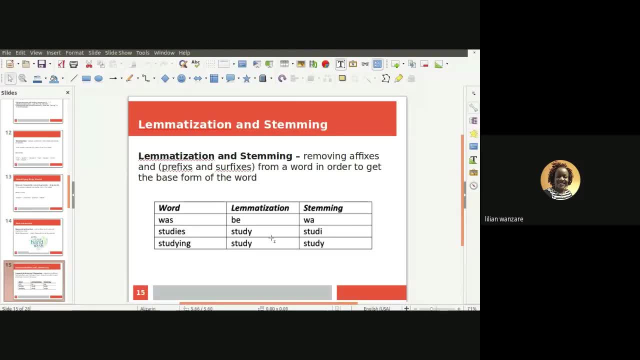 but it always just strips out the last words in a word. so always i always prefer using uh, lemmatization. okay, so studies become study and studying become also study the base. what? okay, that enables us to be able to really understand the words in your document. 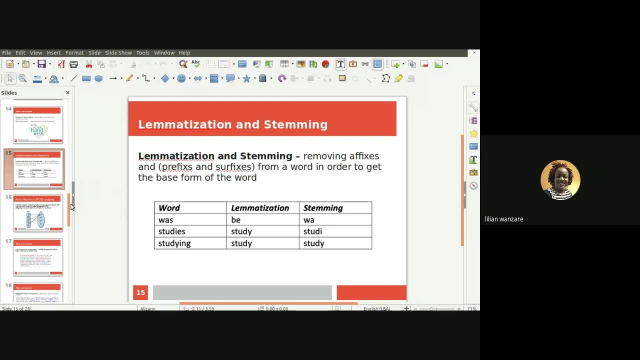 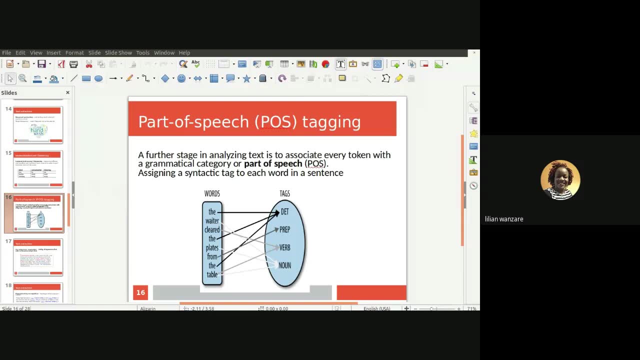 now we have our best words. yeah, what else you might be interested in finding out is the parts of speech texts. okay to be able to enable us understand what it is all about. you want to know what are the verbs, what is the determiner, what are the prepositions, what are the nouns? okay, knowing these. 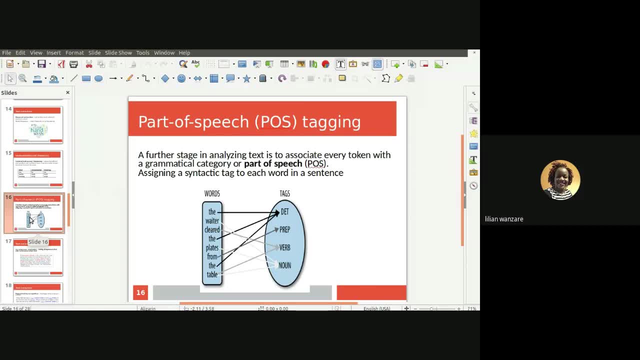 things enable us to do the next things i'm going to tell you about. yeah, so part of speech is really understanding what is the synthetic tag of a given word, like that is from high school english or primary english. yeah, so really have to understand what is the tag. part of speech. 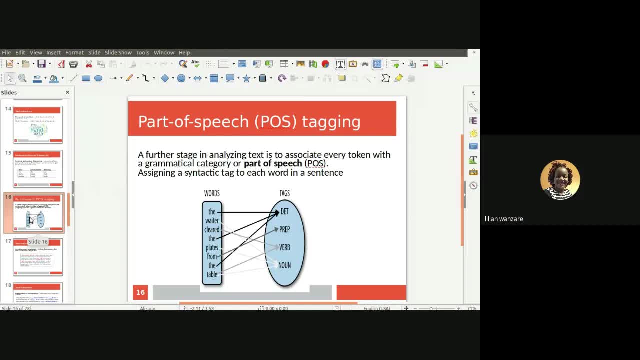 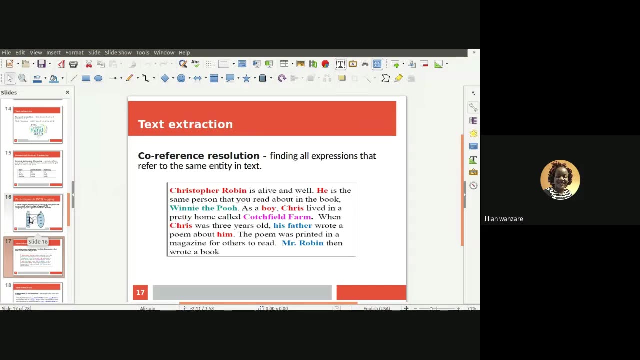 so if now you know what is the part of speech tag, okay. interestingly, if you want to really understand the text, you want to be able to, to get information from the text, okay, now this: there is a technique called the reference resolution, like finding out what an expression refers to in text. so if you have that a text, christopher robin is alive and 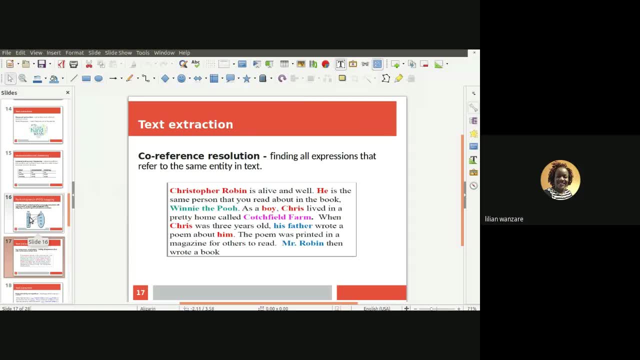 well, he is the same person that you read about in the book blah, blah, blah. you want to know, key the first to christopher robin, okay. and then you want to know that a boy, chris, lived in a pretty home. so you want to know this: a boy is chris, it is the he and is the christopher water robin. so you're. 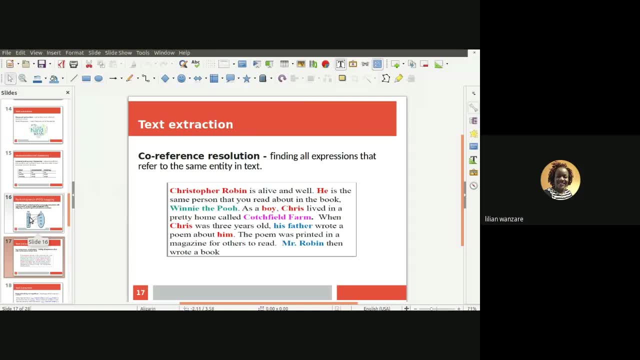 trying to really um connect the different entities to their to the same. the different what the same water person. we're able to know this because you know that, for instance, a boy will have a tag and okay, he is a pronoun. i know that nouns and promise can refer to some proper words. 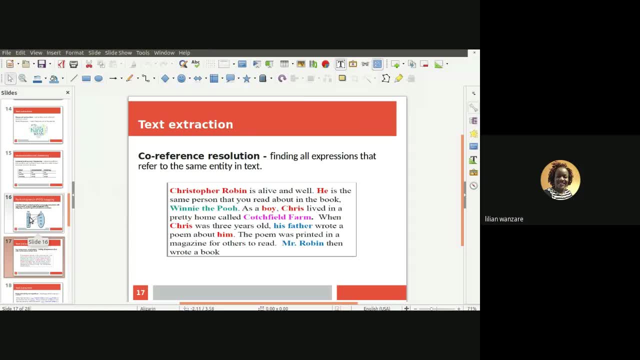 noun, for instance, if you know the different tags. so all this enables us to extract information. so here, if you want to, if somebody asks you, for instance, um, what, um, where did robin live? you can. where did christopher robin live? you can know he lived in a catch field. 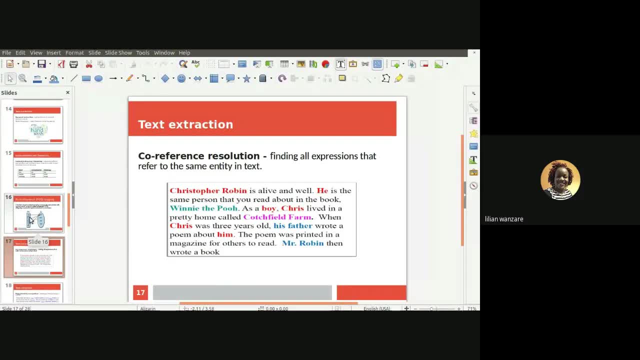 farm because you are able to to put together that, this crease and the name of this little girl we call the chris mcgraw. you can say: this is chris the boy and he is christopher water. probably it enables you to answer questions from a given text, if you ask how. 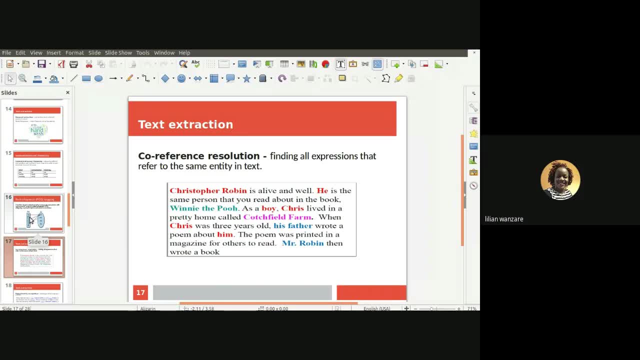 old is the staffer? robin, you can say, is three years old, because you know that this chris is a christopher. what, uh, robin? okay, so really, it enables us to extract information from from text. the other thing it enables us to do is what we call net entity recognition. okay, you're also going. 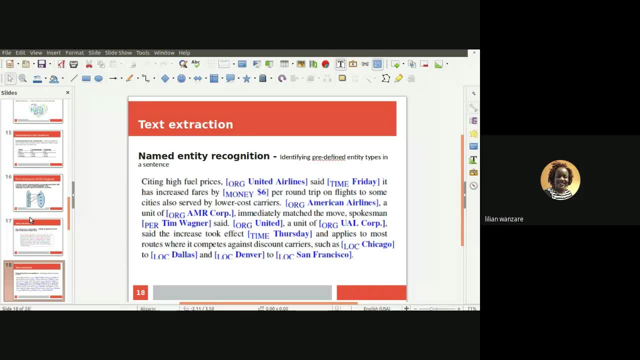 to watch an example of this. so really here, if you want to understand what the asks to do for that, so are the predefined entities in a text, like: who are the people in the text? are there countries in the text? is there time in the text? are there locations in the text? you know, those are what. 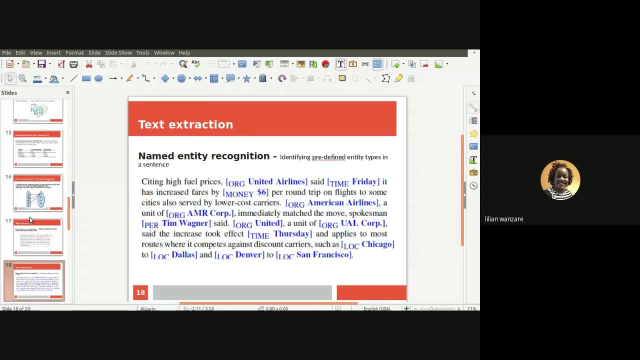 are called predefined entities. it will be more clear once i show you an example how to to program that. okay, that is what we call entity. all this is possible once you're able to tokenize. you do part of speech for reference resolution, then you do entity words resolution on top of it. okay, so 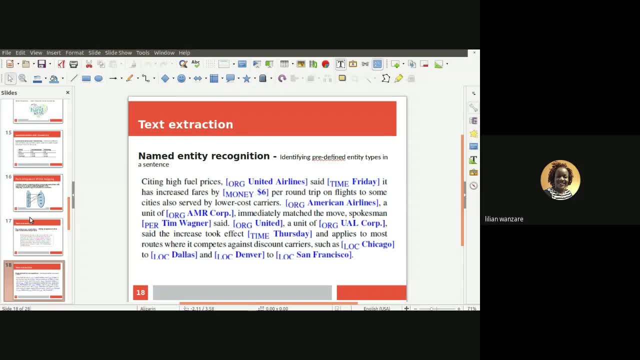 everything kind of builds up to more and more complex words, techniques that are enabled to extract information from text. for example, we have here is um. united airlines is an organization. you know friday is time, six dollars is money. you know, for instance, this: uh, team wagner is. 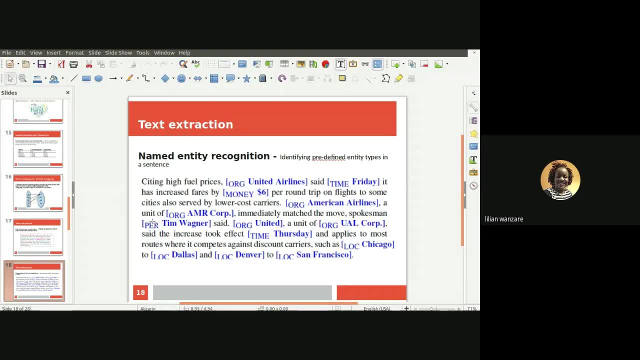 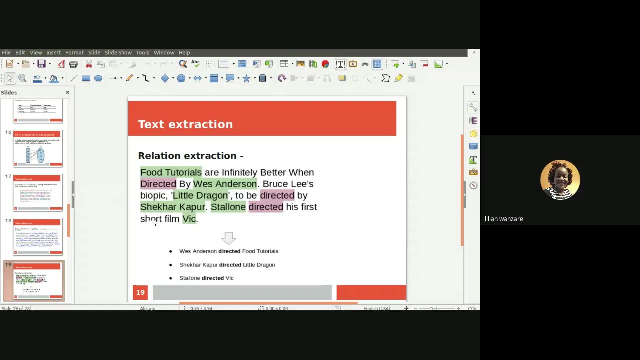 a person, so net entity, really tries to look at all the proper nouns in the text and give them a tag. okay, this is really important for what is called, uh, information or relation, what extraction? okay, so i'm building upon all these concepts. once you do a reference, then you do the. 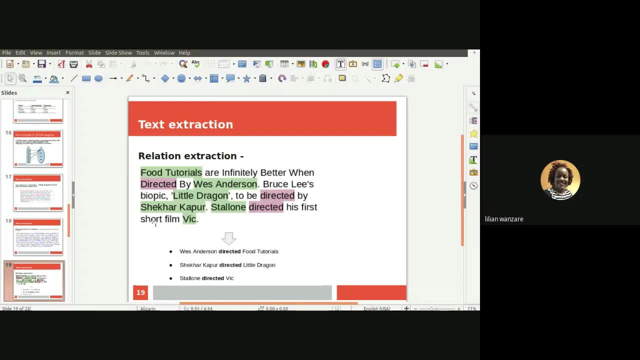 entity recognition. now you're able to extract information from the water text. so, for instance, you know that maybe this food tutorials is a kind of entity, okay, and the west anderson is a kind of. it's a person, then directed is a verb. then you can extract information from the text and saying that: 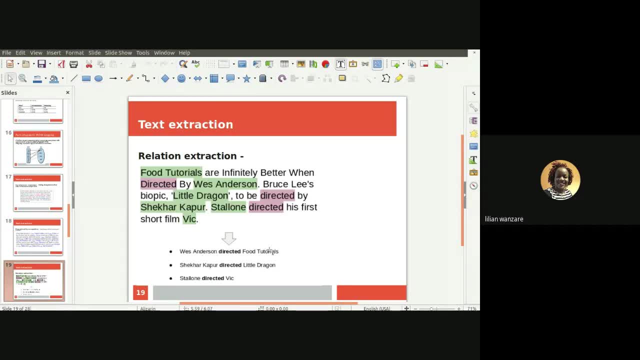 west anderson directed food tutorials. all this is possible because at the beginning you split the sentence. you tokenize part of speech tagging. you need some for reference resolution? okay, then you're able to. you did some kind of entity resolution. now you're able to extract it from the what text like, only the necessary information that you really look for. 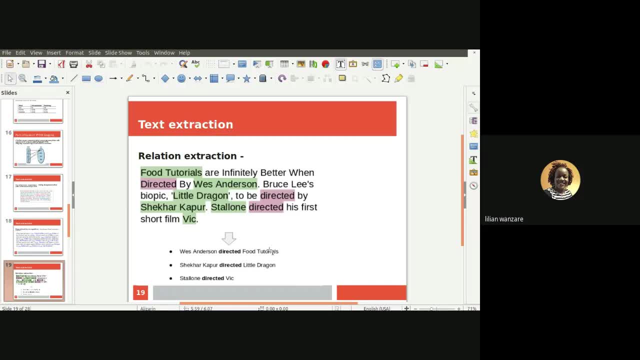 okay. so everything kind of builds up into the final tasks that now you want to extract information from, from uh, from text, okay. so i hope more or less, um kind of gives you an idea of, uh, the techniques that you want to use. i'm going to repeat all of them throughout now, practically so i can be able. 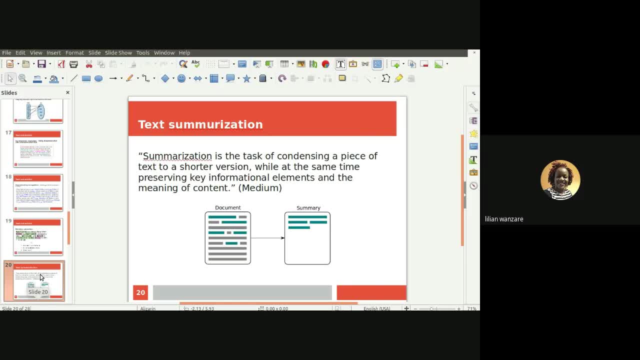 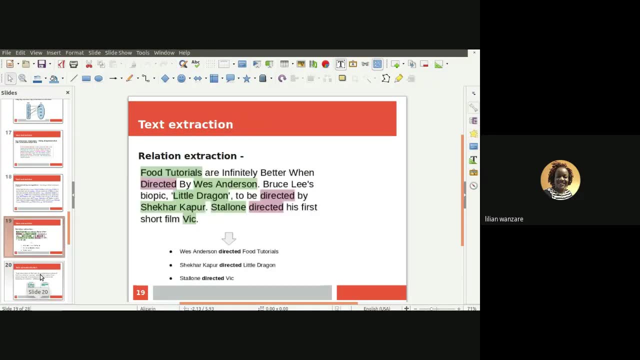 to understand. okay. the last bit is all this enables you to summarize awards a document. so you can imagine if you extract entities on all the text. whatever comes out is like kind of a shortened version of the text with only the key things from the water text. you have to. you have come from a 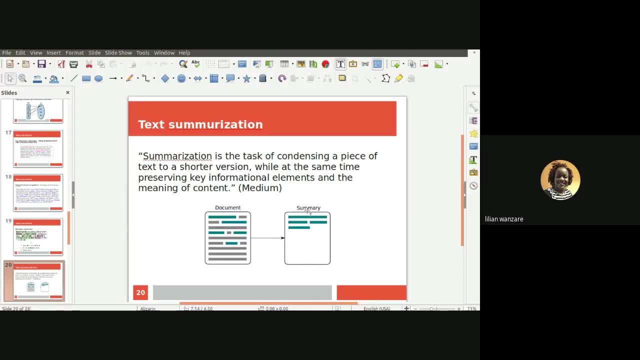 whole document to a small version of the water document, so condensing a text was shorter, uh, fashion, okay. and all this is possible because from the beginning you're able to do the whole pipeline- we call it a pipeline, the whole natural language processing water pipeline- from sentence splitting: 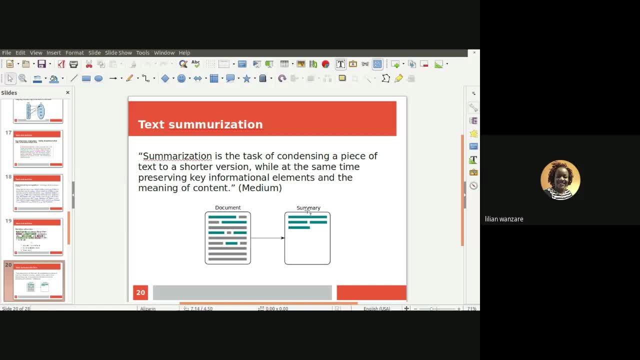 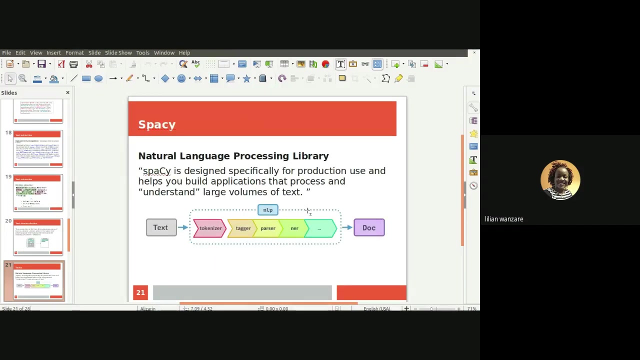 to tokenizing, to battle speech, tagging, you know to, for reference, resolution, to name entities. all that enables you to do what? summarization? okay, be able to get a summary of your, of your text. so, without much ado, we can just start with the what you wanted to do, practically okay, so i'm going to introduce you to. 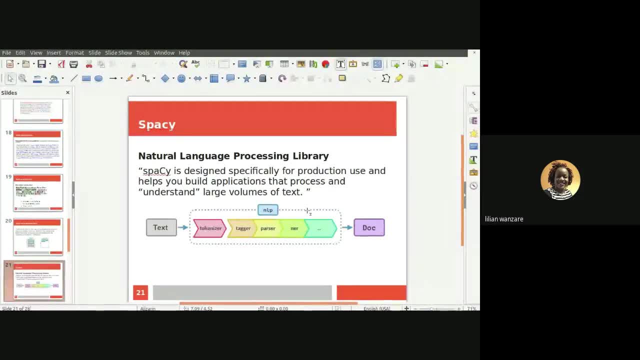 a toolkit, an open source library called sparse. so sparse is really designed for, you know, optimized for production use, like you know, like real life applications. yeah, so what the beauty of sparse is? it does all the things you're talking about. you give it a text, okay, you pass it through the nlp pipeline. it does everything from sentence. 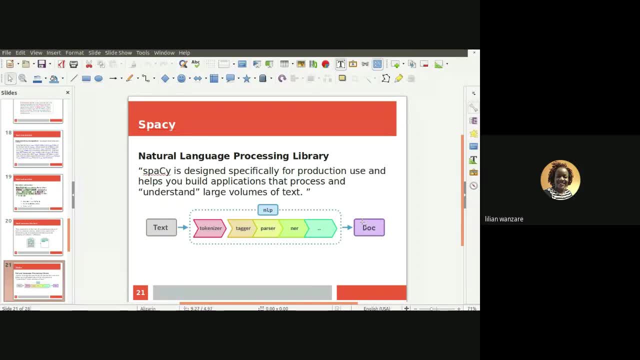 splitting, to tokenizing, to tagging to net entity, completely to your document, and you only extract what you need from that document. okay, so let us really see how that works. so let me see you can tell me if you you're able to. let me share that screen. 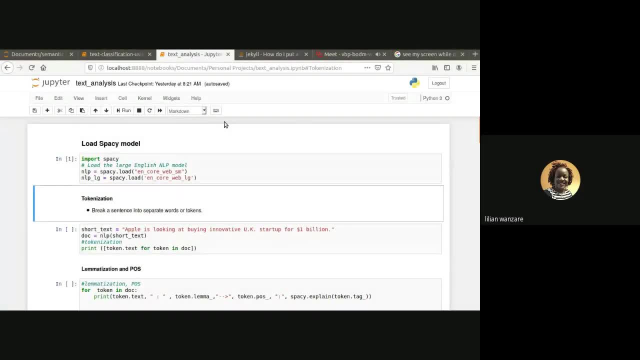 just a minute. we talked about sparse, yeah, so let us just go through all the things we've talked about, okay, so this really assumes you know more or less we have some python background. okay, if something is not clear, you can also just still ask. okay, so the first thing you want to 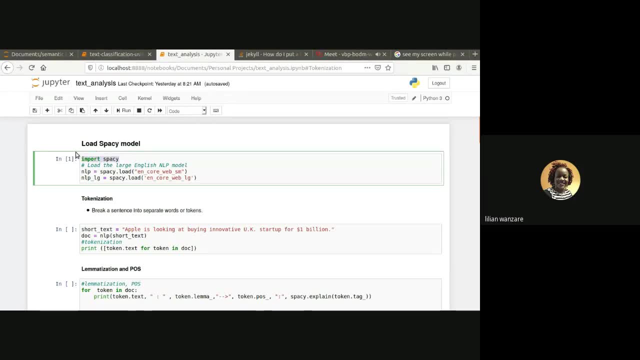 do is to import this passive model. for those who wanted to try it out, um, you have to install a anaconda or python- okay, but anaconda contains all those, uh, scientific packages for text processing and data science in general, okay. and then, on top of that, now, you install what is called sparse, sparse. 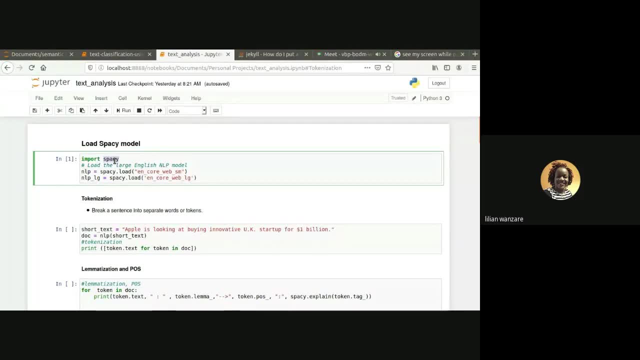 is normally installed using pipe. okay, so you have to do pipe install sparse. yeah, okay, once you import the sparse, you have to import the pre-trained models. okay, of course, all these things to do tokenization, sentence policing- this is a model behind it that was trained to be able to. 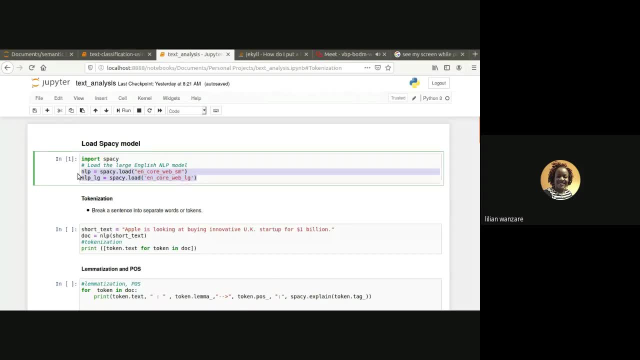 do that okay, especially for english. so for english we have- uh, already you know- modus outside here that able to enable us to do all those text processing techniques. okay, so we just load the models, so you also have to download them, and then you just load them, the way of saying in. 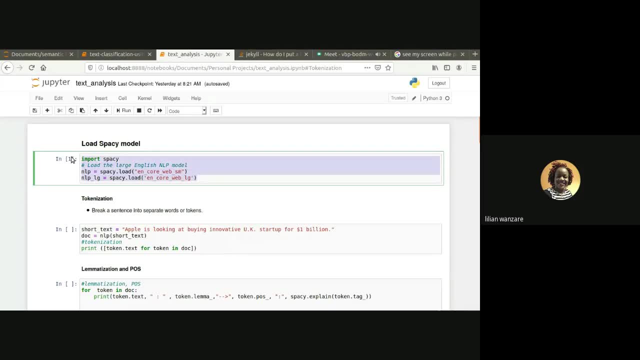 express password load. okay, so once you load them, Now let us start in the next. the first thing: okay, I started with tokenization, really breaking a sentence into separate parts So we can proceed. So, working on the first one, you're working on the text analysis one. okay, 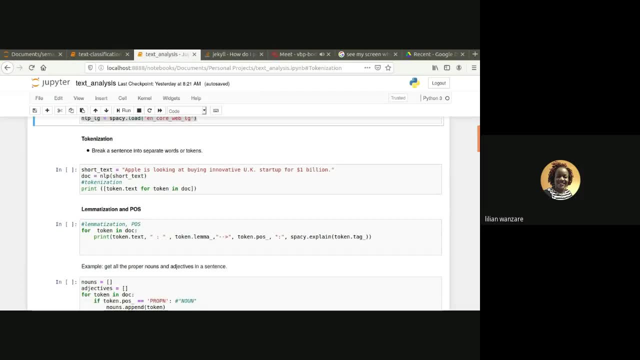 Okay, So you're looking at now the tokenization part, so splitting a sentence into respective tokens, okay. So the beauty of PASI is, once you load the models, you just need to apply NLP on your text. Once you apply NLP on your text, it's able to perform all those analytics techniques I talked about. 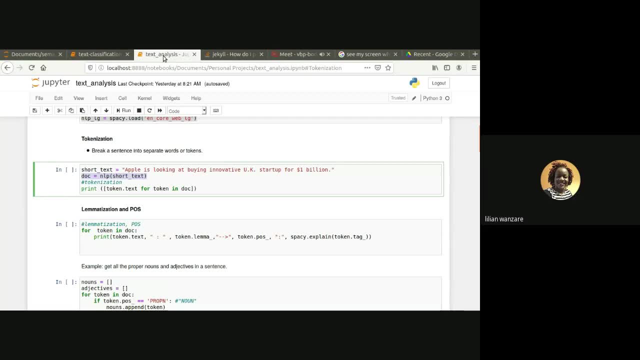 It does tokenization, analyticalization and, you know a part of speech target. It does all that with just one command called NLP on your text, okay, Okay. And then when I run this, for instance, you see that it prints out the individual tokens: okay, including the punctuation, okay. 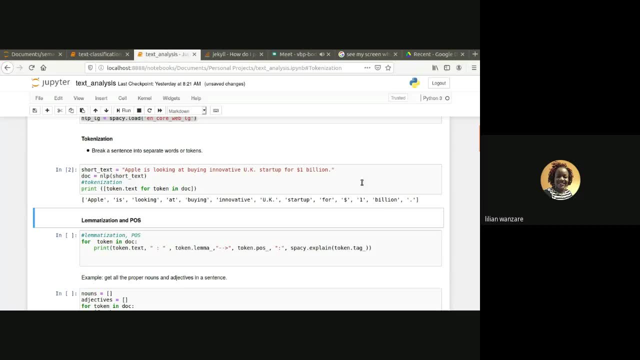 Therefore, it's looking at buying an innovative UK startup for Amiga using just the keyword NLP. So NLP does the whole NLP pipeline okay, It is the pipeline that we talked about when you're looking at the different stages of text processing. 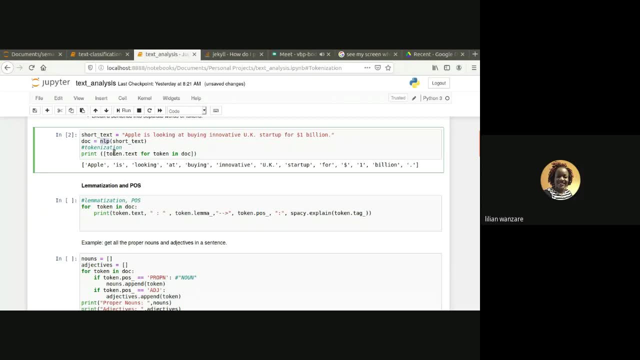 Okay, Again, from just doing NLP on your text, you're able to check out what are the lemmas of my document and extract only the lemmas of your document. So the beauty of PASI: everything is represented as a hash, okay, or a hash mapping okay. 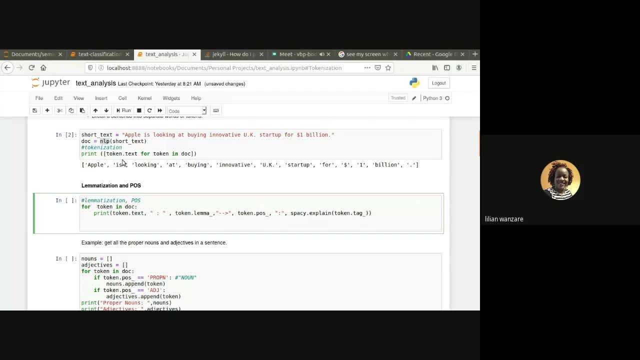 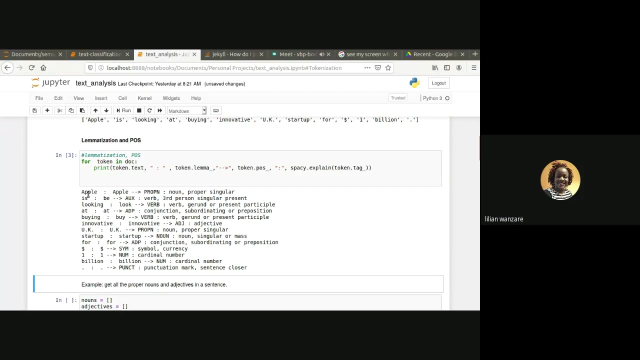 That enables you to access every individual process by just calling the token And if you want the text or the lemma, or the part of speech or the, you just call it. everything is kind of it uses a hashing technique, okay. So if I run this for token in document print- for me the text which is like Apple print, for me the text dot lemma. 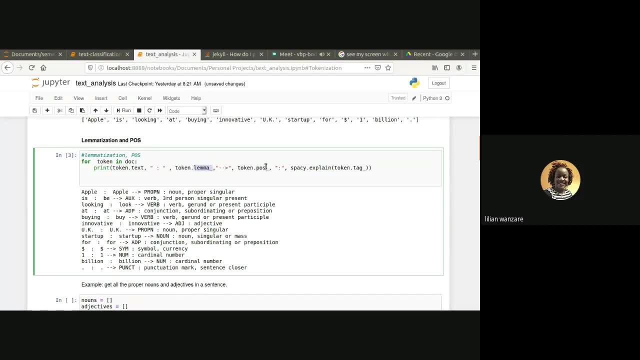 the text, dot the part of speech which is the post, and then explain to me what that tag means, the post tag. Okay, In our case, Apple is looking at buying Innovative UK Apple. the lemma is just Apple and it's a proper noun, because that is Apple, the company okay. 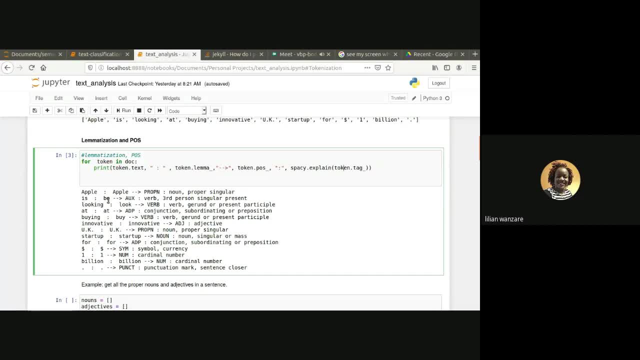 Is is the verb or the word. okay, Its lemma is B. okay, which is just an auxiliary verb. okay. Looking is the text, Look is the lemma. Those are just a word, a verb. okay. So just by doing NLP you're able to get all this. 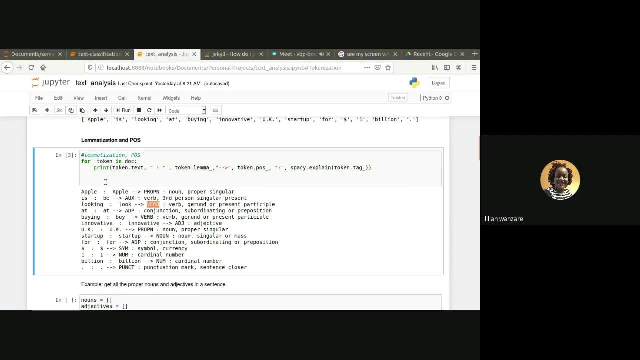 All these steps are formed on your text, okay, So you can see that buying the lemma is buy innovative. the lemma is just innovative because it's an adjective. okay, UK is a proper noun, a proper noun. startup is a noun okay. 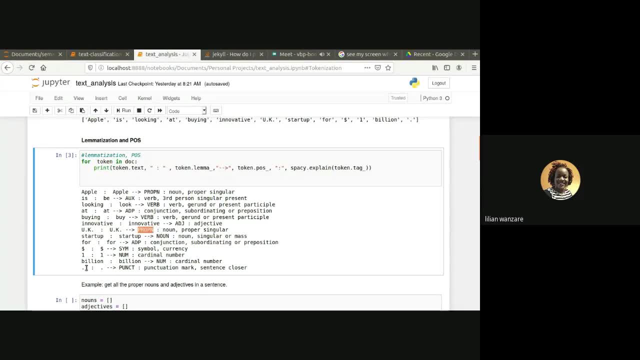 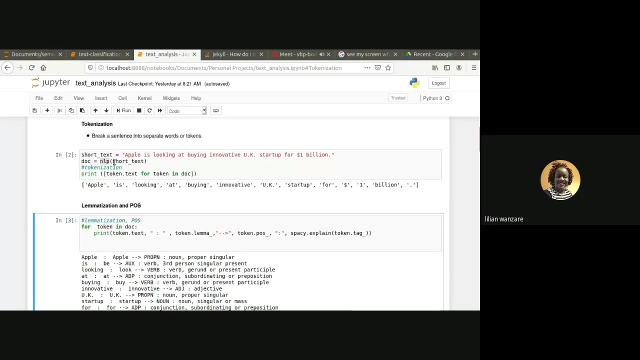 You can see that a billion is a cardinal value and the full stop is a punctuation. okay, The dollar sign is just a symbol of currency, So really it kind of breaks down your text. Okay, By just having to do one line, which is you perform natural language processing on your text. 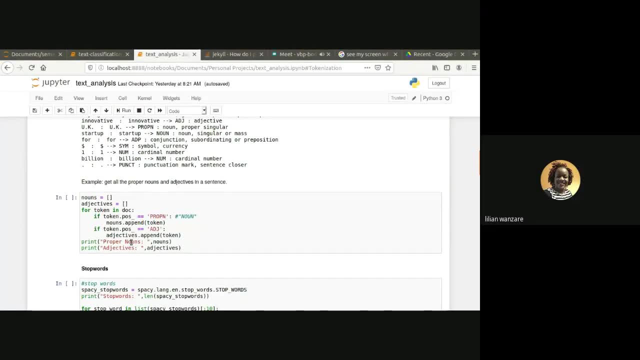 So, for instance, if I say I wanted to extract- I don't know nouns and adjectives, okay, I can just say for every token in my document, yeah, If that token is the part of speech of, the token is a proper noun. you know, save it for me in some list, okay. 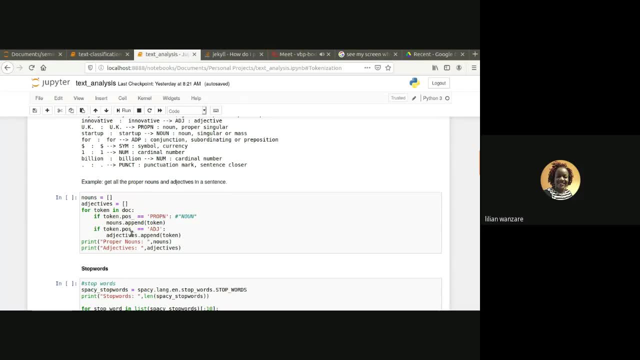 And if the part of speech is an adjective, put in the adjective. okay, Put in the adjective words list. It's like that when I run this it kind of gives for me all the words that are proper nouns and all the words that are words adjectives. 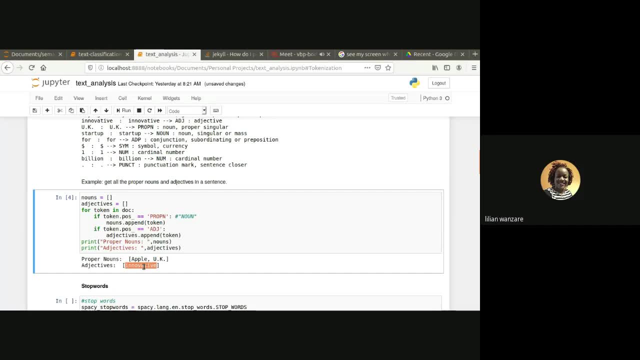 You can think of whatever thing that you want to do. okay, So it enables us to kind of map all those aspects of our text. okay, So we are now. we are now understanding more or less what is this text? 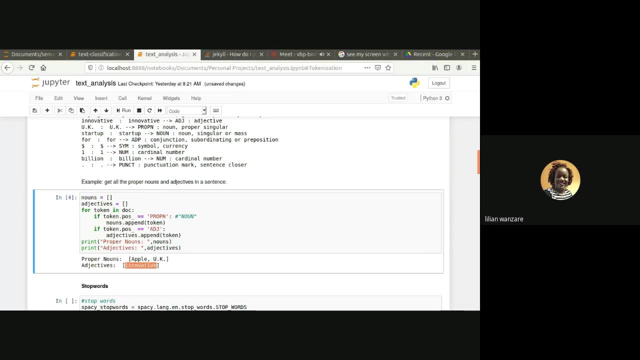 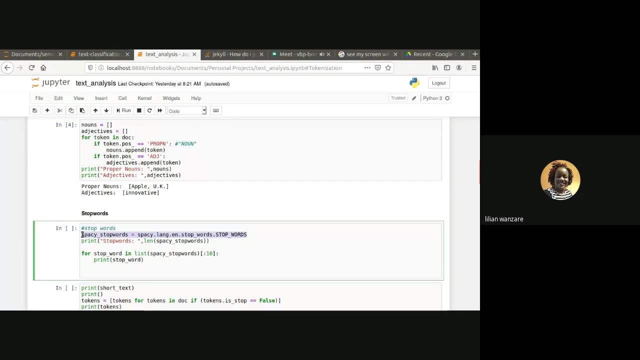 You know about, You can do the same to stop words. yeah, So you have to load the stop words. So you can. it is this command of sparselanguage, the English stop words. yeah, So you call sparse, you call the language, the language is English, and then you want us to load the stop words. 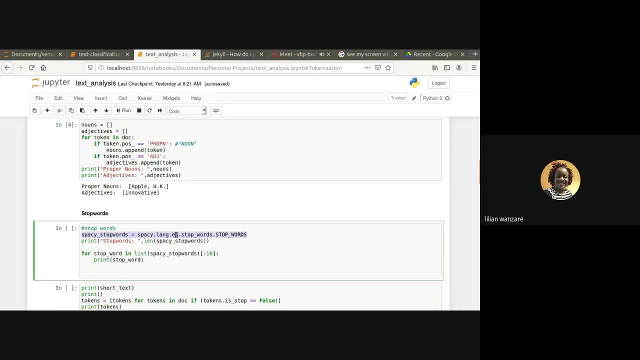 There are many languages in sparse. Sadly, there is no African language. yeah, I think. I don't think there is one in Swahili, I'm not sure. even if it is there, okay, But you're able to load it. 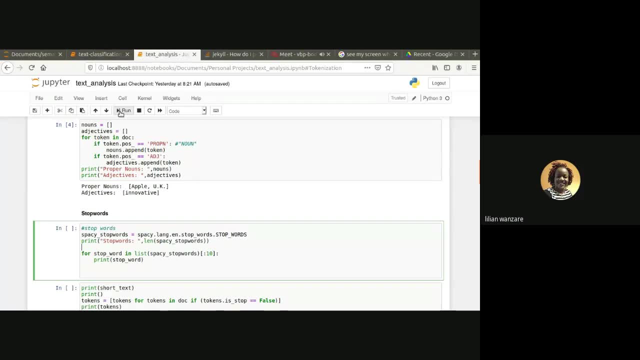 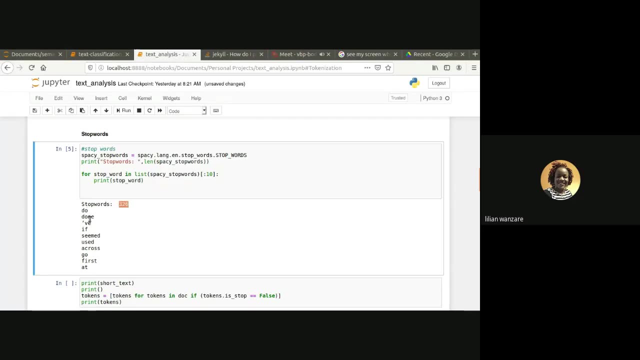 Okay, So here are the stop words. So let us look at some examples of stop words. So in sparse there are around 26 stop words like do, done, if seemed us. okay, If I run again, you can get another set. 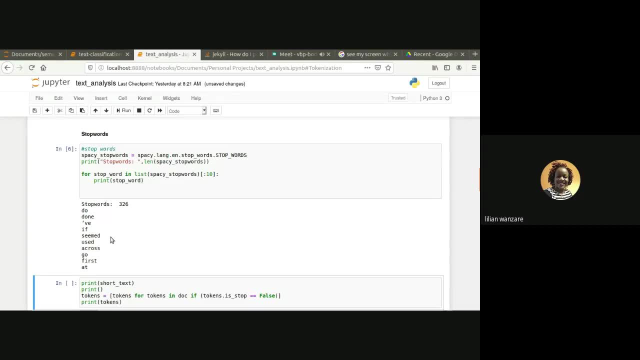 Across, go fast. okay, So these are just derived from large texts and they look at, like you know, the top 300 most occurring words. Those become what? Stop words, for instance. So just a dictionary of a list of words. when I think about it, 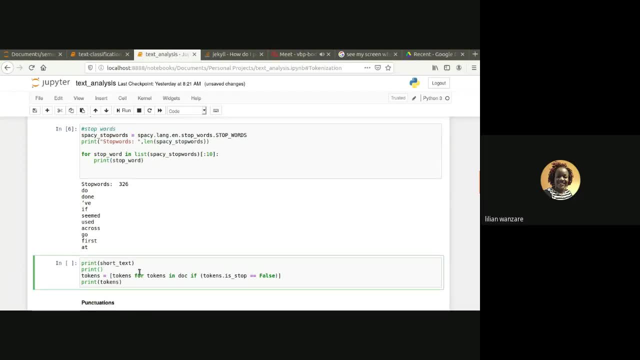 So that means, if I want to extract only the words from my text that are not tokens, I just want to extract all the tokens from my document where the token is not a stop word. yeah, The stop word is false. okay, So what that does is these are the original sentence. 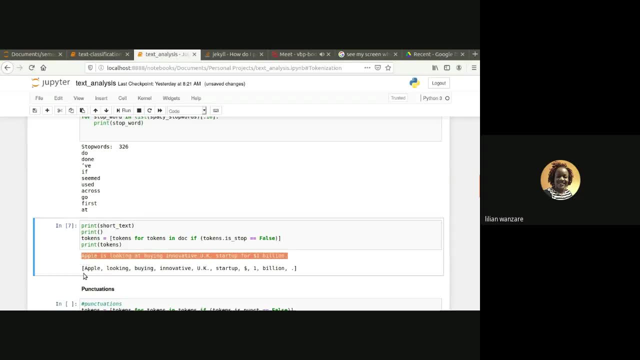 So, for example, it's looking at buying innovative UK startup. and then this is the list of tokens, without the stop words. You see is has been removed, at has been removed and I think for okay. So you know you only have the content words. 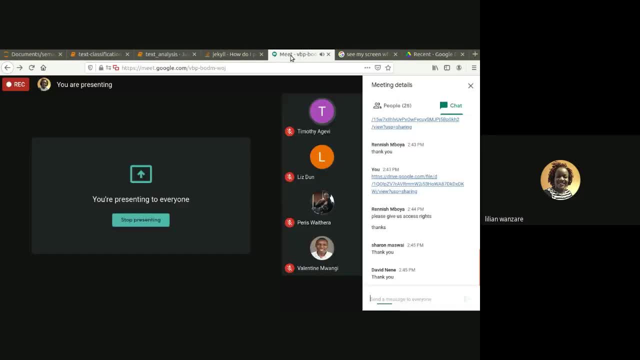 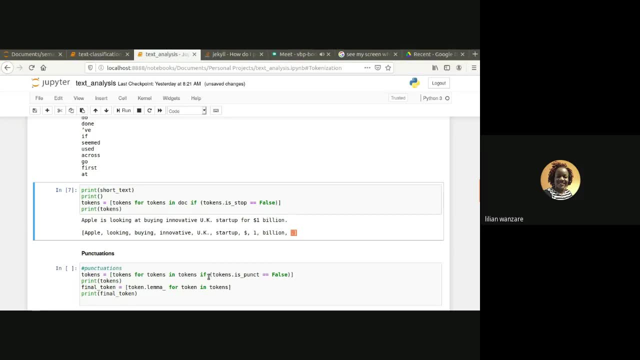 We still have punctuations, though We haven't removed the punctuations. okay, The punctuation can also do the same way. You just call the same function: Token is punct or is punct? It's false. So you only want to select those tokens where it is not a punctuation, okay. 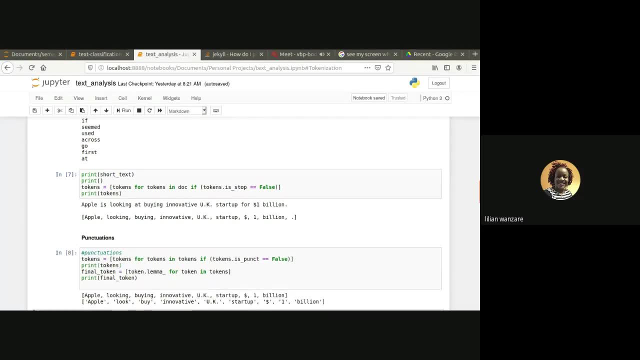 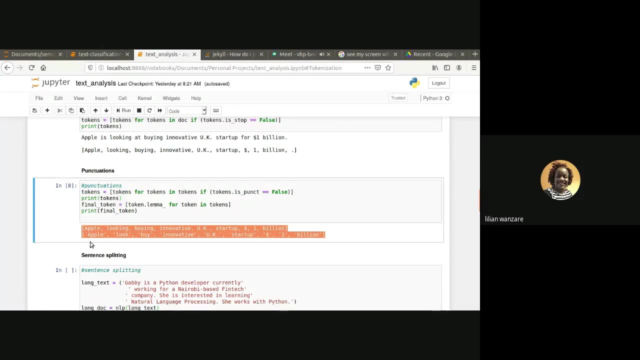 And if I combine all that, what we now left is this: okay, After you do tokenization, you remove the stop words, you remove the punctuations and you lemmatize. What is just left is the final tokens. You call: look, buy innovative UK startup. you know. 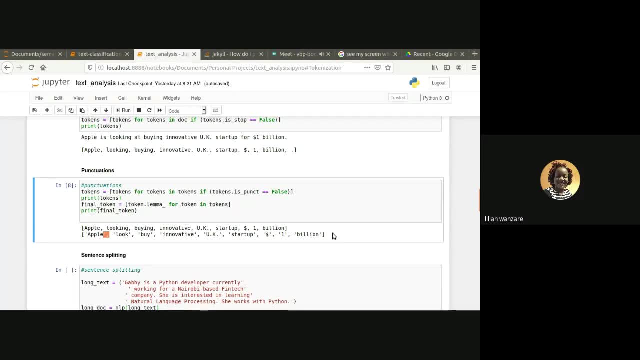 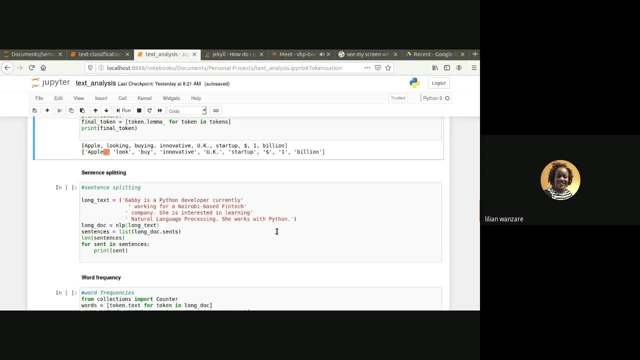 So this is now our kind of the contents of our document, our short document. Any questions? so far? So I'll just proceed As I said, not with the tokenization, but again, if you have a longer document or if you have a certain long text, okay. 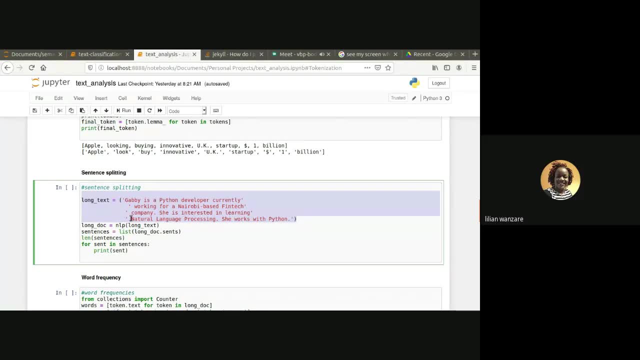 Gabi is a Python developer currently working for Nairobi-based fintech company blah blah blah. You still perform the same NLP on the long text. Remember, NLP performs the whole NLP pipeline, from sentence splitting to tokenization, to speech tagging, plus others that I haven't talked about. okay. 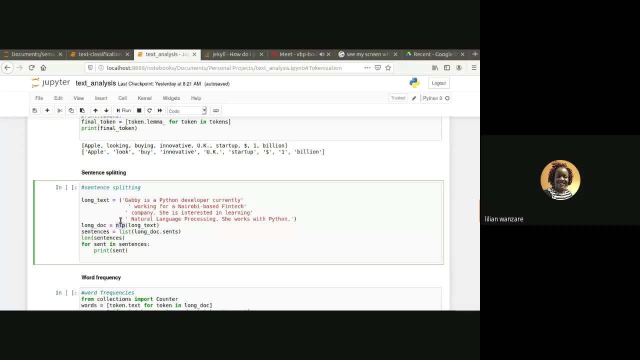 So it really does all those on your provided text. Now, if I want to look at what are the sentences in my text, okay, I just called my sense And I say: okay, from the NLP, give me all the words, sentences, yeah. 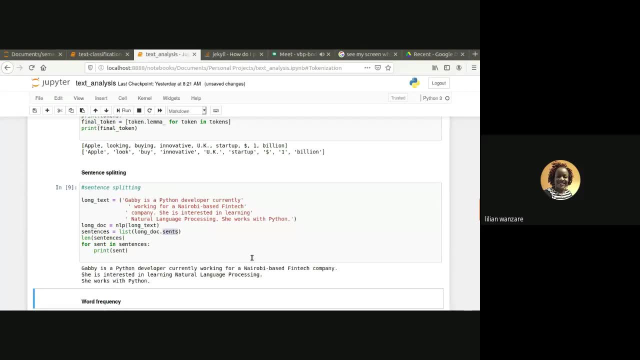 And if we run this, we get the individual sentences. yeah, Every sentence has been split correctly, So we have three sentences from our document. okay, So just by doing NLP, you're able to perform the whole NLP pipeline. 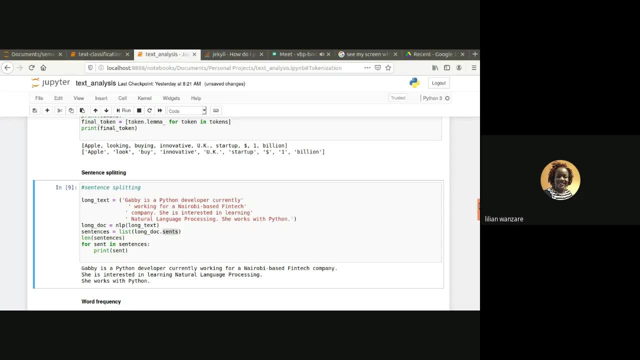 And that's why sparse is quite applicable, especially for people who don't have to really worry about the nitty-gritty. So that's why we have split our document. So you can imagine, if you have this document, you can also print out the tokens. 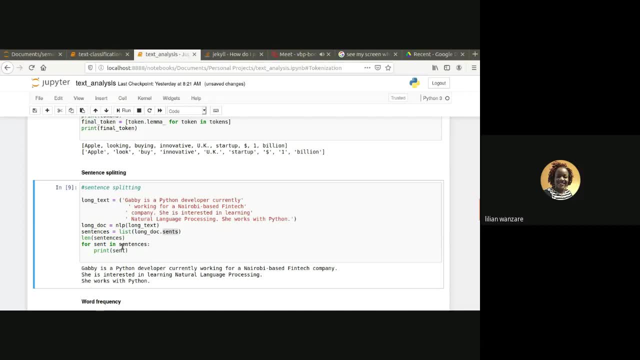 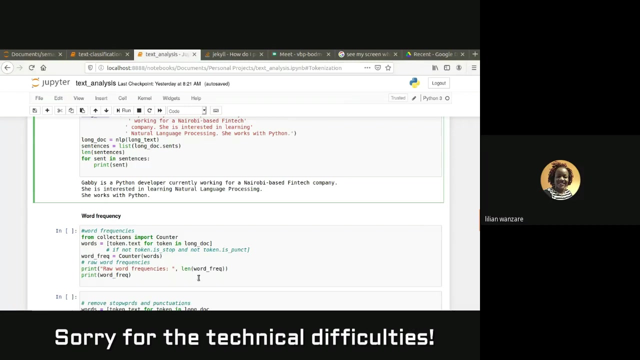 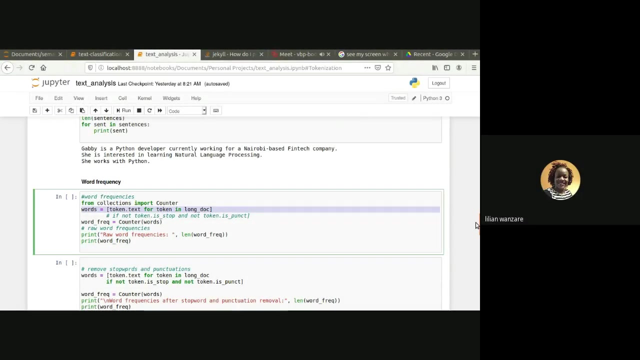 For every sentence we'll print out the what, The tokens. For every sentence you can print. you can remove the stopwatch, you can remove. Okay, So we are at word frequencies. Okay, So we keep on moving between the presentation and the chat just to see if someone's asking a question. yeah, 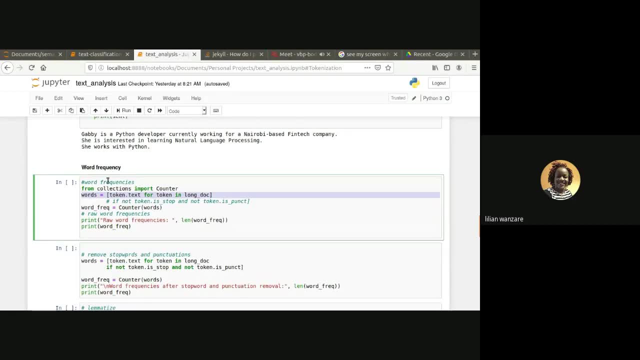 Okay. So if you want to now just look at the word frequencies, Now we just get all the tokens from our long document. All the tokens will now be our words, okay, And then we count how many words we have. So in this first part, what I have done is I have just tokenized it. 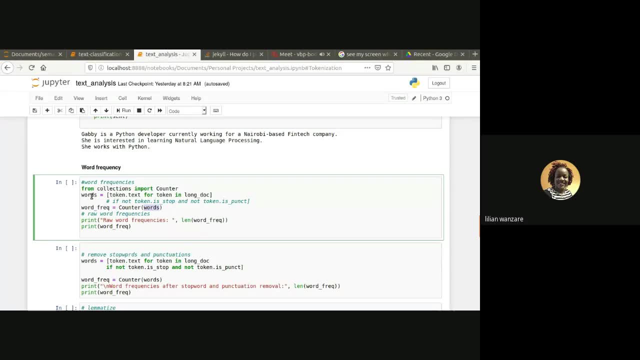 I have not removed any punctuation, I have not lemmatized, I have not removed any stopwatch. So if we run this, we see we have 23 words. Okay, Even a full stop is counted. There are three full stops. 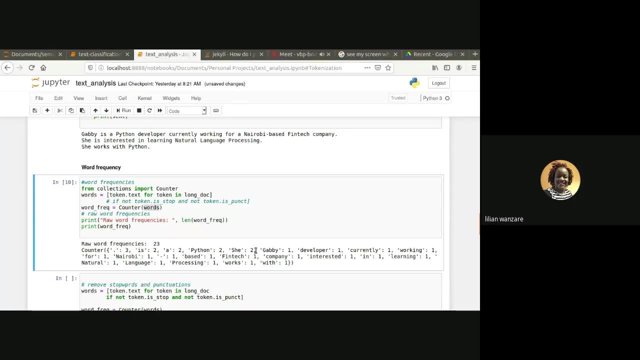 There is is, there is a, there is python, there is she, there is gabi developer. Okay, So here I've just taken, I've just only the tokens. Okay, We have 23 raw words more or less, or raw tokens. 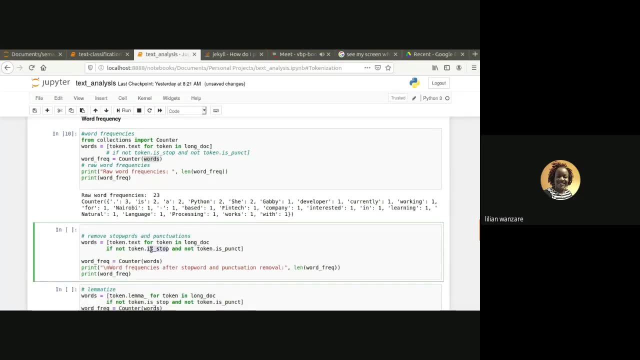 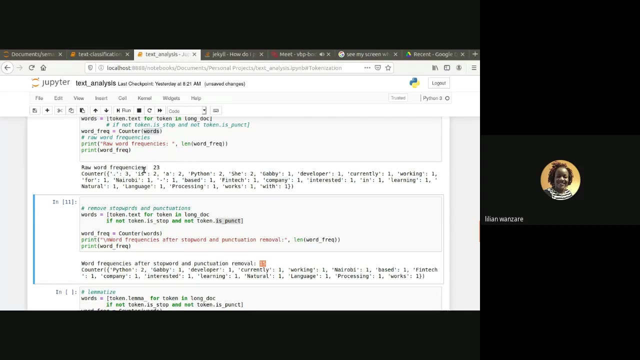 Now, if I remove the stopwatch, The stopwatch, and I remove the punctuation, So okay, What I am left with now is just 15 words. Okay, Because now, as you can see here, we don't have the full stop, We don't have the stopwatch is. 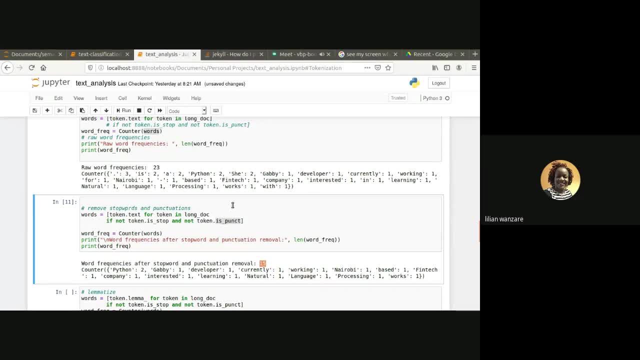 We don't have are and all the other punctuations. So now we only have the words, Only the content words. So you can just achieve that by saying: all my tokens. I don't want tokens that are not there, I don't want tokens that are stopwatch. 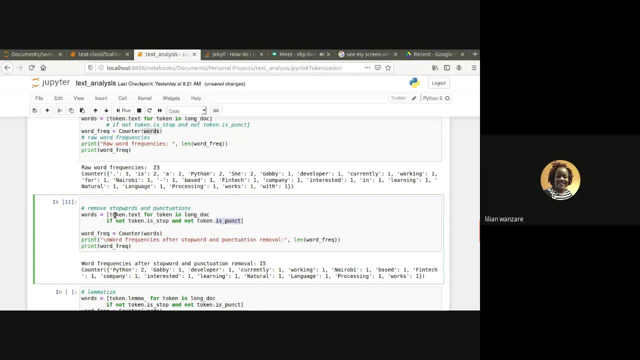 I don't want tokens that are what Punctuations? But give me every other token. Okay, So that allows us to get the number of words in our document. You can go a step further. and now we just don't remove the stopwatch. 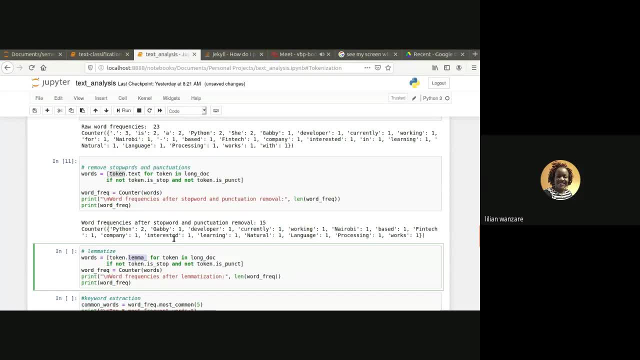 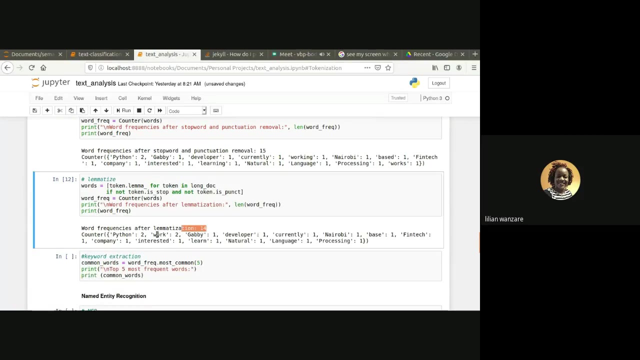 We now lemmatize. Okay, As you can see, here working is counted separately and also works is counted separately. But if you lemmatize Now, you can see we have only 14 words, Because now work has been lemmatized and now it's counted as one word. 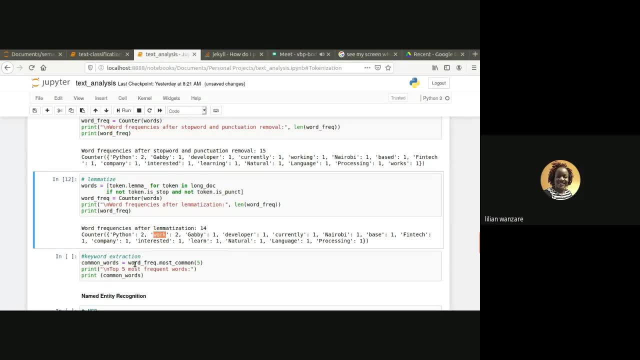 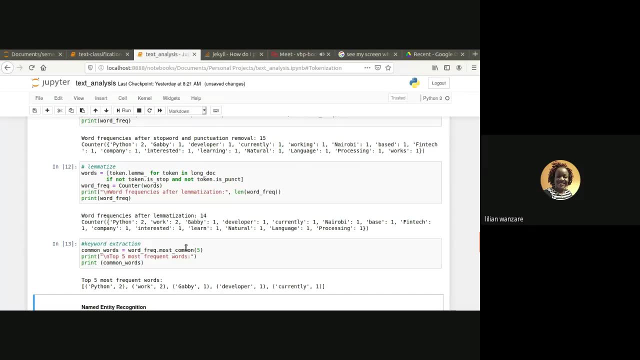 Now if you now want to know what are the top most frequent words in your document, you can now just call you know top five, most frequent or most common. That gives you like Python and work. So if you had a longer document you can imagine be able to extract and see what are those keywords in your document. 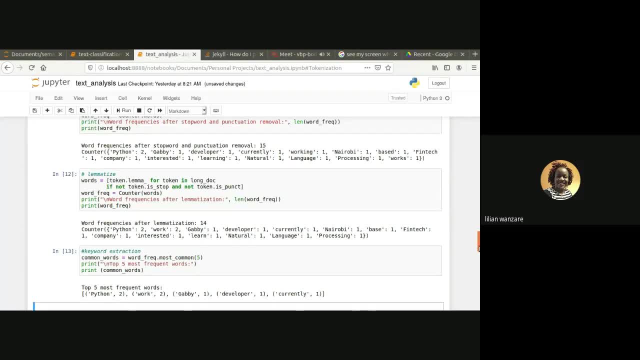 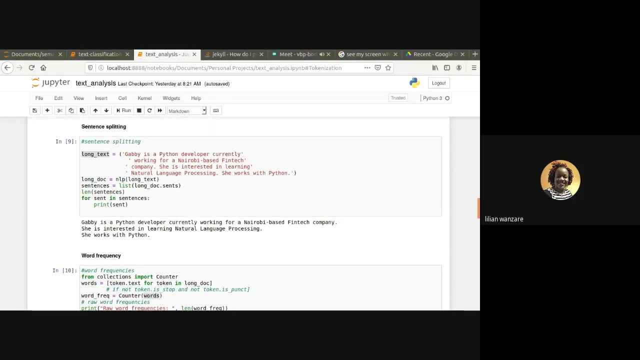 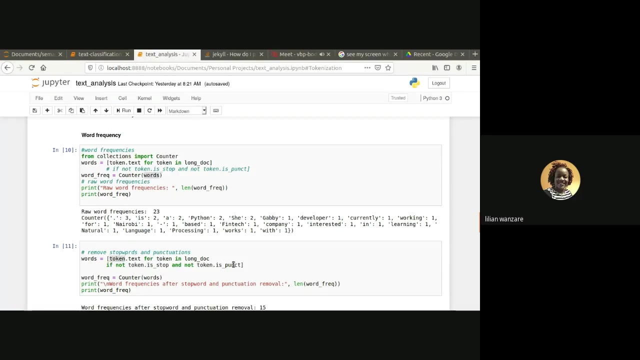 Okay, So that is more or less from: if you have a long. I'll repeat that If you have a long document, you perform the sentence splitting on the document. Yeah, You can be able to extract all the tokens and be able to remove the stopwatch and the punctuations from all the tokens. 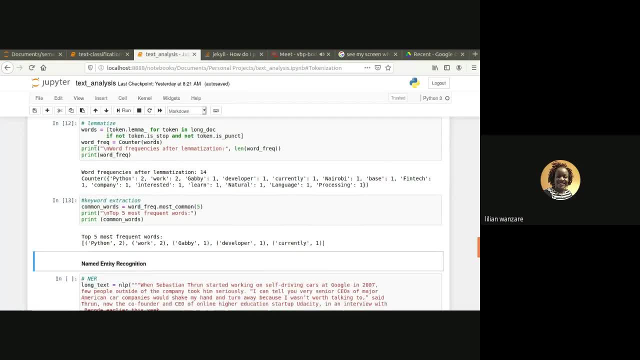 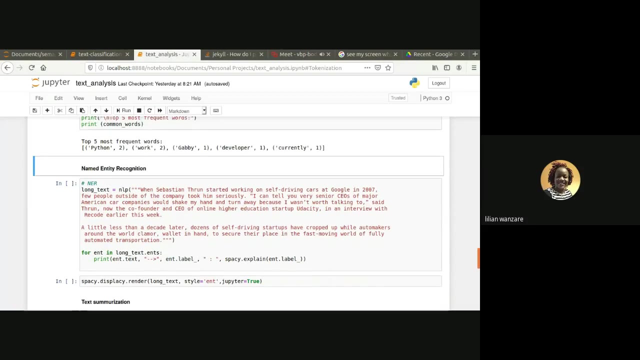 And be able to lemmatize, And that allows you to get the most frequent words in your document. Okay, So far, so good. I hope, Yes, thank you. Okay, Now let us look at some applications. I'm already running out of time for the next half of the presentation. 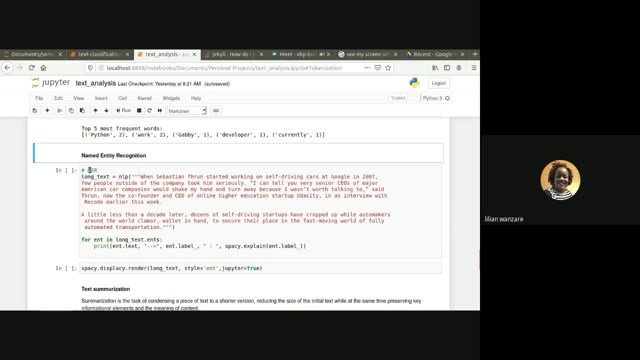 If you wanted to do like NIMT, entity recognition. Okay, So now you have a really long text, a longer text. Yeah, Again, you can just call NLP on your longer text. The beauty: NLP does that, NLP does the whole NLP pipeline. 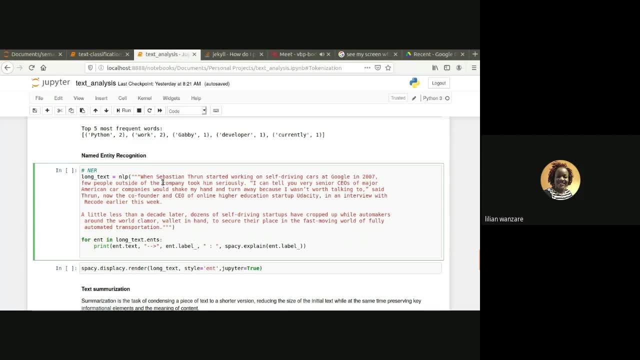 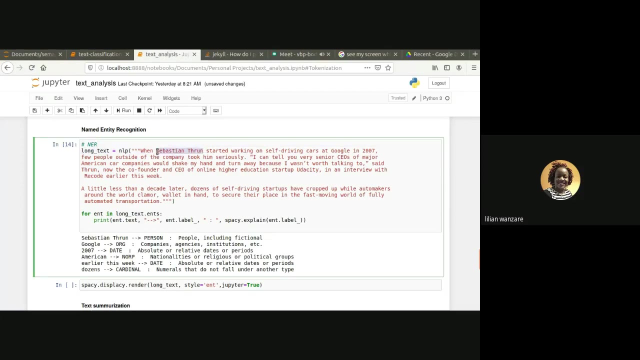 That is the beauty of sparse. Now we are not looking at the tokens, We want to get the entities. Okay, Let me run this so that you can see The entities. for instance, it has identified that this, Sebastian Thrun, is a person. 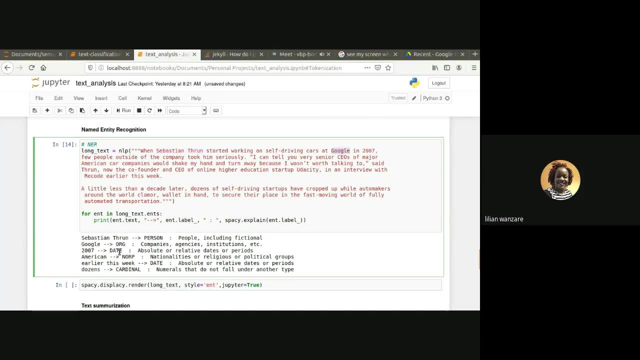 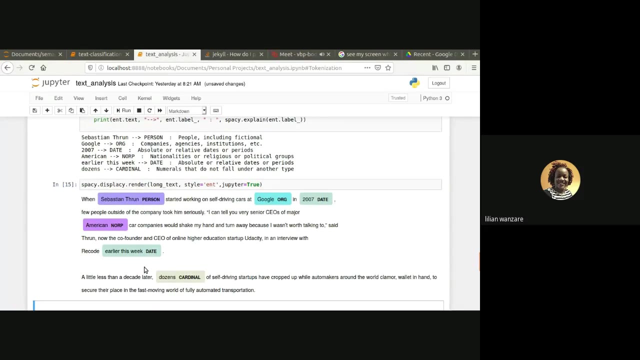 Okay, Google, which is here, is an organization. 2007 is a date. American is a nationality. All this, Let me visualize this. So if I render this, it gives you a nice view of your document, where all entities are. 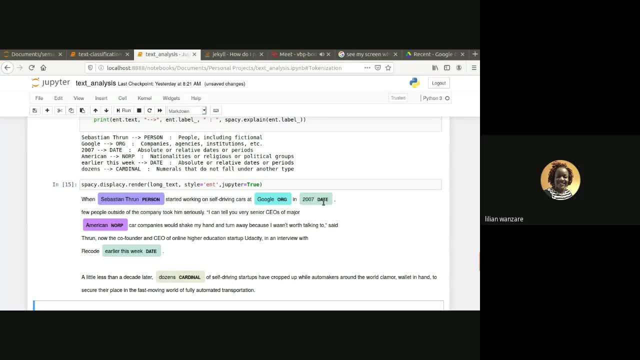 what Highlighted, Okay. Now, if you want to do relation extraction, you can just say, for instance, this: Sebastian Thrun started working at Google, Okay. Or Sebastian Thrun started working at Google on this particular what Date? 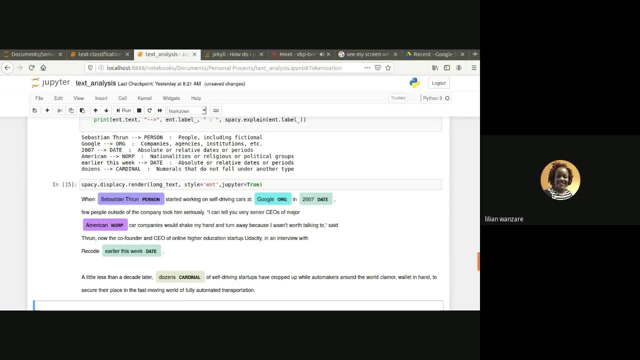 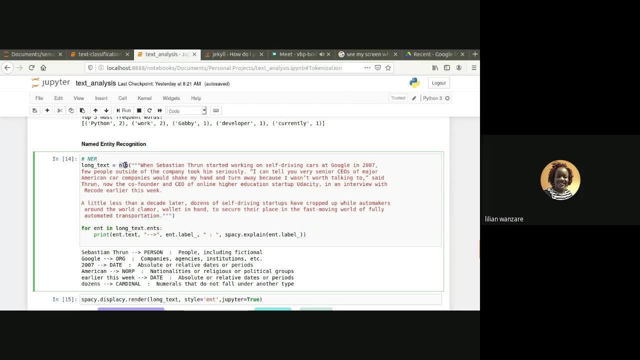 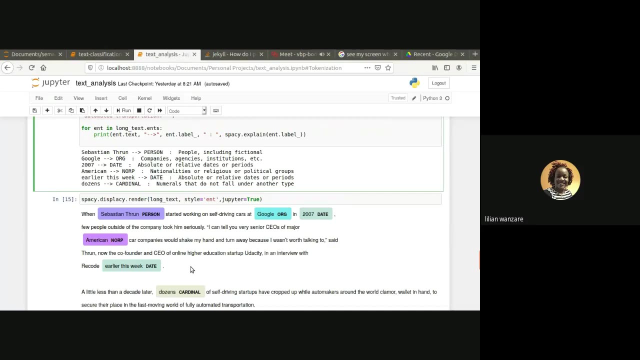 So all this is possible because we ran NLP on our document. behind the scenes. It did sentence splitting, organization, part of speech and everything, and now enables us to extract the entities from the text. Okay, And now you're able to see what is your text talking about. who are being mentioned in? 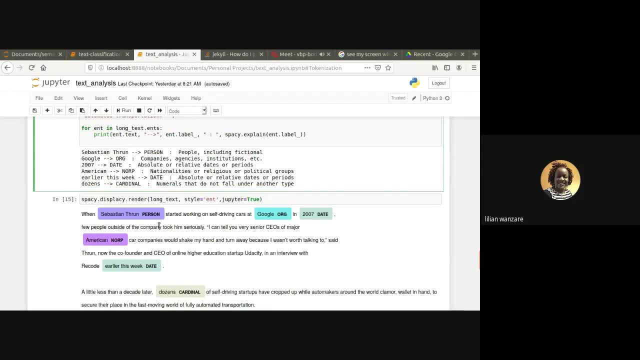 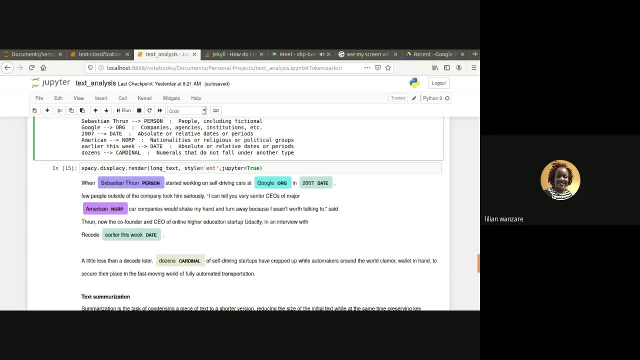 the text. So the text is about this Sebastian guy And we're looking at Google and something about him, more or less Okay, So that's really one application. The last application that I'll talk about in this first half is text summarization. 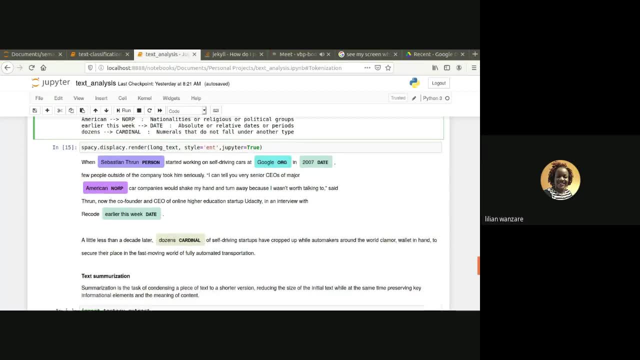 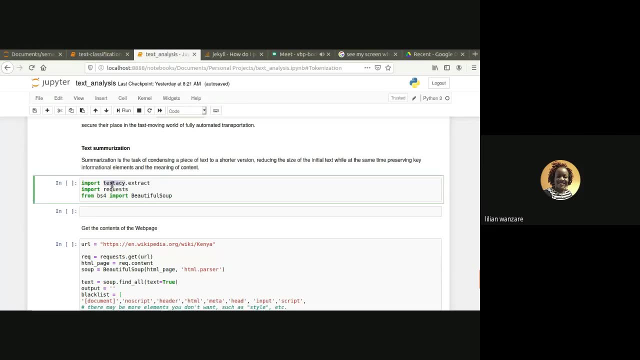 Okay For text summarization. we need something extra to enable us to do that. We need to install this. It's called text to save. It runs on top of sparse. Okay Request enable us to get data from a web address. 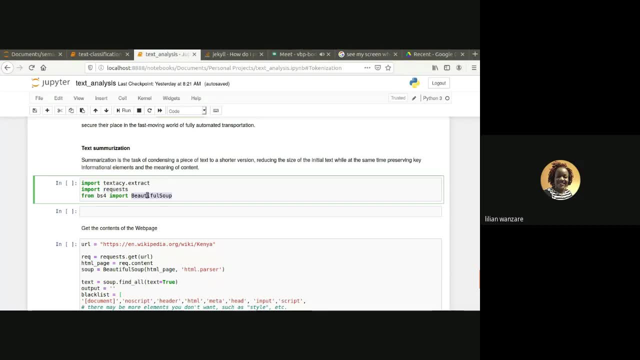 Okay, Request Beautiful soup. enable us to extract information from a web page or an XML from a web page, So I just combine those two. Okay, So now you want to know what is Wikipedia Kenya talking about? So our URL is just a Wikipedia document for Kenya. 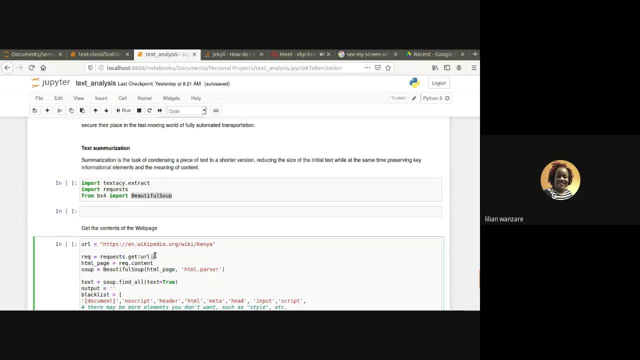 So we ask the requests to get for us the contents of this document. Okay, So it goes online and gets the contents of the URL, And then we get only the content. What is the next part? We get the content, Then the contents of the URL, we pass it through. Beautiful Soup. 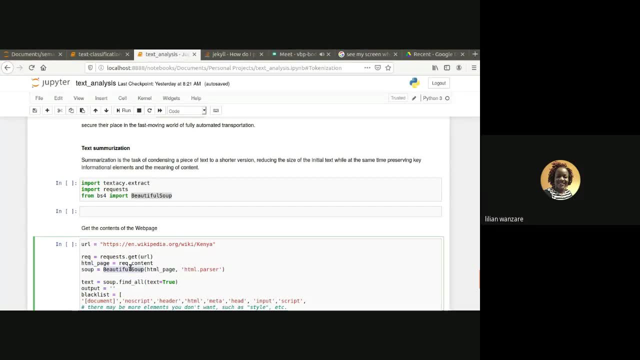 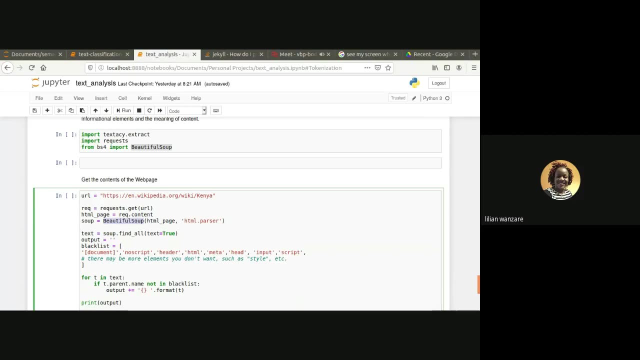 Yeah, And Beautiful Soup only extracts the text part of your document. You can do more with it, but mostly you can just want to extract the text part. Of course it's a document. Of course it's a Wikipedia. It has, if you're familiar with HTML, there's a lot of tagging going on behind the scenes. 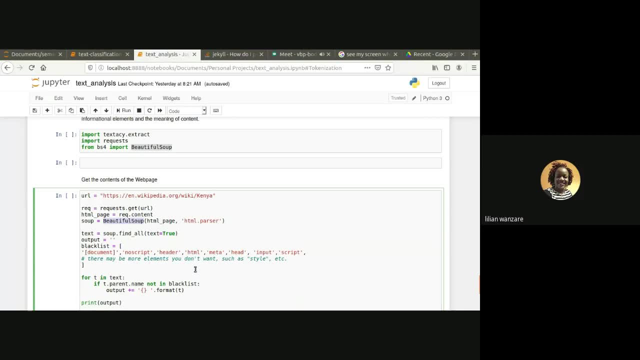 So there are some tags that you're not interested in. Okay, You don't want the metadata, You don't want the head or whatever other tags you don't want, So I'm just going to remove everything that is in this blacklist. 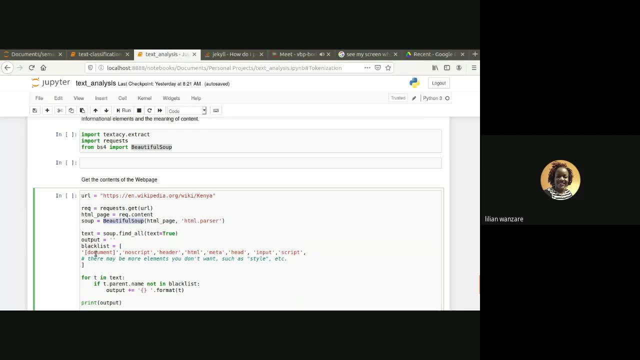 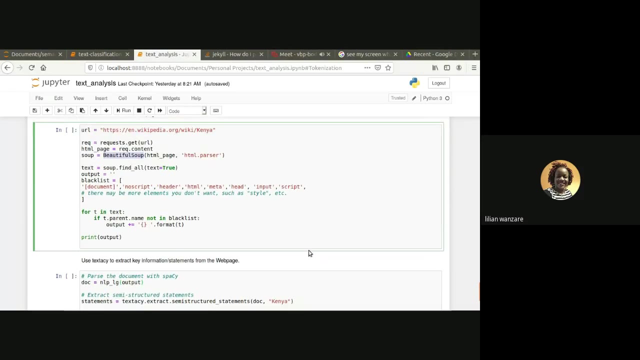 I don't want those tags to appear, So only give me the text part of all the tags in the HTML page whose parents are not in my blacklist. Okay, So when I run this just a minute, The output: oh, it takes some error. 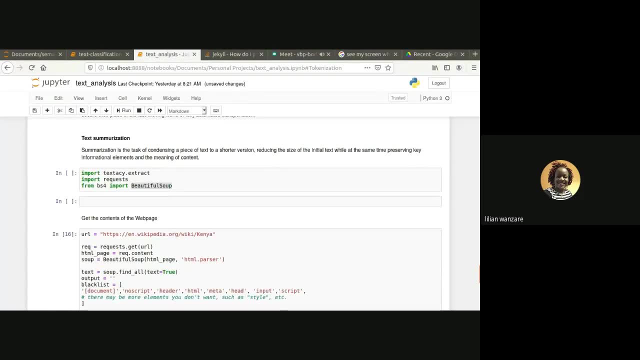 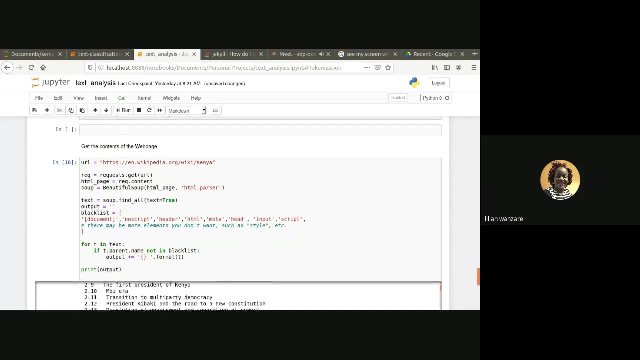 What is the error again? Oh, requests. I didn't run requests. Sorry, I have to run this one first. I have to load the requests first. Okay, So now you've loaded the requests. Okay, So the output you can see. it has taken everything in blacklist. 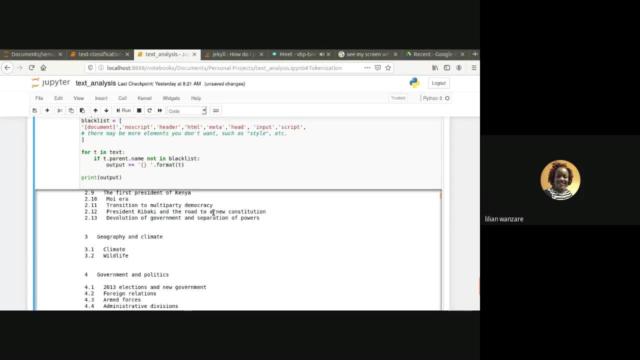 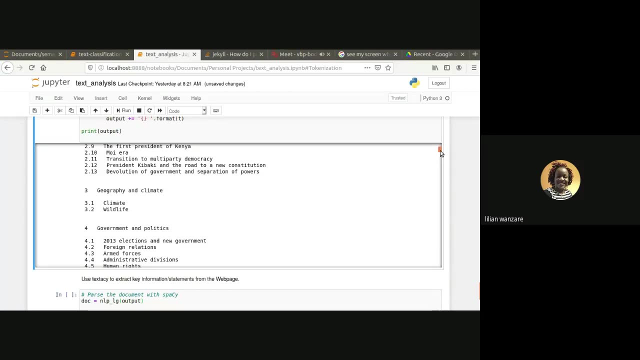 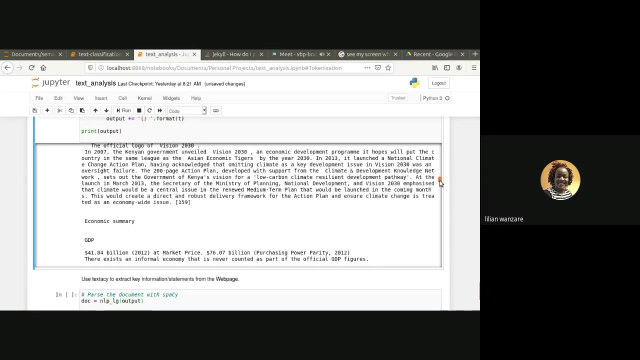 Okay, It's taken everything in our Wikipedia page. Okay, Sorry, It's just all the data on the Wikipedia page. It's a lot of information You can imagine. The history of Kenya is all in the Wikipedia. So just by using Reapers and Beautiful Soup, you're able to extract information from a. 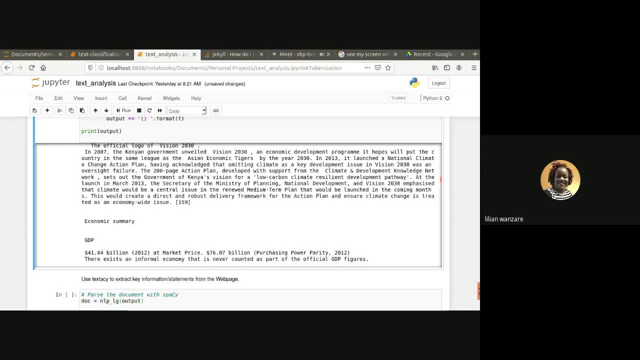 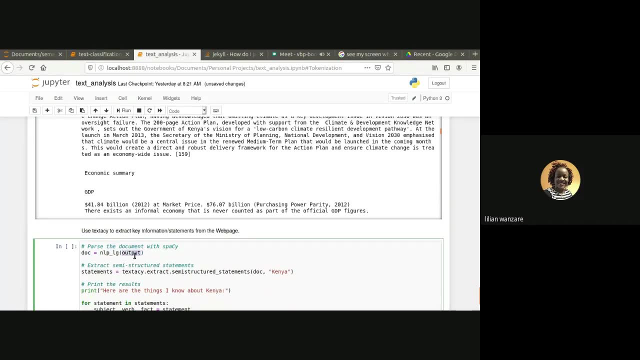 web page. Now let us do NLP on that web page, Okay. So we do NLP on our output, Okay, On our Wikipedia page, And then we use this text, you see, to extract for me the key information that I want from. 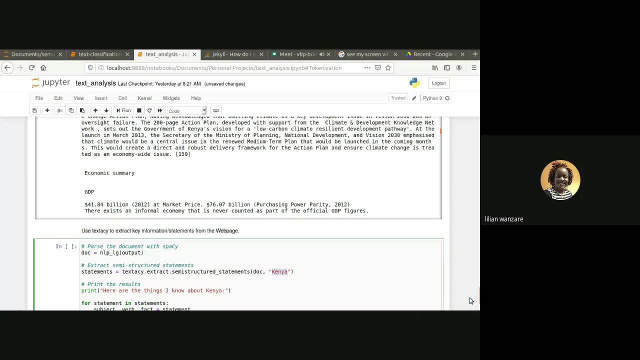 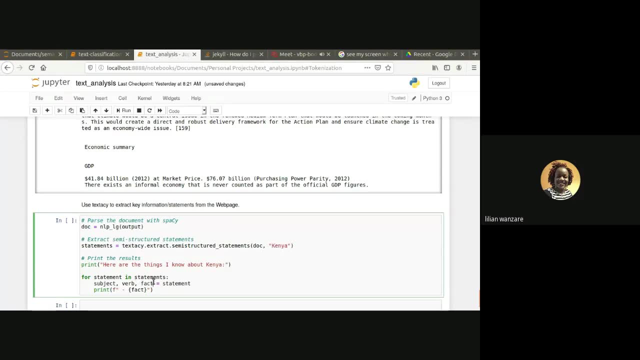 that document that talk about what? Kenya, for instance. Okay, All of them are going to be statements in the form of subject verb and then the fact about that statement. So the cool thing about this is, when you run that it takes a bit of time when you 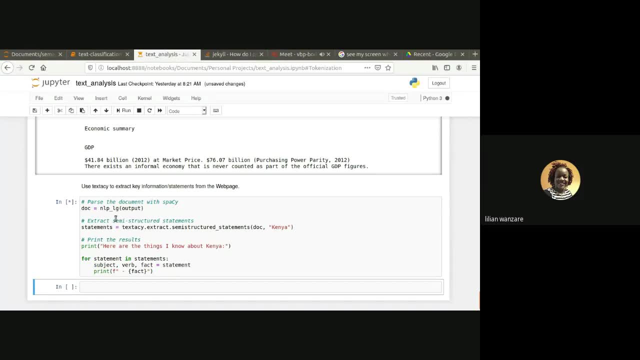 run, that NLP behind the scenes is going to show up Behind the scenes, is able to perform the whole NLP pipeline. And then the text you see is going to extract semi-structured statements from our document that talk about what Kenya. 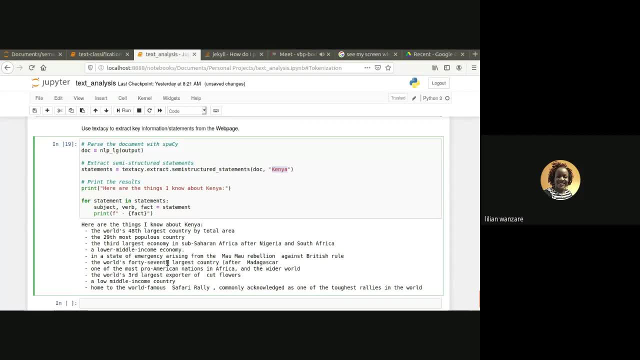 And what you have is just a list of summary of the Wikipedia page. Okay, That says like: Kenya is the world's eighth largest country. the ninth most popular country, you know, is the home of the famous Safari Rally- coming for the toughest rallies. 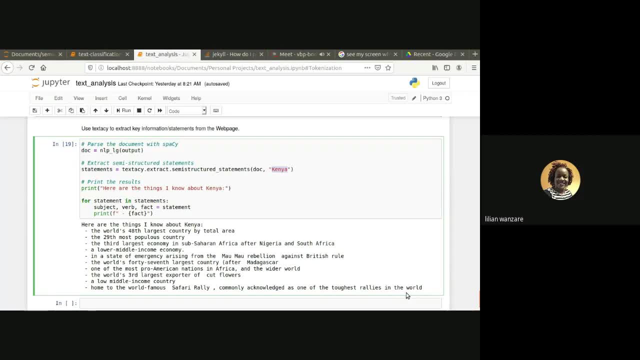 in the world. So, you see, it enables you to extract, like, a summary of a webpage that you're looking at. Okay, That enables you to really, in a nutshell, just get the gist of what the page is talking about. 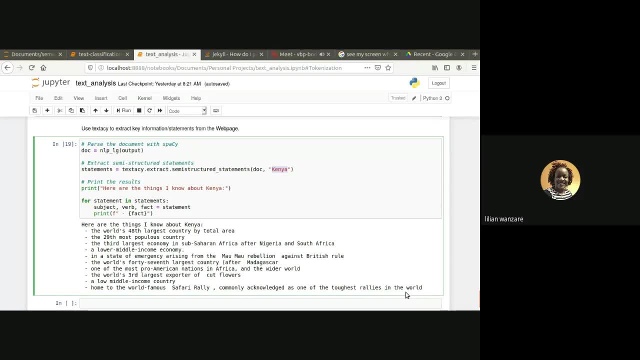 And all that is possible because you're able to do the whole NLP pipeline using SPARC And on top of that use Dextasy to extract the semi-structured information from our document. Okay, So that is really just to entice you to try out and see. 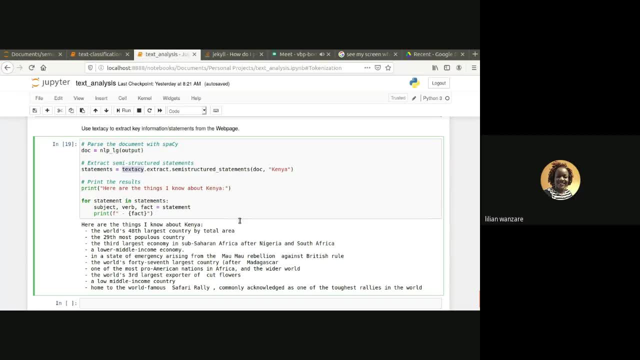 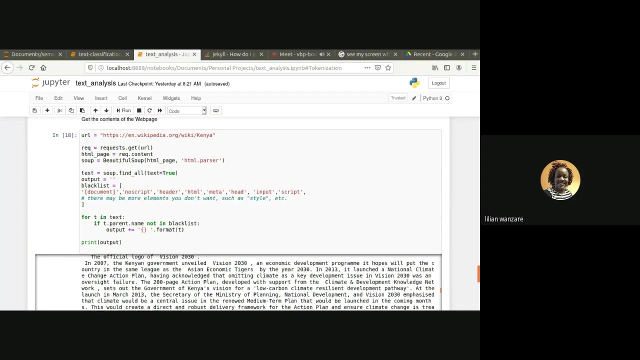 But you can be able to extract from different pages of your choice Any questions. so far for the first half of this presentation, So I hope of course you cannot learn everything today, But I hope the presentation gives you a kind of you know zeal if you want to learn more. 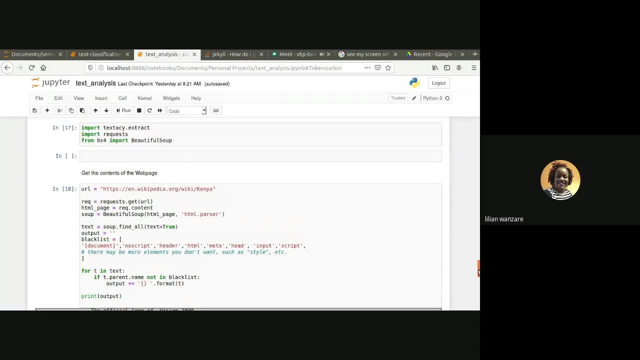 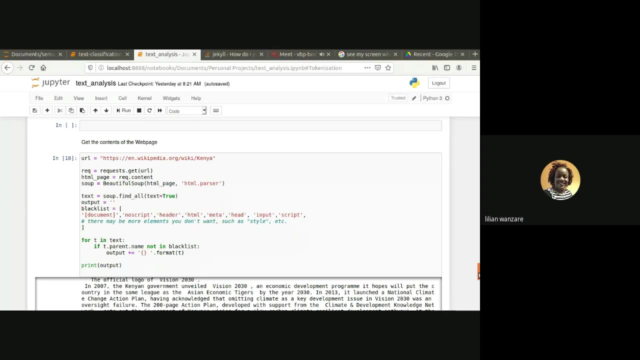 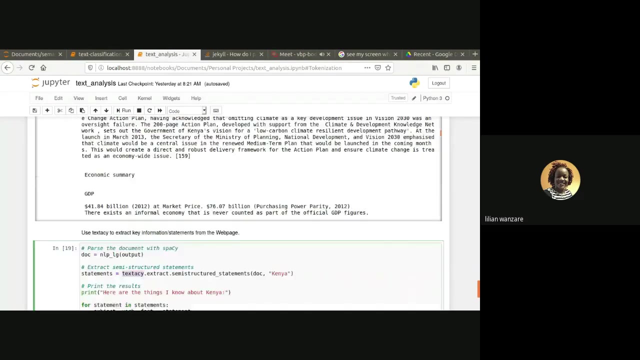 about, you know, text analytics in general and practicing in different applications. There are many tools outside there. One of them is just SPARC, But there are several other tools that exist That are also enabled to do text analytics, Questions or comments. so far before I start the second half. 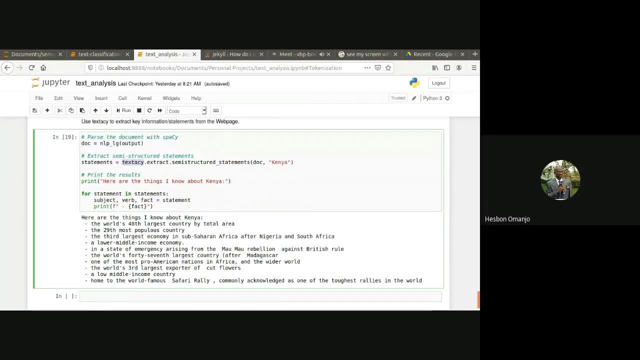 Hello Linda. Yes, Okay, Thank you for your presentation. Yeah, It looks very, very intriguing, And my question really was about how you implement SPARC in normal, basically your normal work, day-to-day work, Because Hi. 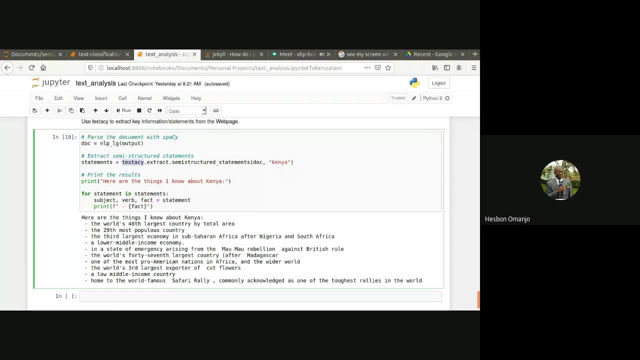 The tools NLP. Yes, So I know you can actually take an offline dump and then you run the tool on it and do your language processing. Yes, And now you talked about something which is interesting, which is HTML passing, and then 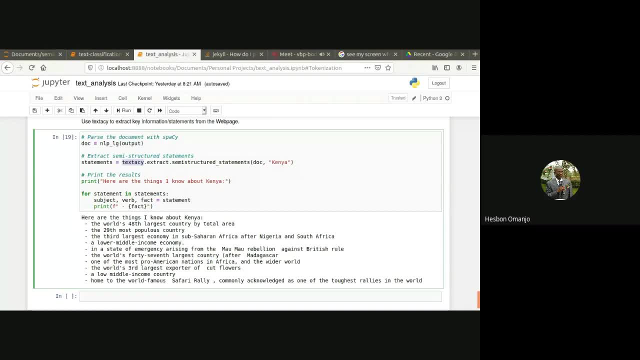 basically look at that. But have you done an integration with an application before, Like, for instance, if later you know there's data entry logs logged into a certain tool of choice or an application in a bank, for instance? Yes, And then they are capturing data. 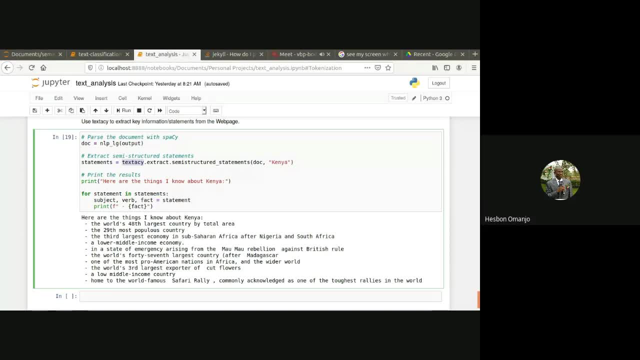 Do you have any situation where you have run this on the background, interfacing with that application through some EPS? Yes, And then this Mm-hmm, It's possible. Yes, Maybe just give us an idea about that and such You can have some expectation as well. 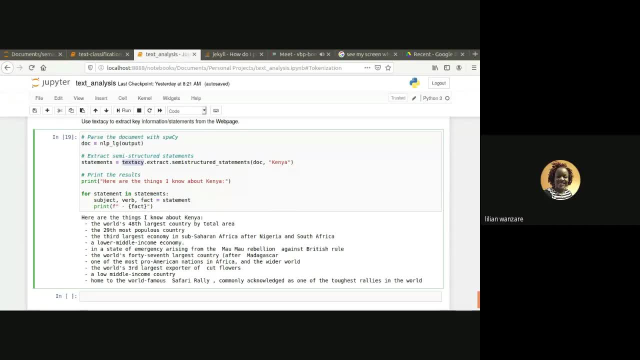 Thank you so much. Okay, The beauty One of them is: You know all of this. it's kind of The main question is: how do you, Once you have your model, for instance, yeah, how do you expose it out as an API, for instance? 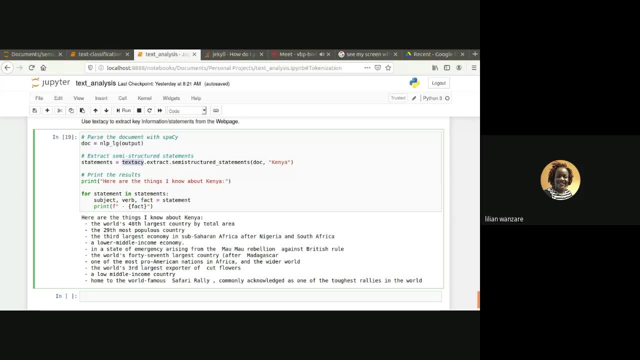 if you so wish. Okay, Yeah, Yeah, Yeah, If you so wish, Okay. So the fun thing about most NLP: you find that you get like what you have said: you get a lot of data. you build your tool, which is more or less kind of a machine learning. 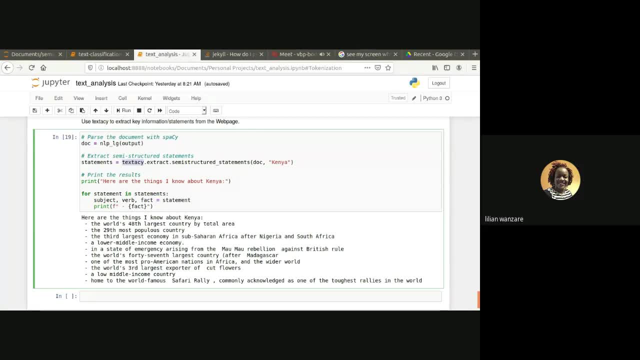 model. Okay, The only thing you need to do is to expose that. Okay, And now that is another level of how do you expose our tools. Okay, So it's really really. There are already tools there which you can talk about in another session now in. 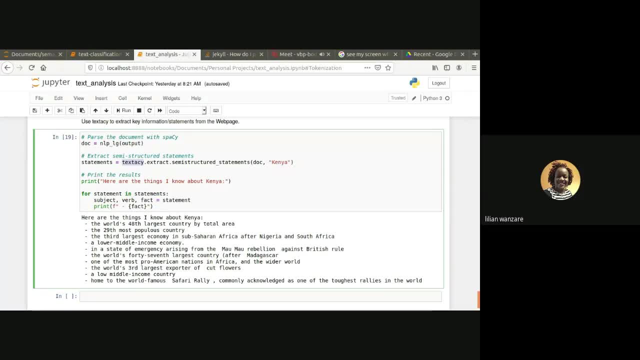 a more practical session. Okay, That you can be able to use for that. Okay, So I'll just leave my email after this and anyone who has some specific question like this one, we can talk about it in a certain Because some people could be too high level for them for this particular meeting. 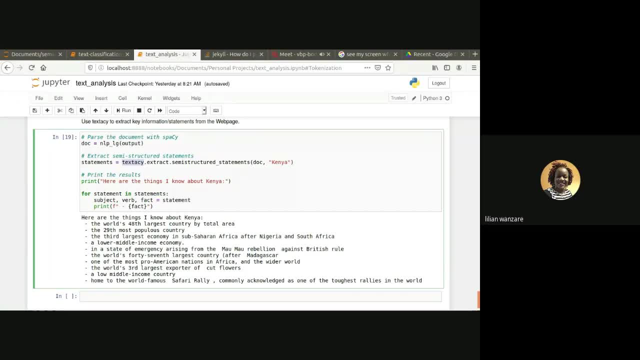 Okay, But you can take up that with you if you're interested. Okay, Thank you very much. Yes, I'll give my contacts after that. Yeah, Yeah, Okay, Yeah, Anybody else? There is a question in the comment section. 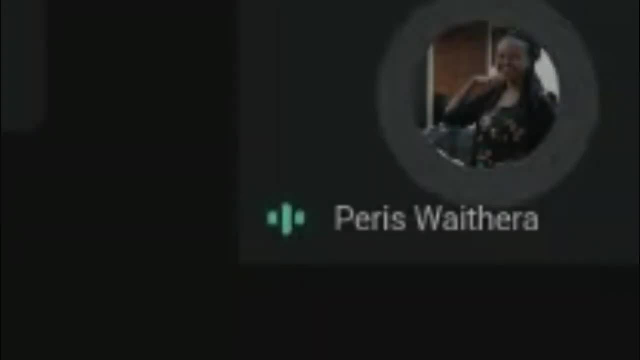 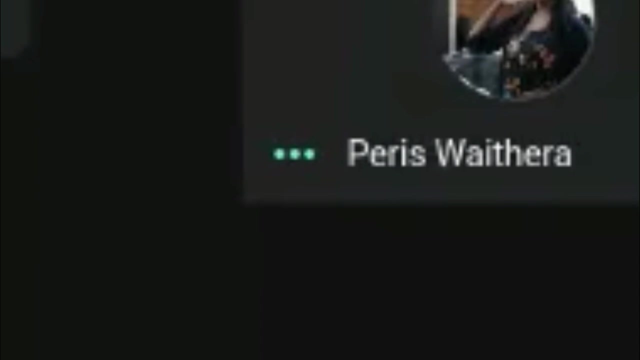 Okay, How would one deal with not sexed objects? ie like emojis, Uh-huh. So there's actually an emoji parser. Okay, There's actually emoji parser. Those are two different issues. There's actually an emoji parser. 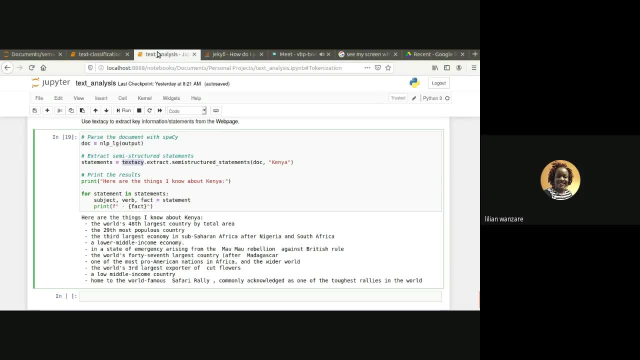 And also one of them is actually on top of sparse but enables you to decode emojis. Yes, That is another application area if you are interested in that. Okay, So that's another area. If you are into emojis, yes, there is an emoji parser for that. 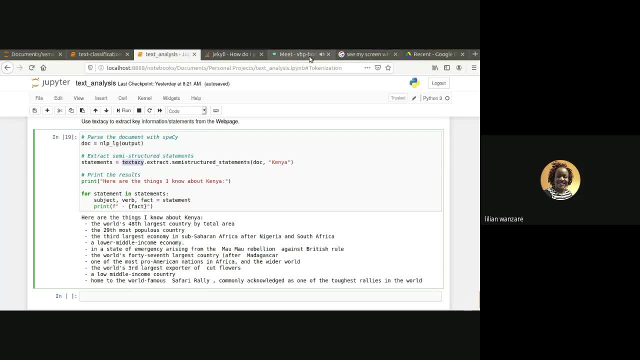 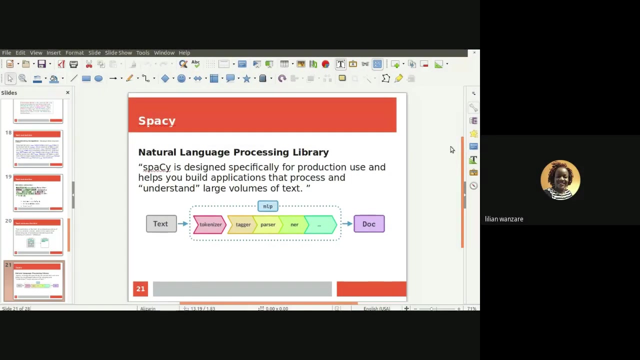 Okay, That's another area of trying to decode what an emoji is all about- Another area of interest for some. Okay, Okay, So there's nothing specific about what I've presented. Then I'll start with the second half. Okay, So we talked about sparse and NLP and the whole NLP pipeline. 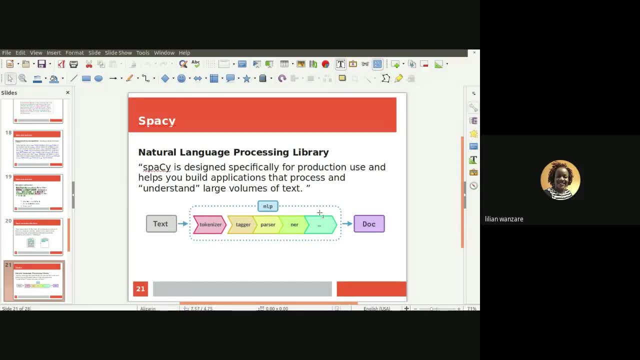 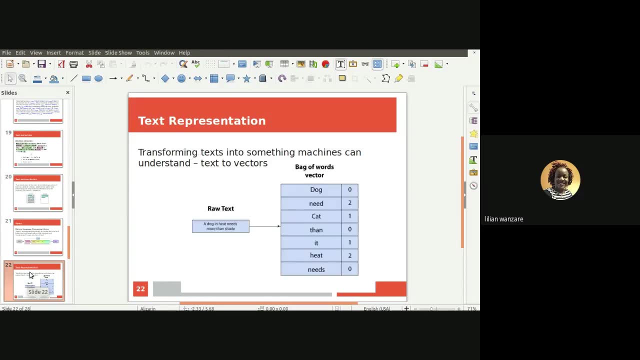 Of course, there are many things going on behind NLP, but because of time I've only picked a few, Okay. So try and see what else is behind NLP Now. I promised to do an application on text classification, Okay. 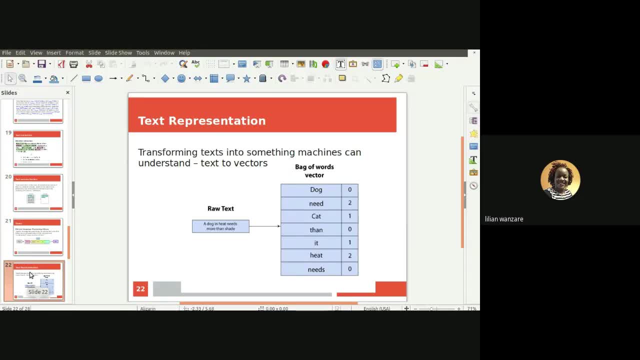 Now to be able to do any kind of modeling on text. of course the language itself, we as humans are able, or we as people we're able- to understand the text Like a dog in heat needs more than shade. 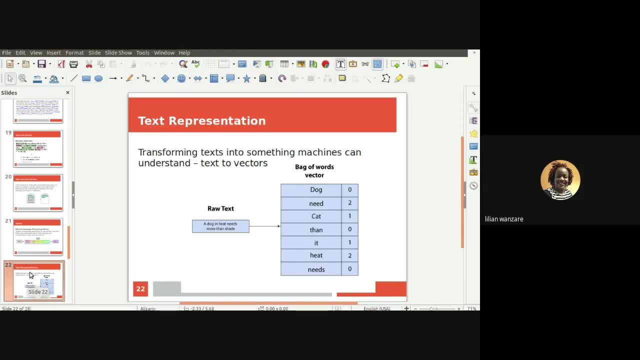 That is just a sentence, But we know machine only understands near zeros and ones at the low level. Okay, How are we able to transform our raw text into a representation of something that a machine is able to compute? That is what is called text representation. 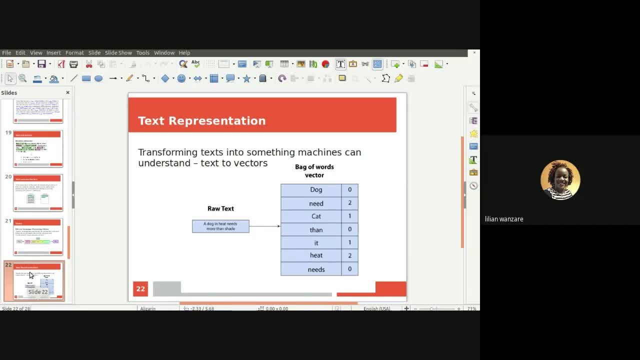 Transforming text into something machines can understand in principle is we're reducing our text to a vector. A vector is just, you know, an array of numbers. You might just simplify it. Okay, Two vectors. I'll give a very simplistic example. 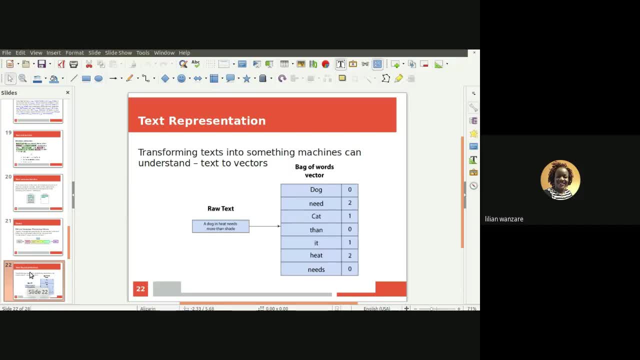 So, for instance, there's a model called bug of words. You take a sentence and then you can imagine, you do NLP on it, You're able to tokenize it And then maybe you perform lemmatization if you so wish. 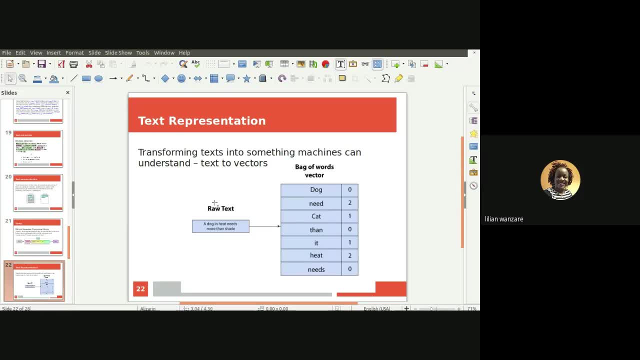 Or you remove the top ones, Okay, And then you just count for every document. how many words exist in that word document? Now, that is possible if for every word. think of it as you create a dictionary. Okay, So you have your sentence. a dog in heat needs more than shade. 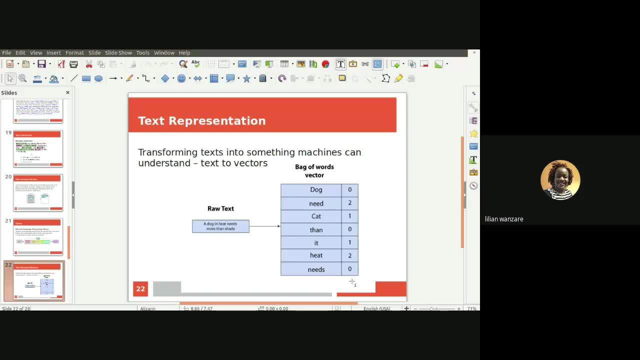 You extract all the words in the sentence And then you create a dictionary mapping of all the words. So, for instance, you can say: dog is position zero, need is position one, cat is position two, blah, blah, blah. It is very important. 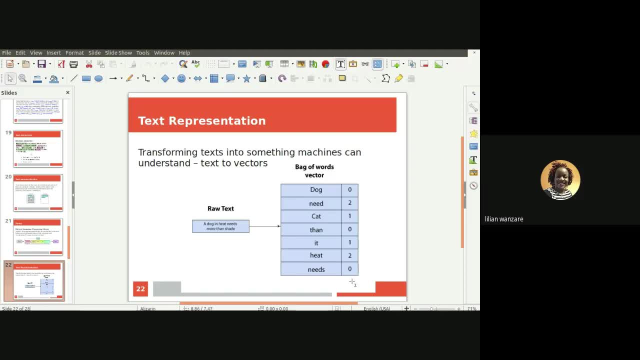 The first thing you have to do is create a vocabulary or create a dictionary representation of all the words in your text, So that when the machine looks at word zero, it knows, like in any document, if it sees word zero, that is a what. 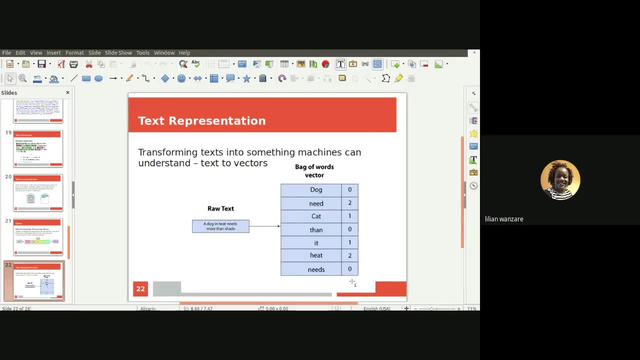 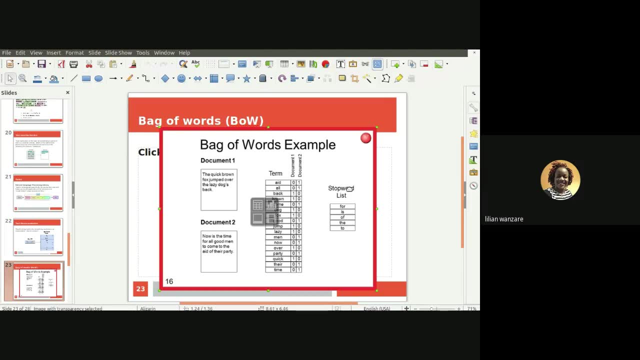 A dog. If it sees word one, that is a need. Okay, So imagine you have such a text. Okay, We have two documents, document one and document two. The quick brown fox jumped over the lazy dog and now is the time for all good men to come. 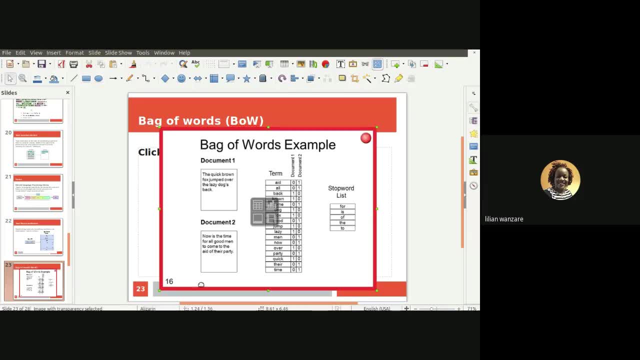 to the aid of their party. You combine all your documents and extract all the words using NLP. When you extract all the words, you tokenize, you lemmatize, you remove top words, blah, blah, blah And then you form a vocabulary of your words. 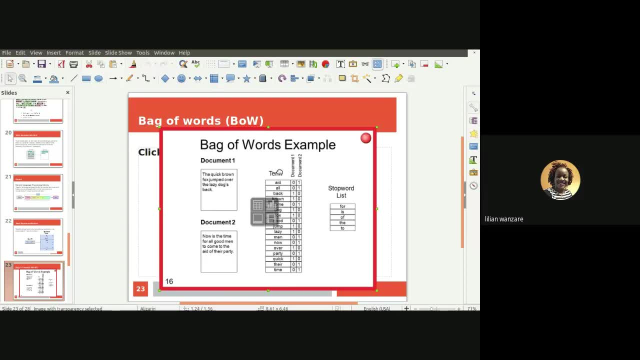 Okay, That is the term. So all the terms in your documents. that becomes your vocabulary Now, because it is a fixed dictionary. you know that position one is for word eight, Position two is all, three is black, four is brown. 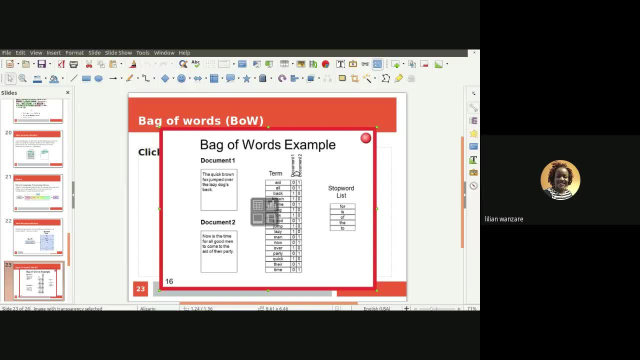 Such that you can represent document one by a zero, or one that represents the presence or absence of a word, Or absence of a word in your dictionary. Okay, So document one will be zero, zero, one, one, zero, one, one, blah, blah, blah, depending. 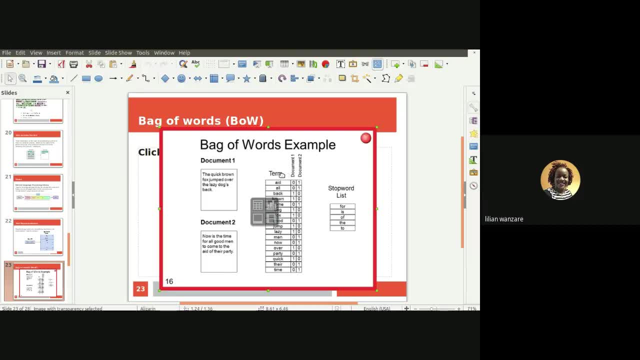 on which word from the vocabulary exists in that word document. Document two again will be one one, zero one one. blah, blah, blah, depending on which word in that word document. So in a way you have transformed your text into a vector. 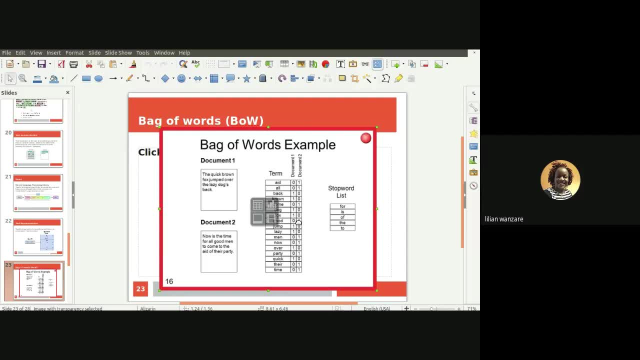 So, instead of each document being just a series of words, each document is a vector. Okay, So a document is a vector representation that kind of captures what words exist in your document. Okay, In a simple way, That is what we call like the bag of words model. 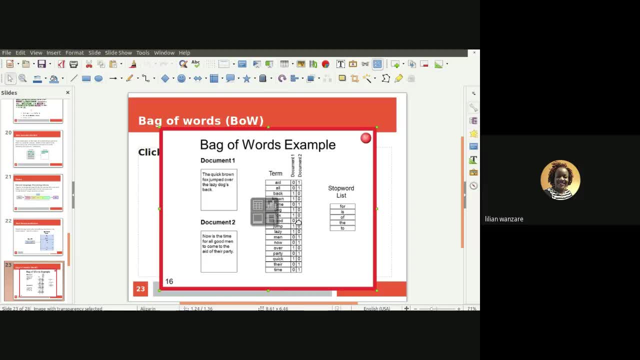 It is the simplest of document representations. Right now. there are more complex techniques that we use what we call embeddings, that are based on neural networks That really, really capture not just the presence of the word, but also captures on top of it. 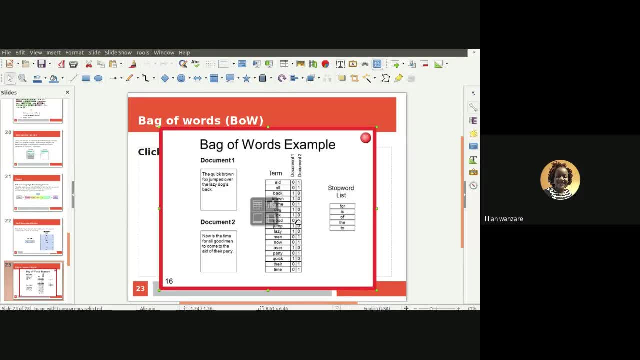 the meaning of the word. Okay, So maybe later on I can have a session later on about just what embeddings and vector representation in terms of complex techniques, not just bag of words. Okay, So there's a question, Okay. 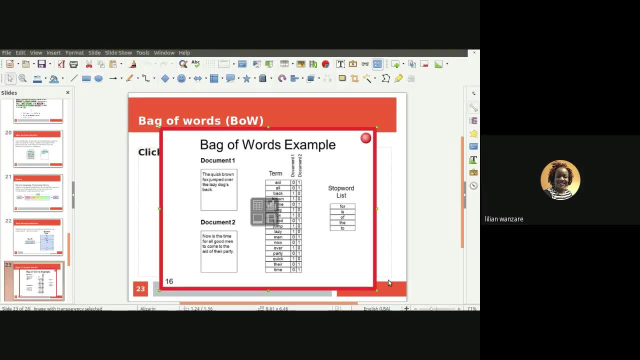 I'll answer that one also. Okay, So that is a bag of words. So really, you cannot perform any machine learning model on a text without representing the text numerically. Okay, That is number one thing you have to do. 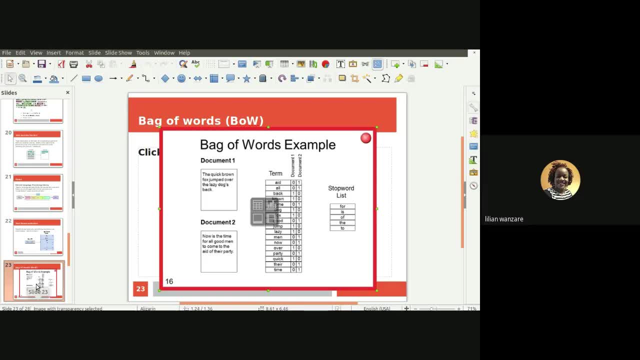 So let's assume, just picture in your mind that you know you're converting your document into a vector of numbers. It can be very complex numbers, but I don't know that it's just a vector of words, numbers. that now represents your document. 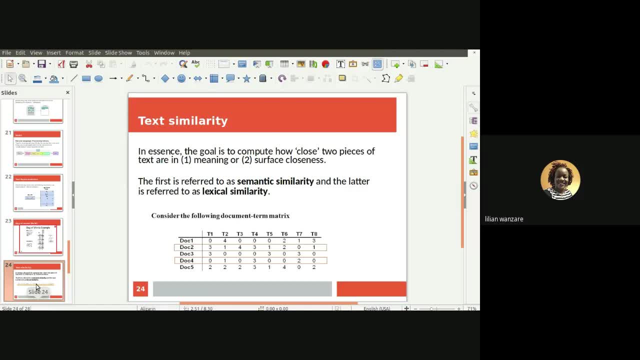 So now you have represented our document, So you might want to find out if documents are similar. Okay, You can just perform a maybe cosine or dot product similarity to see which documents are most similar to the other. Okay, So now every document has been submitted by just a series of numbers. 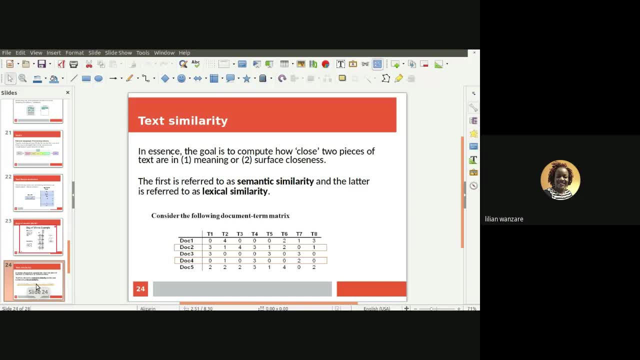 And you can just count how many overlaps are there in the words between documents. The more the overlaps, the more similar the words, the text. The less the overlaps, the more different or distinct the words, the text. Okay, So really, representation enable us to do textual similarity and cluster documents into. 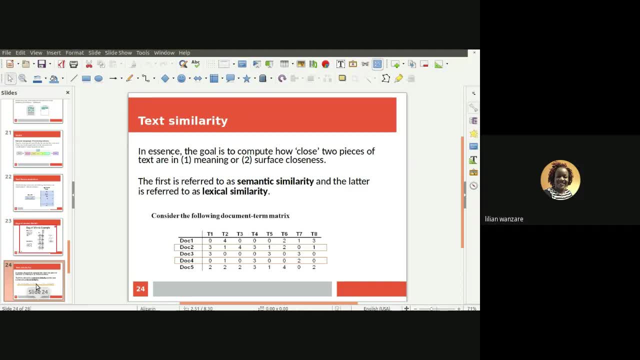 groups of documents that are similar, able to group them, because they will tend to have the same distribution of words if they are similar compared to the ones that are more different. Okay, So you can imagine if you have a document about sports, a document about restaurants, 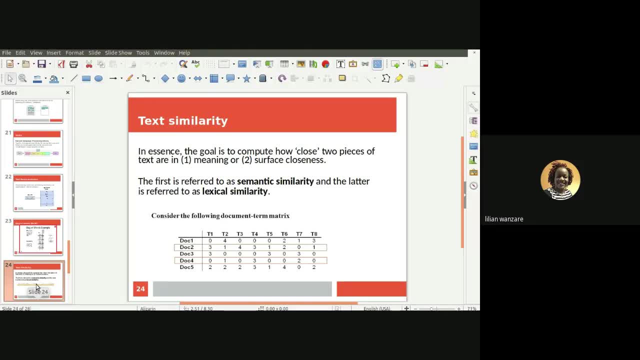 of course, their words will be different. About sports will be more words than sports words, so they'll be grouped together, And about restaurants will be more full-bladed words. So just by doing a simple bulk of words model, we're able to group similar documents together. 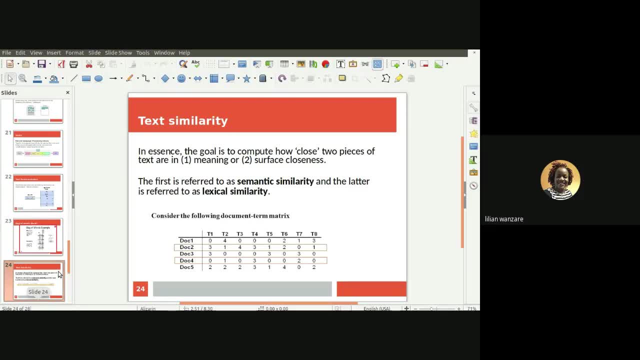 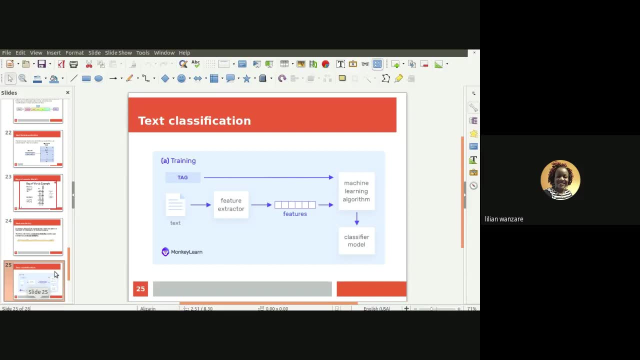 Okay, By using text representation. What I want to talk about is text classification Examples I gave before. Imagine the question somebody asked: You want to train a chatbot to ask specific questions and send feedback. Okay, The first thing you want to do is to be able to, because it's I'm not sure if you have. 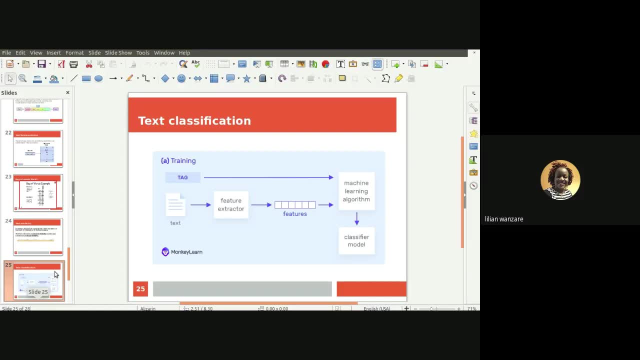 much in learning background. but let's say you want to train a text classification. One thing you need is the text itself. The second thing you need is the tag to that word. text Classification is a supervised task. That means you have to have both the text and the tag. 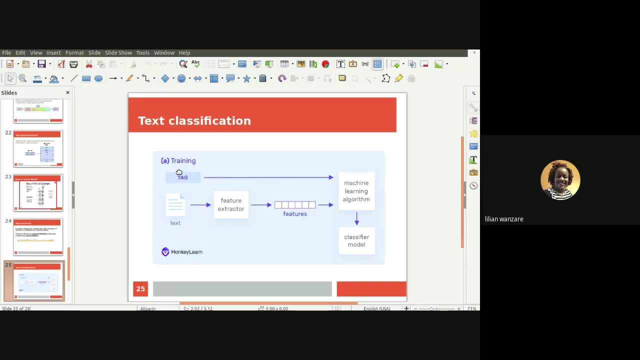 Then the model learns how to associate the text and the words with the tag. So, for instance, you want to train a model to be able to decide if something is a restaurant or it's a spot, So you give it many texts with the tag spot and many texts with the tag word restaurant. 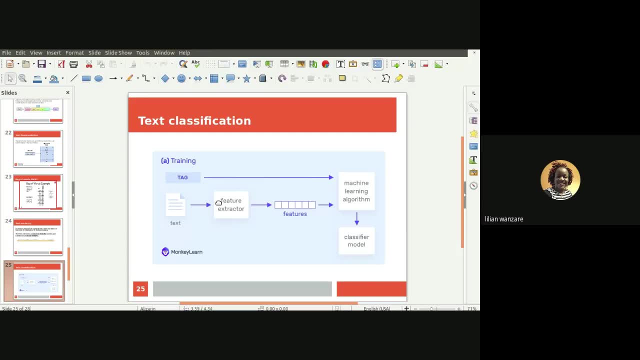 Okay, Then you do feature extraction on the document. Feature extraction just means you transform the document from just text to a vector of what Numbers? Once you have the vector of numbers, you use any machine learning algorithm for classification. I'm going to give you an example. 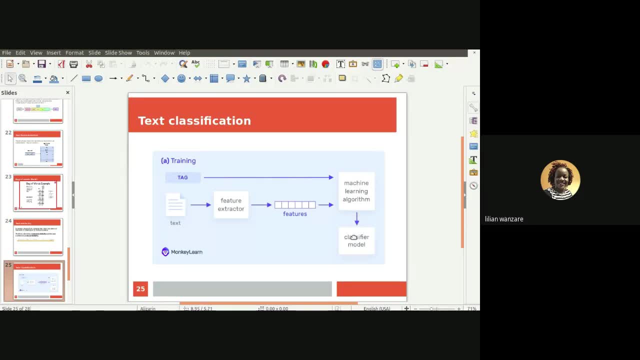 And then you have your classifier words model. So the basic thing is you have your text, which is tagged. You transform the text into features, which is just a vector representing the text. You plug your features and the tag in a machine learning model to help it associate which. 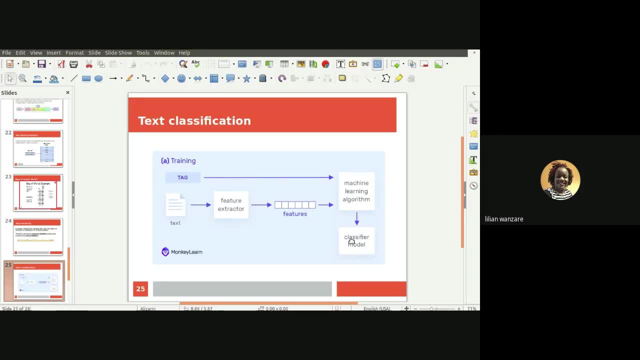 words belong to which tag, And then you build a model classifier. Now, once you have the model, what can you do now? If you have a new text that you don't know its class, okay, you again get the text perform. 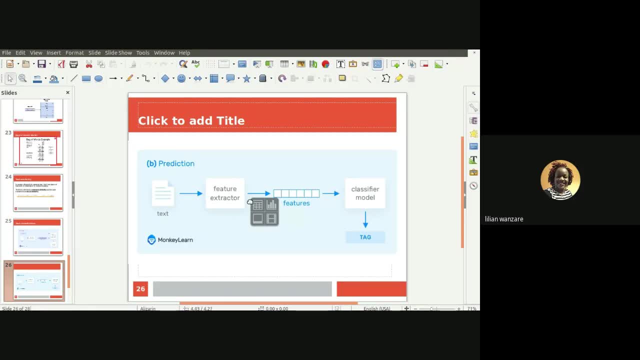 feature extraction, which is just transforming it into a vector, And then ask the model: okay, This text I've given you. what is its tag? The model gives you a. what A tag? For instance, you give it text X, the model. you ask the model: what is the tag of this? 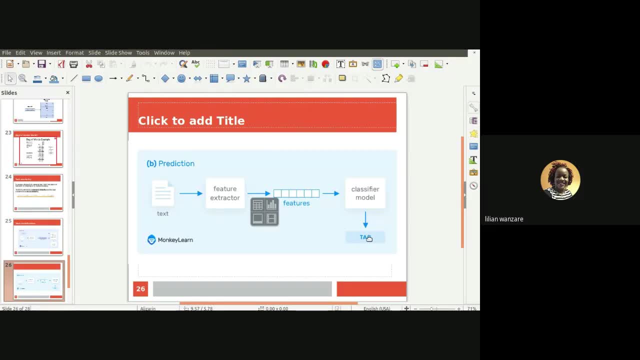 text And the model will say: is it either a sports text or a restaurant? what Text? Okay, So that really enables. you really have to have what is called the training data. The training data is for training your model, And then you have kind of the test data, what you want to test to see how good your. 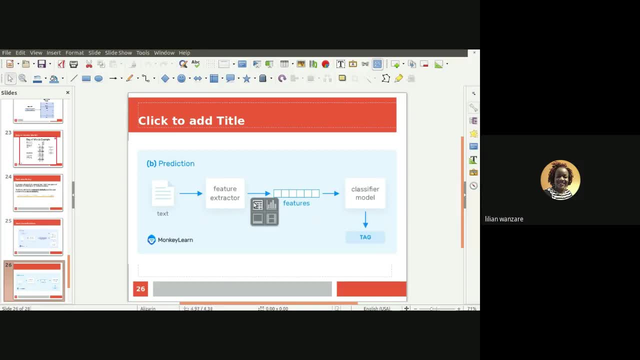 model works by asking it questions about the text And if it uses a what A tag, And you're able to test if the tag is correct or not. what Correct? Okay, That is how, more or less, it works. So this is a bit more complex than the previous set of examples. 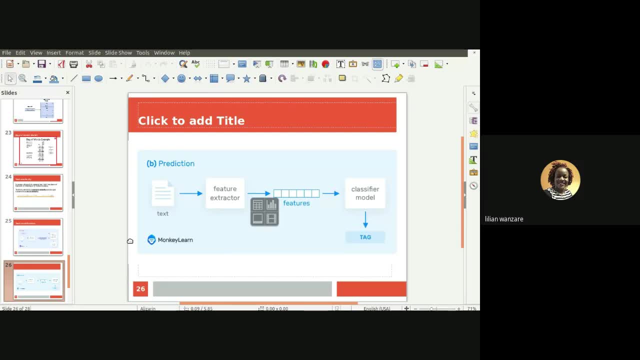 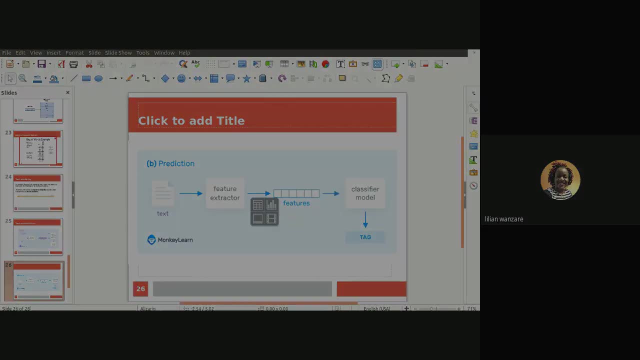 So there's no question, I can go to the notebook And then we go through the assembly- Okay, And then we go through a simple text specification example. if there is no question, so far, Good. So in your mind, just think about what we talked about. 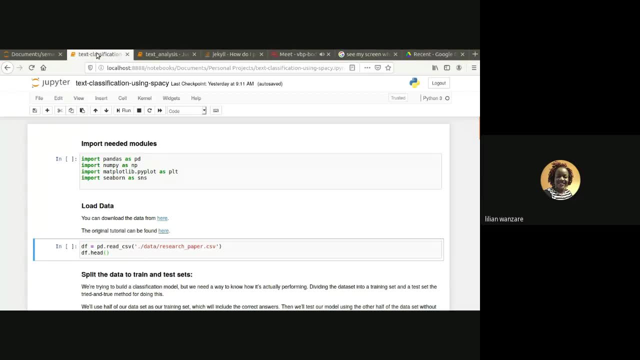 If you want to classify a document, you have to have the document and the tags for that document. You take the two. You extract the features, which is that transforming the document from a text to a vector. You plug the features into a model that learns to associate the features of a particular 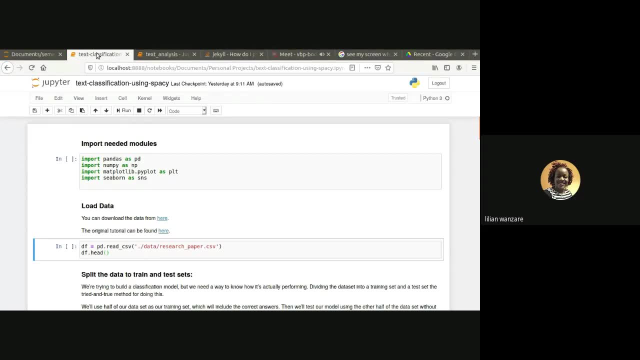 tag And then you build a model. Once you have your model, you can ask your model questions. You provide a given text, You ask the model, what is this text about? And it gives you a what A tag. Okay, 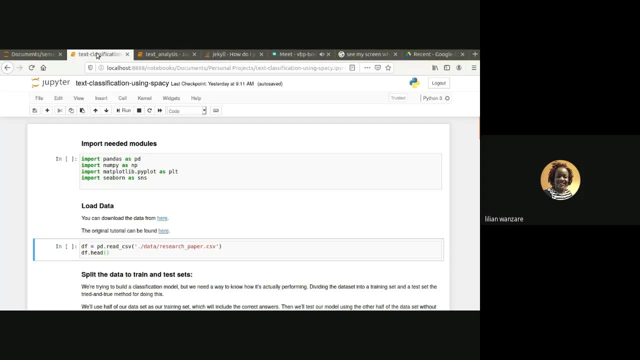 That is more or less, in really short, what we mean by classification. So here we want to classify some research papers. Okay, So you know that there are many research publications, journals. Okay, So you want to know. if you have a text, can you know which journal it belongs to? 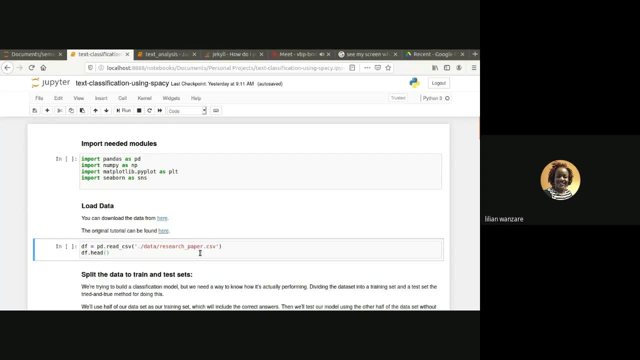 So the data is here, Okay, So let me show you on that. So first I import pandas. I hope pandas is just enabling us to process CSV kind of files. The NAMP enables us to do some numeric calculations. 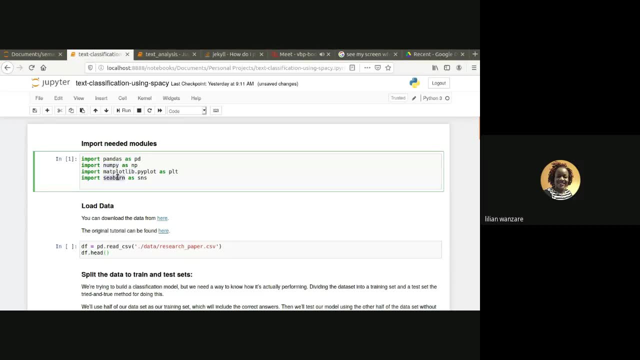 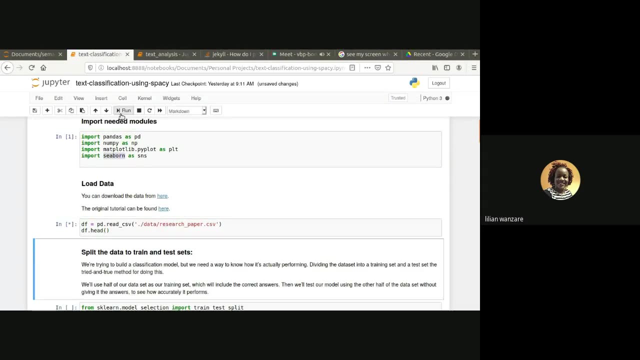 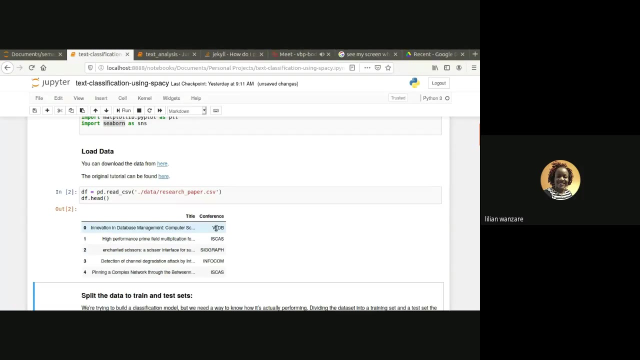 Matplotlib and Seaborn are for plotting, Okay, But once you can learn time, Okay. So let us look at this data. So you look at this data. This is the text, So this text belongs to this conference. 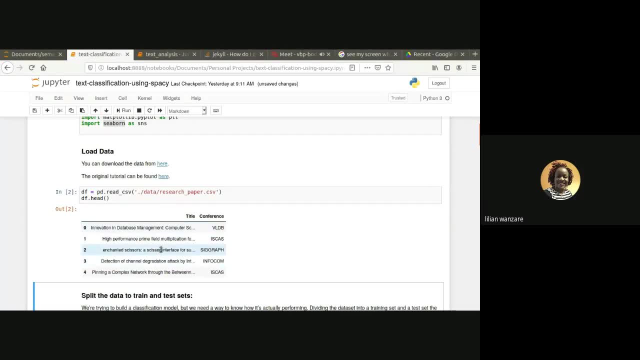 This text: another conference. Okay, So you can see from our representation: you have the text and then you have the word tag. The title is the text, The tag is the word conference. So you have those two, Okay. 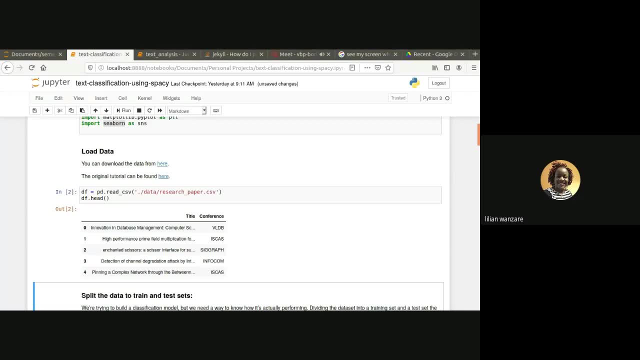 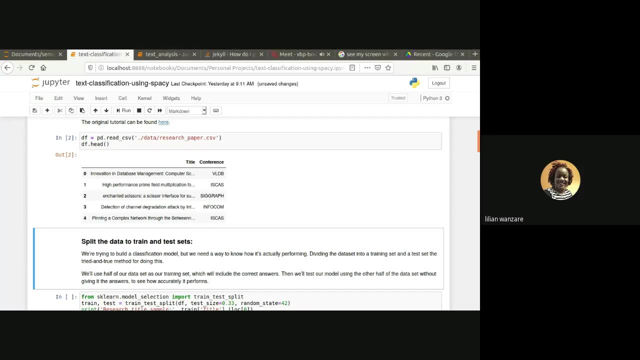 So we have our title, We have our text. That means we have our text, We have our tag. The first thing we want to do is we want to be able to split this data into what we are going to use to train our model and then what we are going to use to test our model. 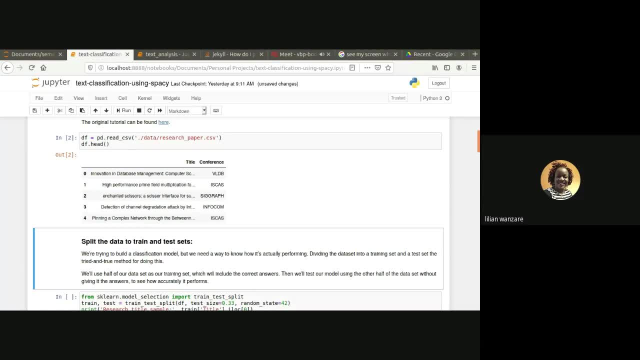 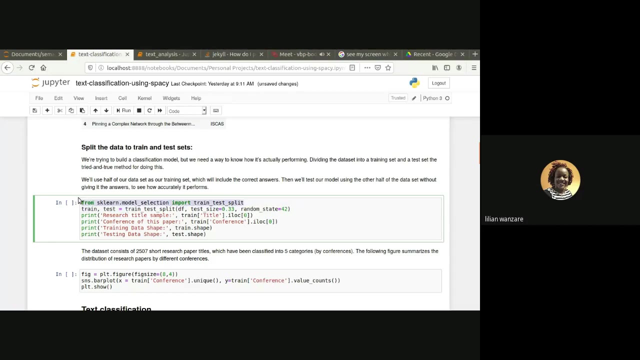 Okay. So when you are trying to build a classification model, we have to really know how our model performs. That is why we divide it into training test and testing test. Okay, That's it. There is Skit-Learn. Skit-Learn is also a tool kit, if you want to call it, that enables you to perform machine. 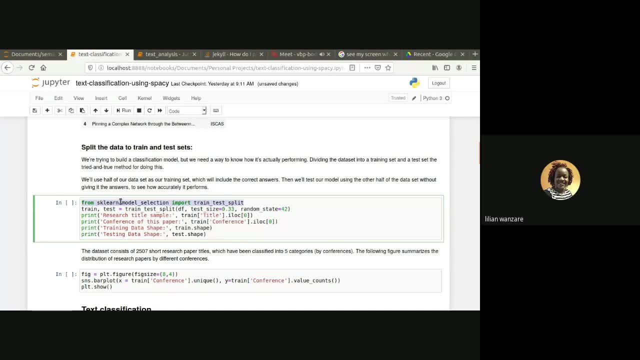 learning, So it's called SkLearn. SkLearn contains many machine learning models, from classification to clustering to dimensionality reduction to whatever kind of models that are existing in Skit-Learn, And they are not just used for NLP, They are used for mean data science and all the other you know, image recognition, all. 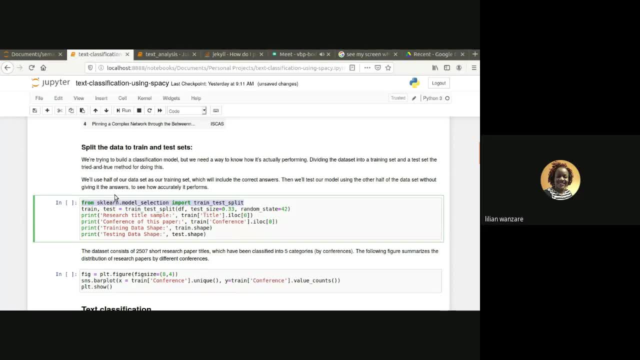 the other fancy, fancy stuff out there. You are able to do them from Skit-Learn. If you are into machine learning, you can try and check out Skit-Learn. So it has a function called train test split. So I am just splitting my data: 0.33%. 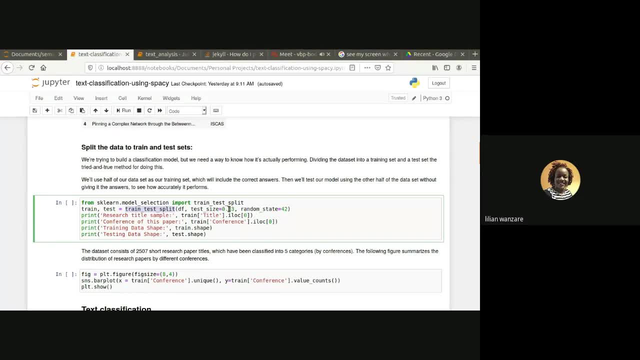 That means 70% of it I use it for training. Another 30% I use it for testing. Okay, Okay. So if I run this, you see that it contains around almost 3,000-ish documents. I have reduced it to just a training set- around 1,600 of them. 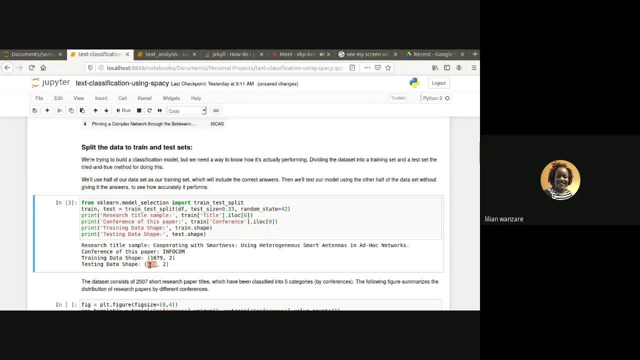 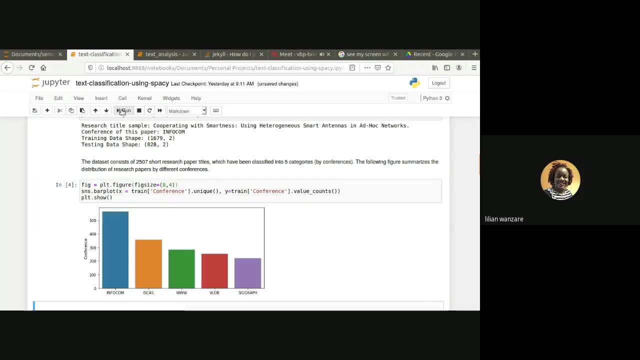 And for the test I use around 800 of them. Okay, And the company is called EFCO. Let me just show you that in a picture that is faster. Here are the number of documents in that text. Okay, So, EFCOM, you have around 500 or so. 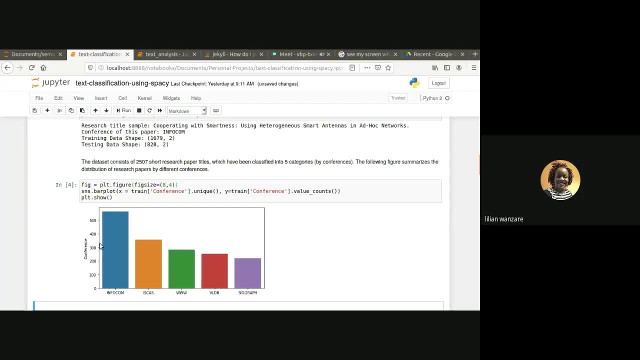 Another one. you have 300. So every text belongs to one of these categories, one of these conferences. So you want to build a model that is able to predict if a text belongs to which conference. Okay, In a nutshell, 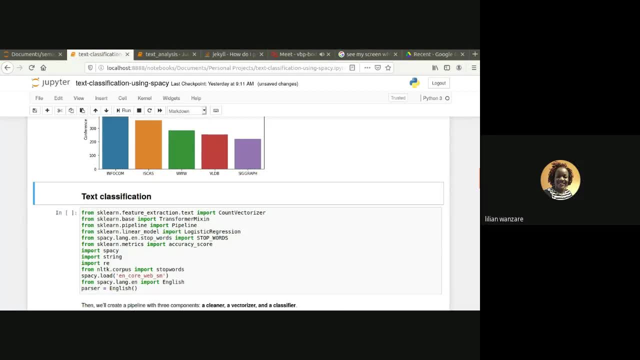 Let us start the training process. Like we said, I will import many things. You will not learn them today, but just to kind of entice you to learn them more, The first thing you want to do- let me start from the non-text- is this part here: 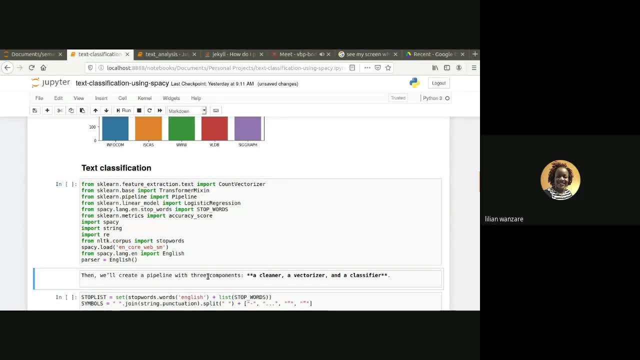 You want to clean your text, You want to vectorize your text, Then you want to do what? Train your classifier. So cleaning the text here means you perform NLP on the text. You remove stop words, you tokenize, you lemmatize, you sentence split, whatever is necessary. 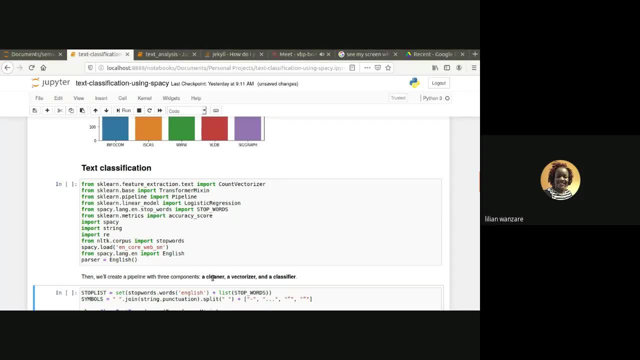 That is part of the cleaning. Once you clean it, you vectorize. Vectorize means you transform it into a what, A vector representation of your what. Once you have your vector, the next thing to do is to be able to do what? 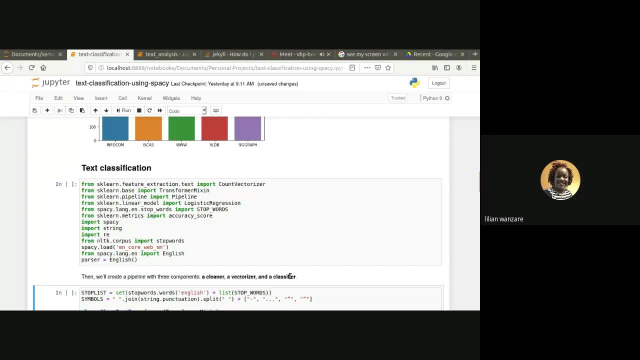 To classify. Now, there are many tools outside there, but I have stuck to either Skitlan or Spasi for this example. Like I said, Skitlan has many, many machine learning techniques. One of them is called feature extraction. 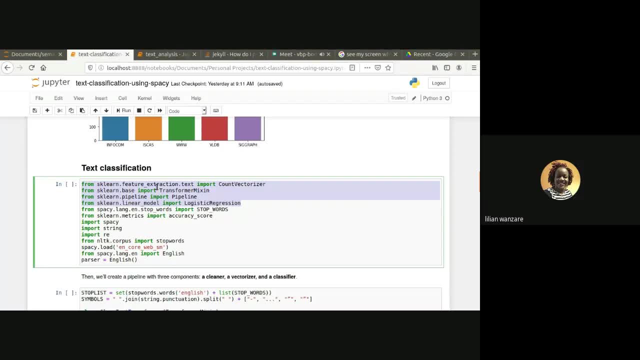 There are many feature extractions. The simplest one is the bag of words. The bag of words is called a count vectorizer. It just counts the number of words in the document and says it's there or not. Okay, It enables us to transform it into a particular vectorization technique by transforming the text. 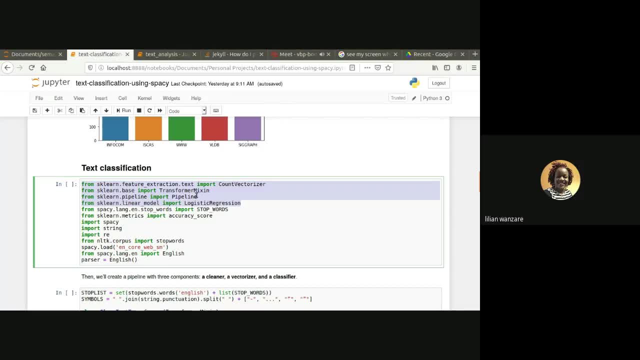 It's almost to build a pipeline. You don't need to worry about them so much. And then I've chosen a linear model called logistic regression that helps in classification. You can choose any other model that you so wish: Support vector machines, if you want, or just a kind of division trees. 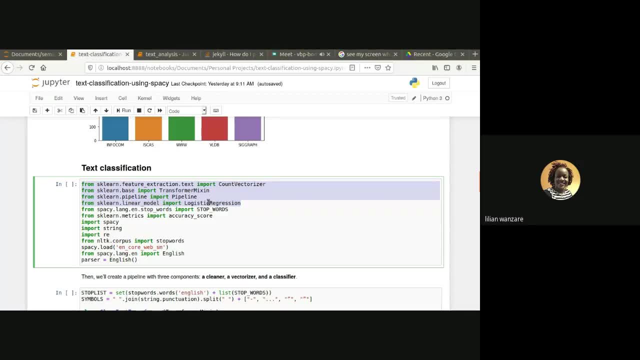 There are many models that exist, But it's one of the simpler models. Okay, Good, So again we do the same. We load this. We load our NETK. We load our data. We are working on English text. We load our stock words. 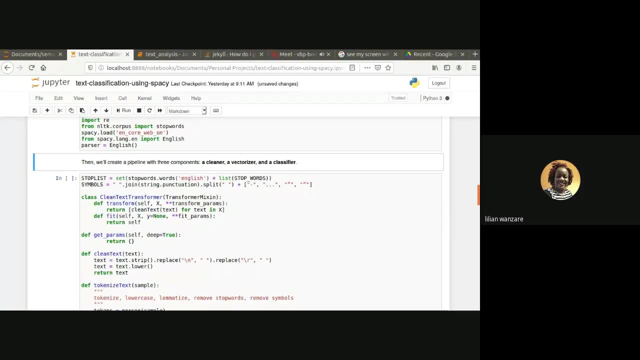 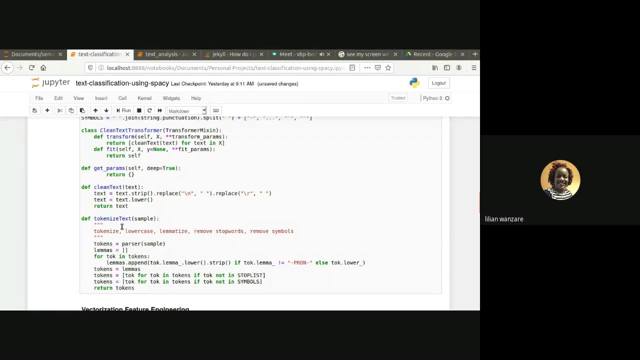 And you want to use them. I won't worry so much about the second code. What it only does is it kind of cleans the text by doing tokenization, It transforms the text by doing vectorization And then the fit is it classifies. it builds the classifier by the fit method. 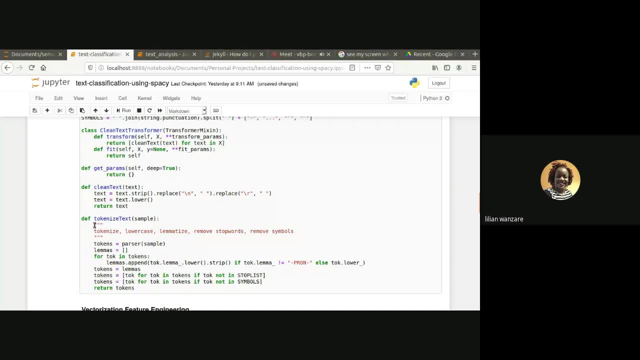 Okay, In a nutshell. So first we clean the text. Clean the text means we are just removing unnecessary new lines, We are lemmatizing. We are removing the stopwatch, We are removing the stopwatch list, We are removing the symbols. 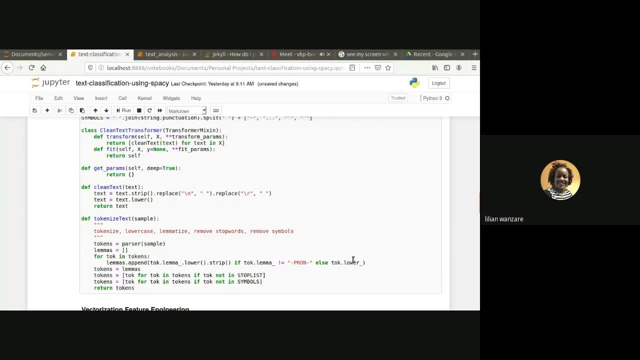 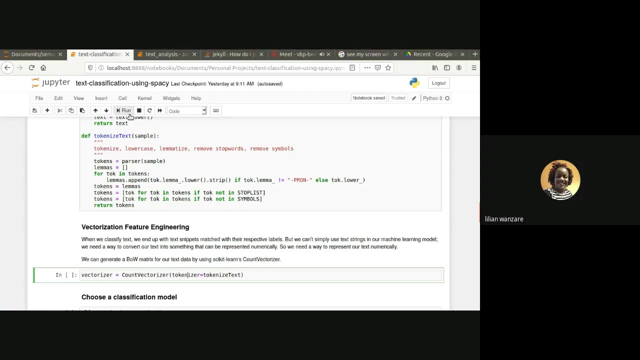 Okay, We are taking it to lower case. That's what we mean by cleaning up the text. Once you clean up the text, we transform it into our vectorizer And then we fit it to our model. Okay, So let's build our vectorizer first. 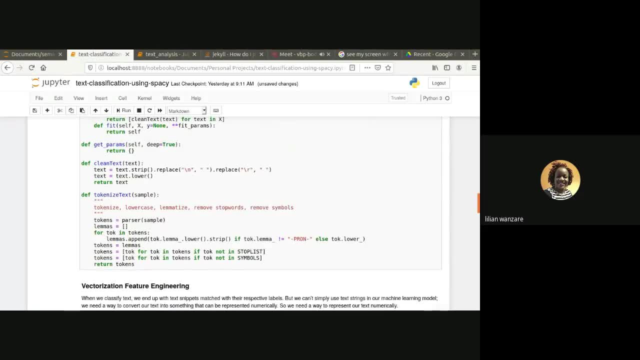 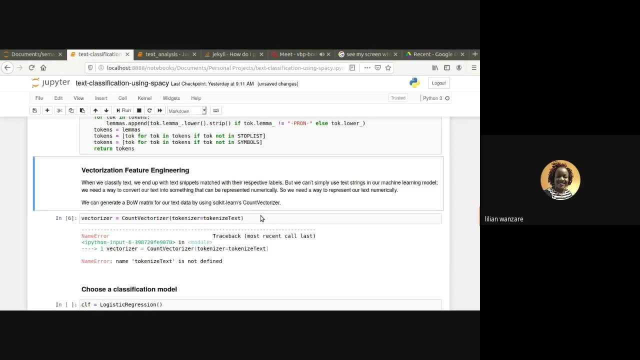 I've not loaded it. I have to load it here first And this one first. Okay, And we can now load our vectorizer. Okay, So vectorizer is just this count, vectorizer- Okay, The vectorizer is text input, the tokenized text. 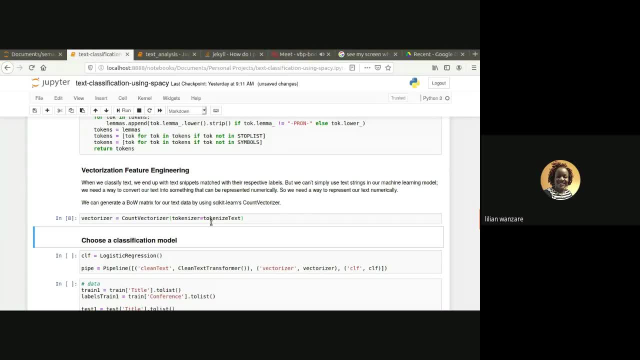 Okay That you have defined up here The tokenized text, And then our classifier is just a little derivation model. When you call our pipeline, what we do is we clean the text first, We vectorize it And then we classify it. 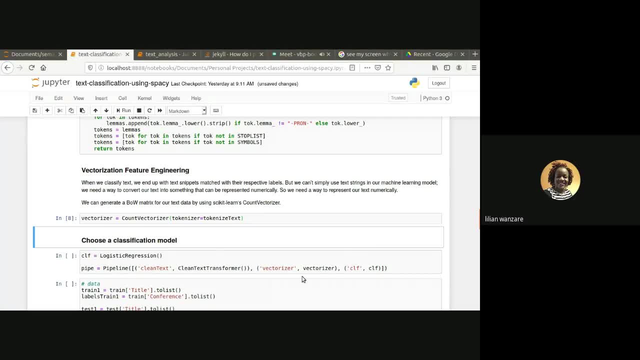 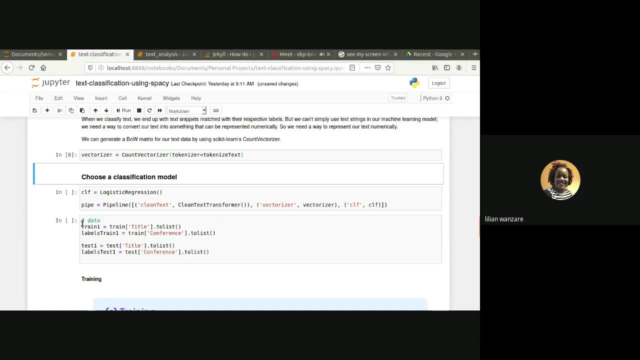 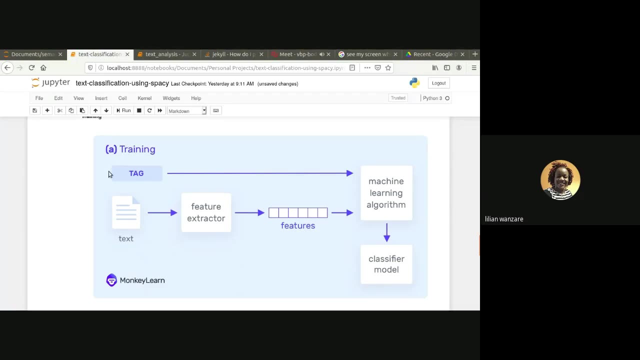 The same procedure: Clean text, Vectorize it, Classify the text. Okay, And we already split the text into training set and test set. So, if you remember, from our diagram, before you have the text, You have the tag, You extract features, which is the vectorization. 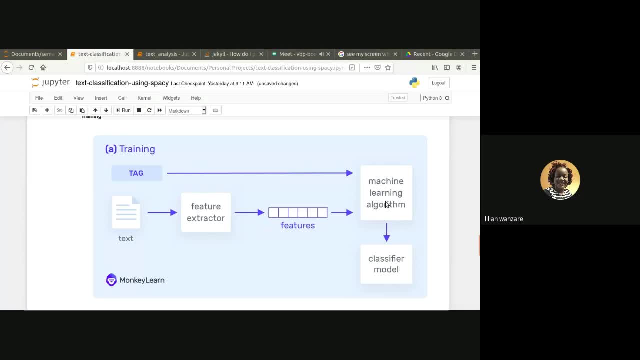 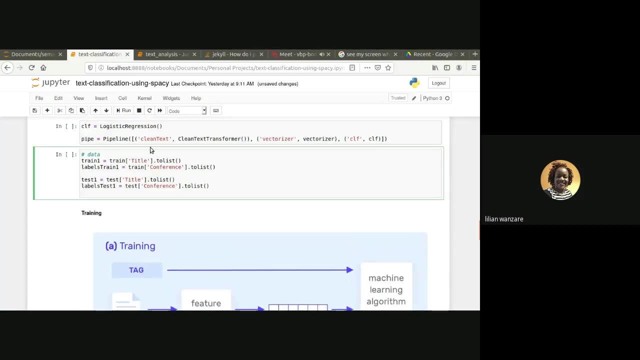 You put both of them into a machine learning model. You get your words: classifier- Okay, It's the same high level idea of it. Okay, Pipefit is what calls the classifier. I have to run this too fast, So I load the classifier. 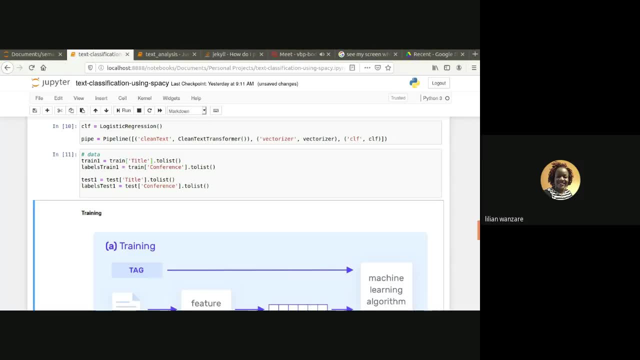 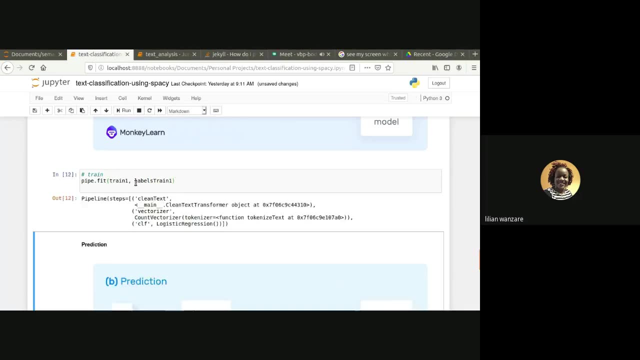 Then I load the data, Then I perform classification. So what a classification does is just: it takes our training data, which is the train, It takes the tag. Okay, It combines those two. it combines those two, which is just here: the training data and the tag. okay, 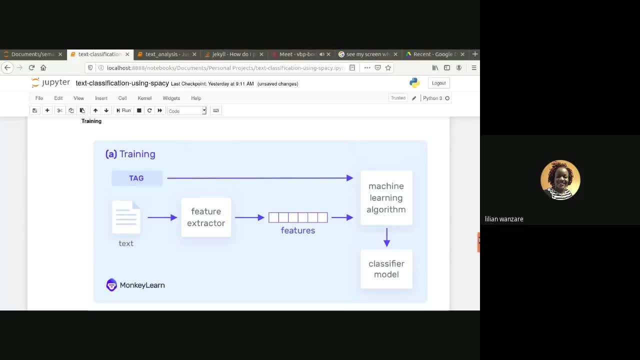 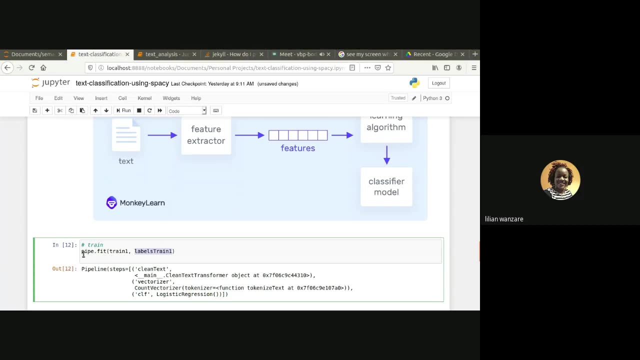 it takes, goes to and builds a model. what i've done here: i've taken the training data and the labels or the tags i put past that to my fit classifier. so what this does is it just trains a model and is able to learn to distinguish different um conferences. 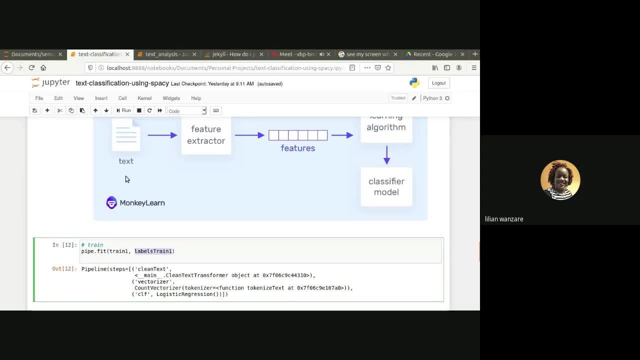 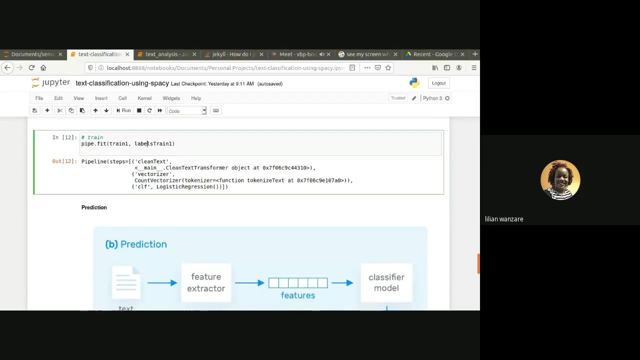 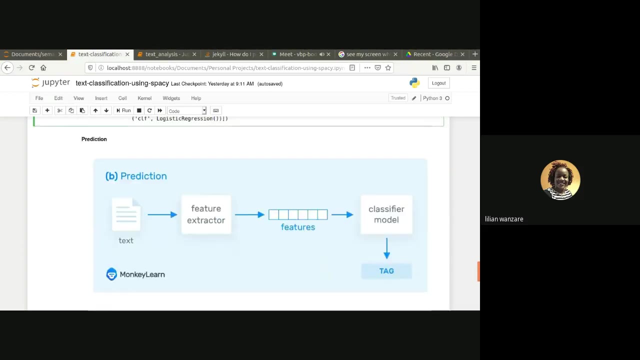 from each other. okay, just takes the text and then the tab. only those two. now, once you have the model. now this is our model. okay, now we have our model. what i want to do next is we check the, we take the testing data, extract features. we ask: our model gives the water attack? okay, but what we have, 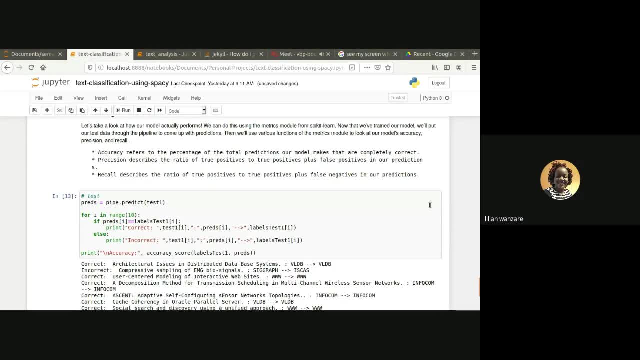 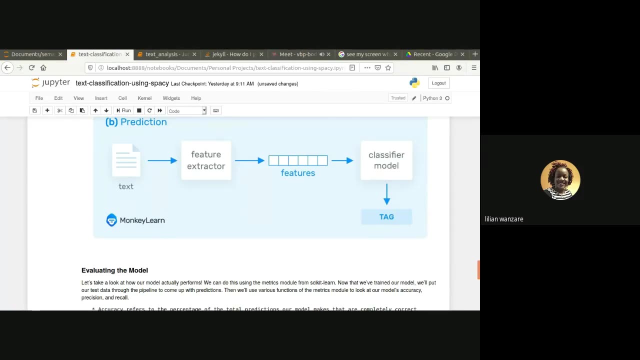 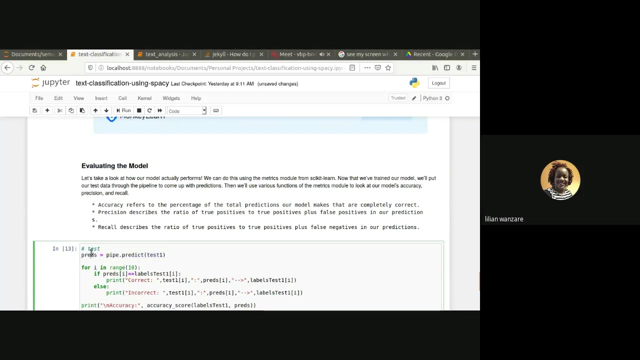 here. we just run that. this part. pipe predict test is what we have just explained in this diagram. you take the text, you pass in the model. it gives you prediction. okay, what we have here. we have the test data, we pass through the model. it gives us water predictions. then i look at the predictions. one: 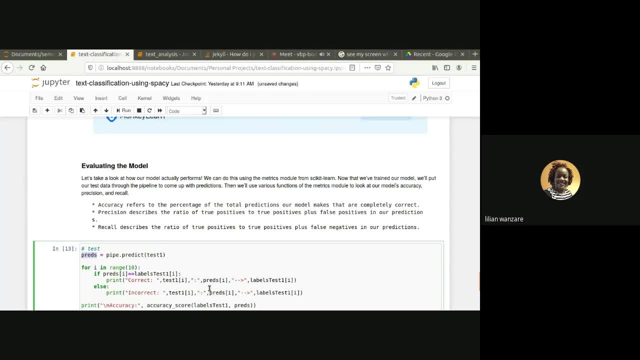 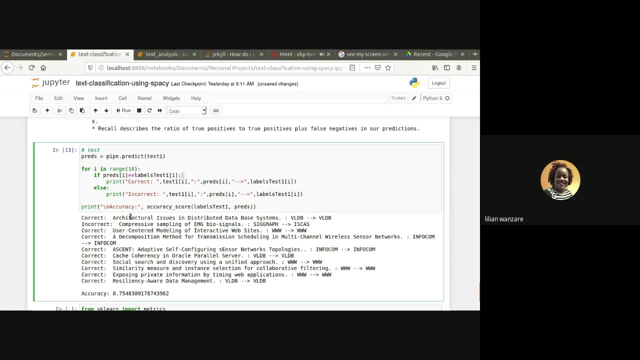 at a time, okay, if that prediction is the same as the prediction that we just made the original label, okay, that is correct. if the prediction is not the same, that is what incorrect, and then i just count how accurate is my system. so the example is here, like in the first one. 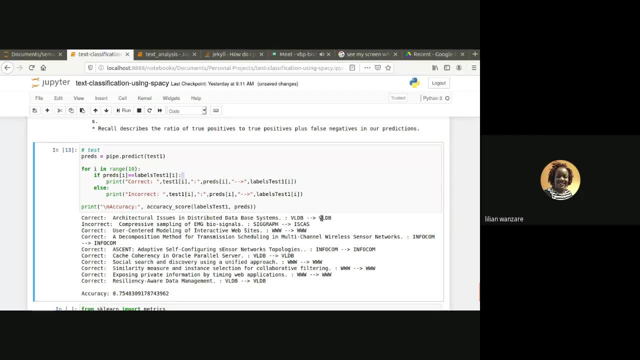 the system predicted that it is a vldb, which is water similar to the correct water level. in the second data, the system predicted this sg graph, but in truth the real label for it is what it is and it's what's incorrect. so you just go through all your predictions and count which are: 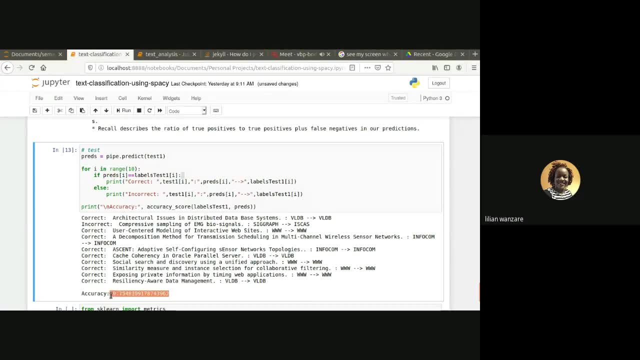 correct, and then our system is 25 percent water accurate. okay, so we have come from building the model and then using the model to make predictions on our tests data, and then we compare the predictions that are made by the system against the actual labels or the actual tag of our text. 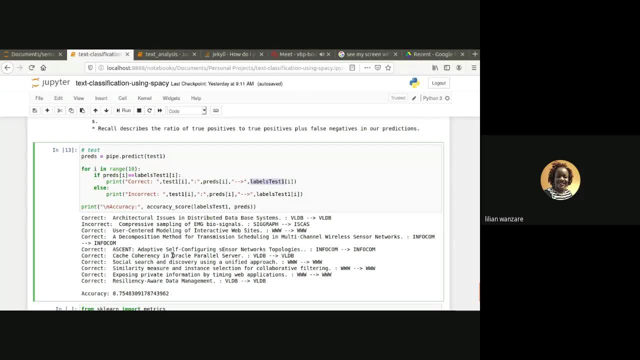 that enables us to estimate how accurate or how good your system is. okay, as you can see, our system is not good. it's not so good. what can we do? we can go back and reprocess the text and try different techniques. instead of using a simple count vectorizer, you can use a more complex. 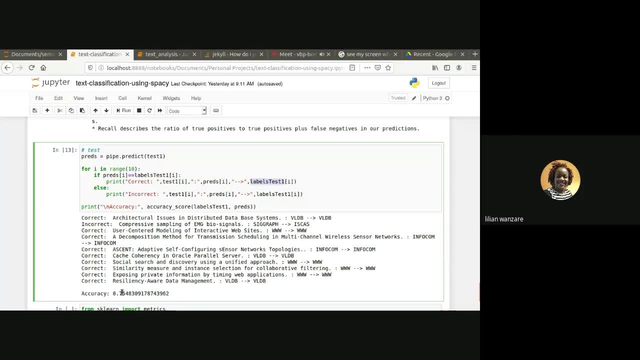 representation, for instance. yeah, you can add more data you can. you know, there are many things you can be able to do to to improve your, your, your model water晶 Your, your model words. That is just in a nutshell. I are able to kind of take your text, okay. 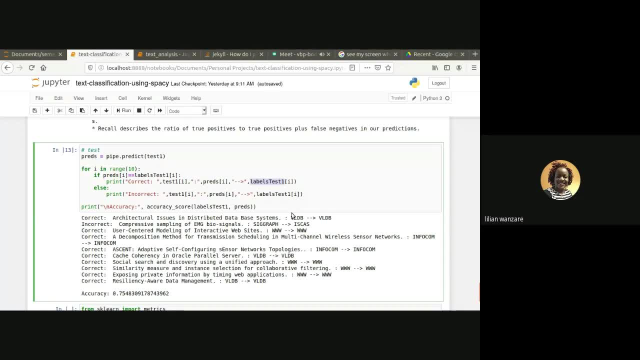 transform it into a vector Representation, use that vector in a model to build a classification model and then use your model to predict. Now, once you have this model that someone asked, you just need to build an interface to expose your model on the Internet So that someone can come and ask a model a question. then it gives a water an answer. 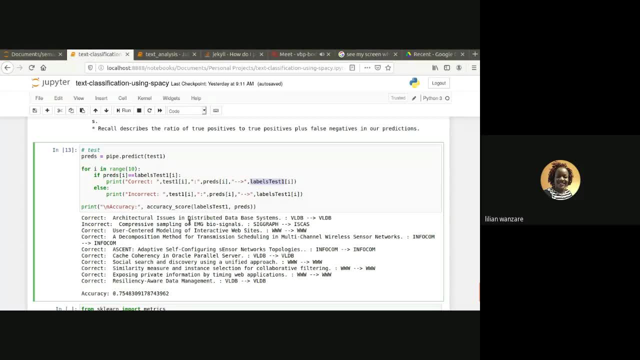 But the training part is normal offline. once you've built a model, you expose your model out to for others. That's the the. the one choosing a model really don't care of the model works. They just want to give the question and they get the water the answer. 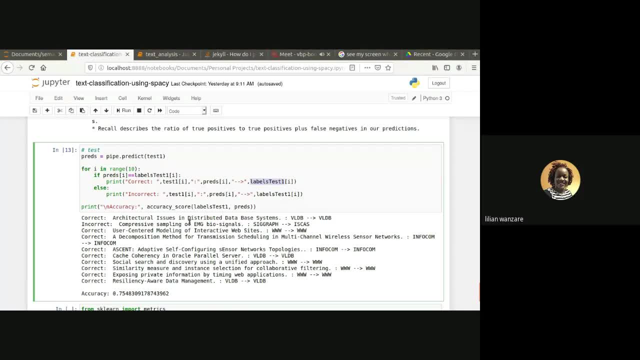 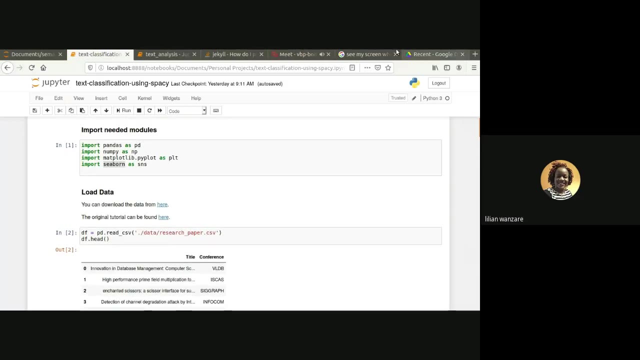 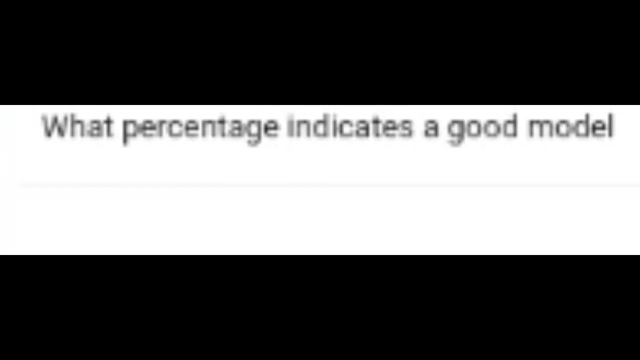 the techniques of exposing your model to be used in the public by by By others. okay, before I wind up questions fast, You have been rather intense, but we have time to discuss and ask any from any part. Yes, there's a question from. There's nothing as Vegas, good. 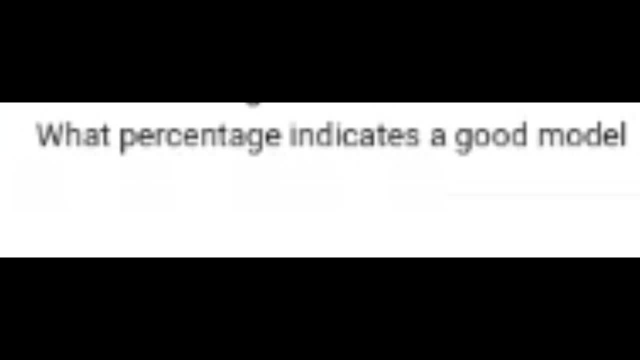 The reason I'm saying that is it depends- This is really a theoretical answer- faster If I got the real answer. it depends on How good the humans are in that task. okay, that's on the theoretic perspective. for instance, Yeah, if I am trying to build a system that is able to. 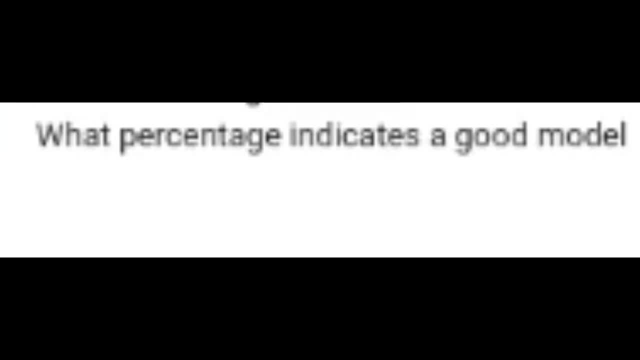 correctly determine. Like: what type of document is this? Okay, and human beings find it very, very difficult for humans to distinguish. Yeah, if you have what is called the human upper bound. okay, if the human Perform like a 70%, your system performs that. let the 65, that is a very good system. 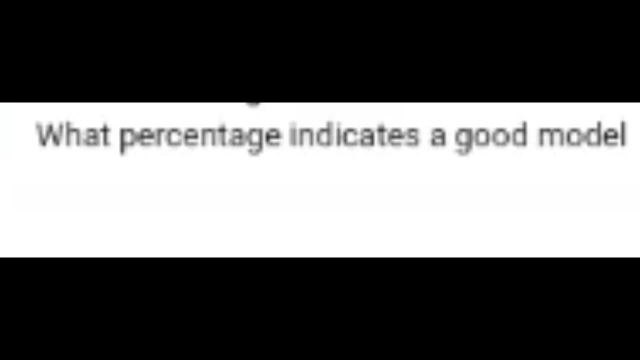 But if it's a very simple task, You must get 100%. a system that six, That's a very bad water, sister, Okay. and then it needs to get more than 90%. Yeah, there's always something called the human upper bound that determines how good I want. What are they like? the theoretical aspect of it now? 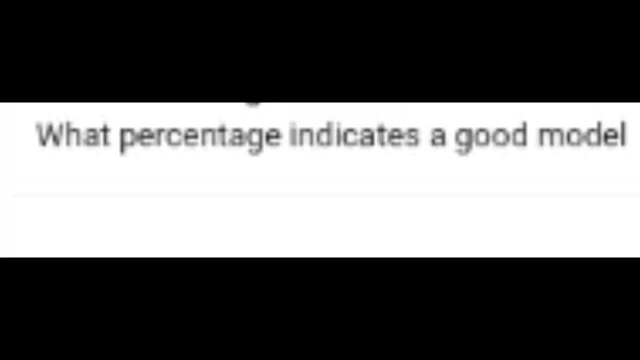 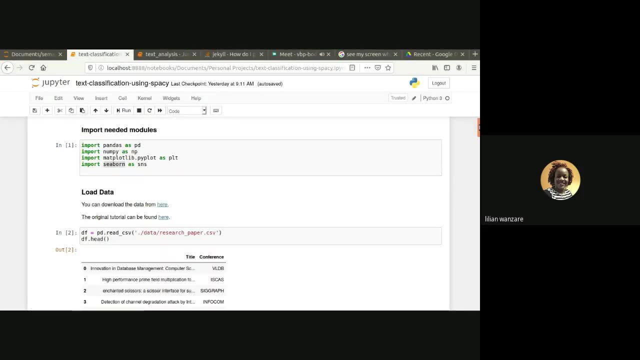 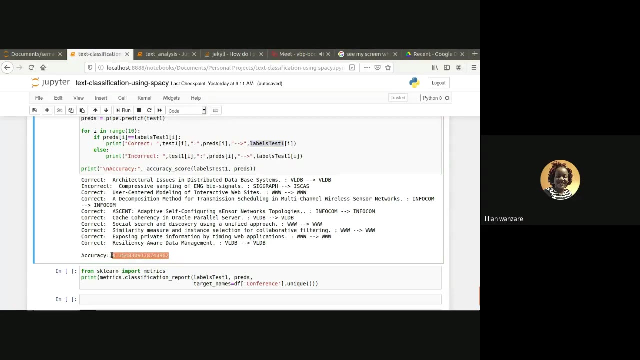 If you come to set an example, for instance, They are. There are many techniques of measuring how good a system is, So what I have shown you is just Classification, is just accuracy. I think this is the simplest model that says: just count for me how many times something is correct or not. water correct. 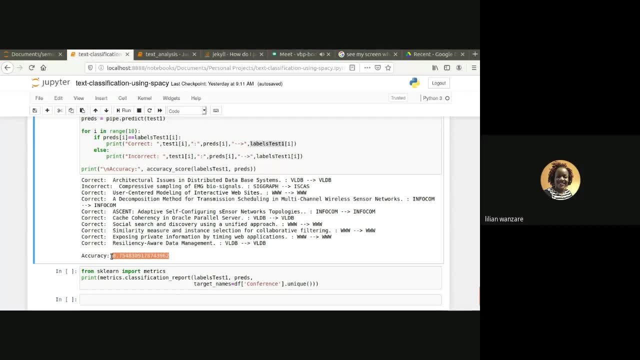 accuracy tends to be biased, depending on the Distribution of the number of items in the classes. of course it was with the majority, Okay. So you can imagine: if you have a system that is supposed to predict if somebody has Cancer or no cancer, Okay, and in your data set you have like, like in the real world, 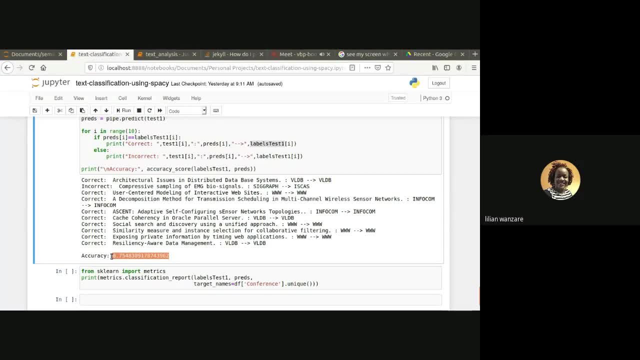 You have like around 90 million people but only 1 million have water, answer Yes, and then 90% don't have, but 10% have. if your system always, always just say: don't have what have, what have. if you 90% water, 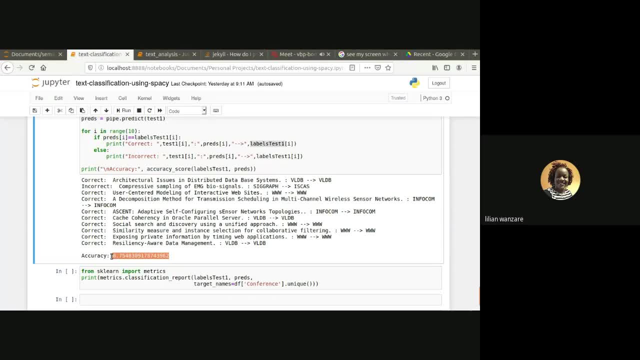 Correct. Is it a good system? You know, because there the issue is, it is more important to get those Who have than to say it's it's. it's worse to say someone does not have cancer there, They have water cancer. So for that system it is important to get this 10% water correct. 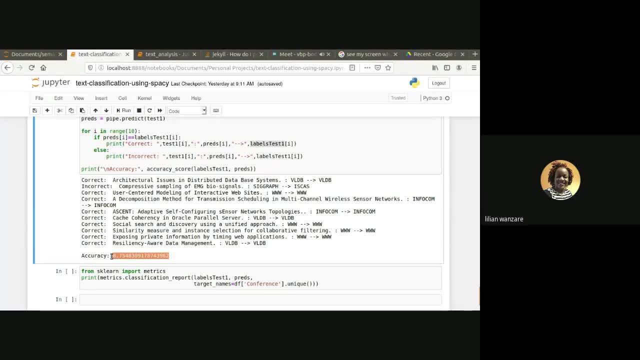 Okay. so really, the issue of goodness of a system always depends on what is your target problem. So in that case the system is 90% correct by just guessing it will doesn't have, but it's just guessing. It is more important that it gets exactly. who has the water, the cancer for it. 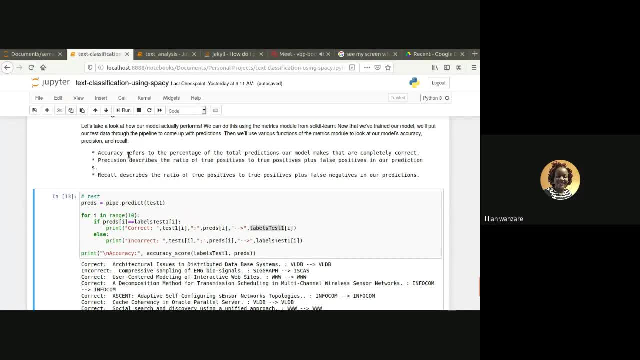 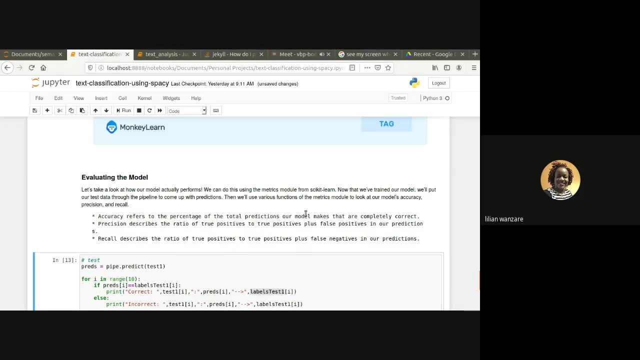 the Other techniques that you have. one of them is accuracy. So accuracy just measures the percentage of total predictions our model make that are completely water accurate. But then this is of precision and recall. Okay, now precision is this: I Stick with the cancer, but it's easy to explain it like that. 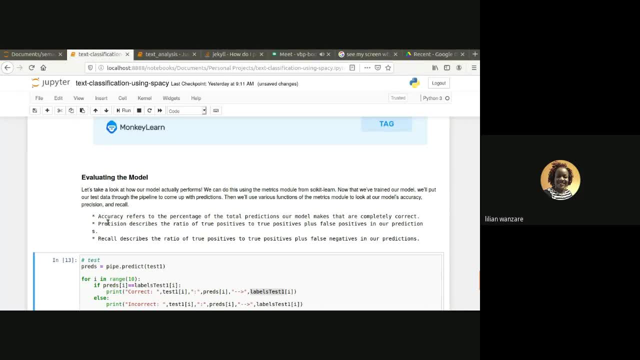 if, out of all those cases That your system have said to have a cancer, Okay, how many of them actually have water cancer? Are they how precise your system is? if your system says 10 people have cancer, after those 10 people, how of them actually have water? 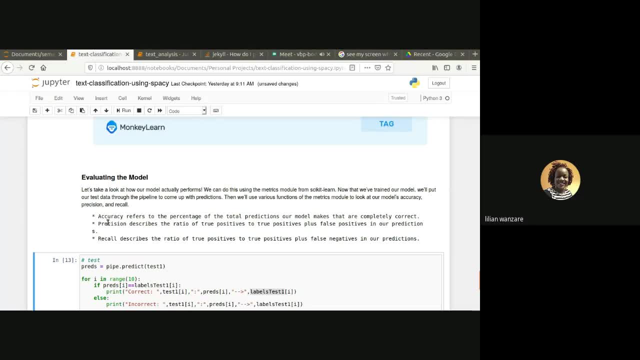 So if 10 out of 100 up your system, I've said, cannot have a hundred have cancer, out of those 10, eight of them truly Have comes the system. How precise is it? Okay, is eight over there number of people that have cancer? Then, aspect is recall: 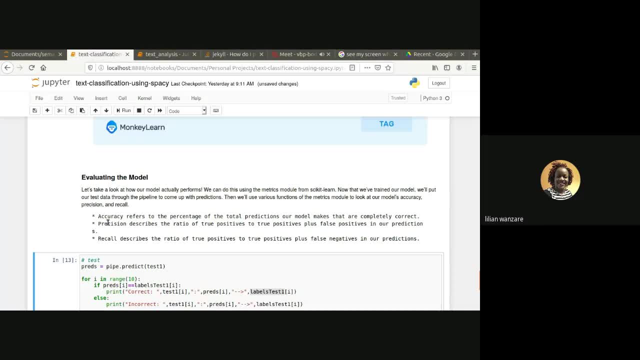 Recall is this: Out of all the people who have cancer in the letter says how many of them your system actually said they have, what Council we can notice in the difference? Okay, So recall measure is: is your system able to capture all classes correctly? Out of everybody who has cancer, how many of your system actually say they have water? 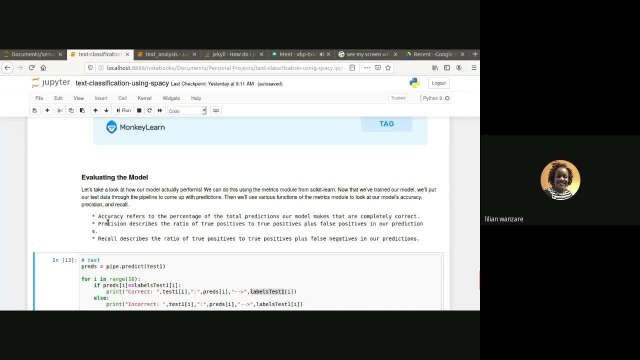 That is recall. position means, out of all those people the system said they have Cancer, how many of them truly have water? If you combine precision and recall, it kind of tells you how good your system is. It's always a better measure, and that's using what's accuracy. 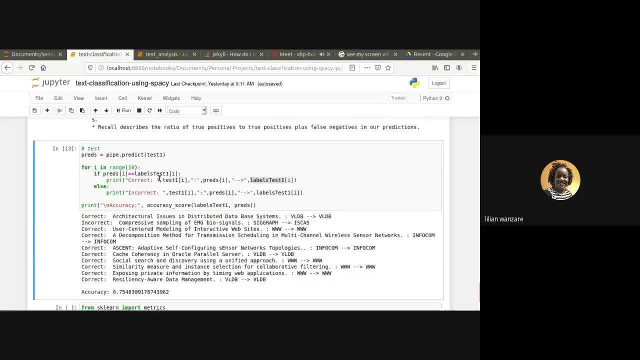 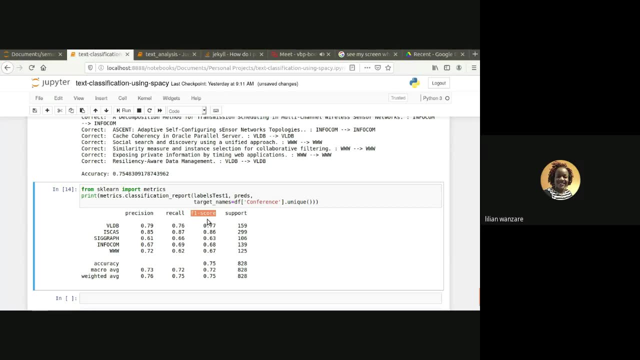 say, combining Mission and recalls gives you a measure called f-square. So if I run this part it's something called F1 score. F1 score: you can see that it kind of gets for every class. So that means if your system was just guessing. 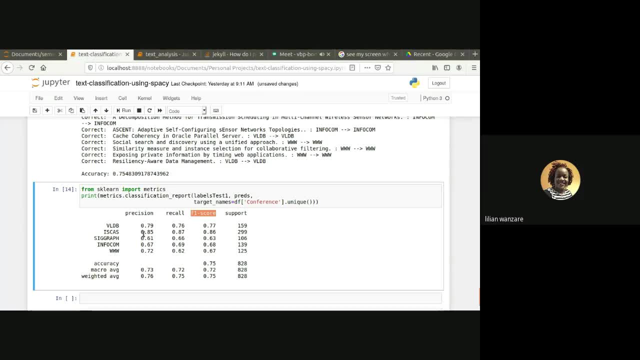 the accuracy will be high, but the precision and recall will be low because it's calculating for every particular class data set. How good is it in knowing that VLDB is different from ICAS? You can see that it performs very well with ICAS. 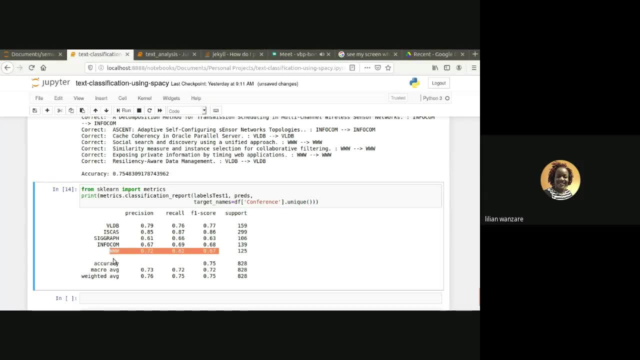 It performs well in what WWW data set. From this it enables you to see for every class how good your system is. It's better than just saying accuracy in general in a nutshell. So really that is the two main ways you can be able to tell if your system is okay or not. 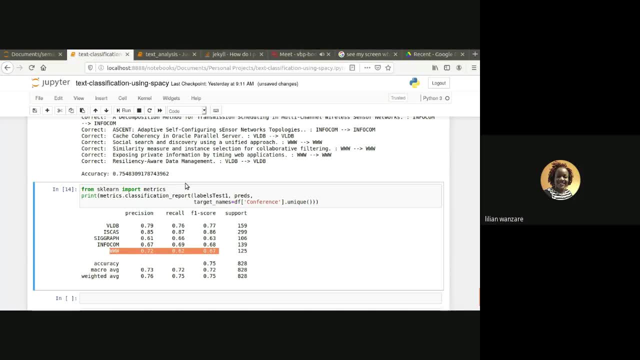 Theoretically think of upper bound. How is the humans one And only the problem domain? What is more important for you in your system That determines how good the measure of goodness of your system Someone else? I hope that more or less makes sense. 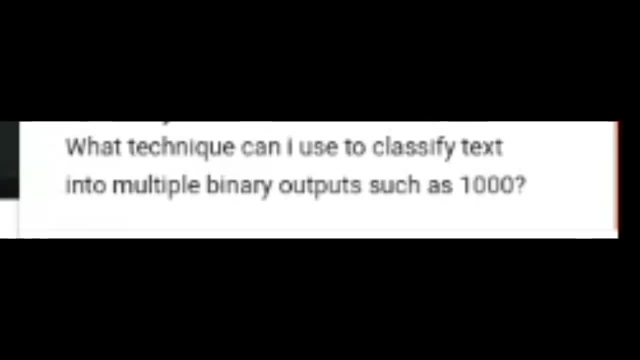 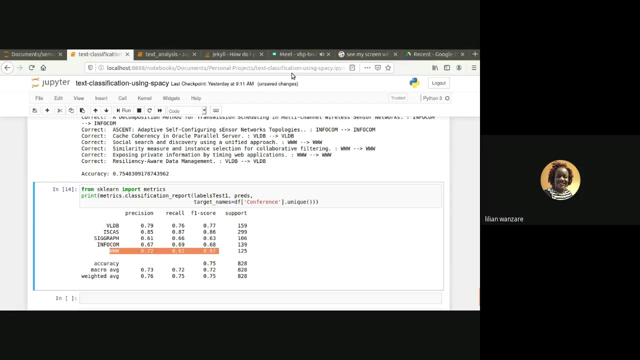 Yeah, there's another question from Juma. What technique can I use to classify into multiple binary outputs such as 1000?? Okay, Okay, When you say multiple binary outputs such as 1000, what exactly do you? I'm not sure I get your question. 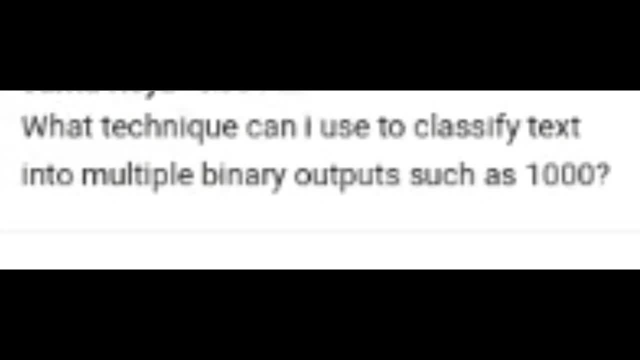 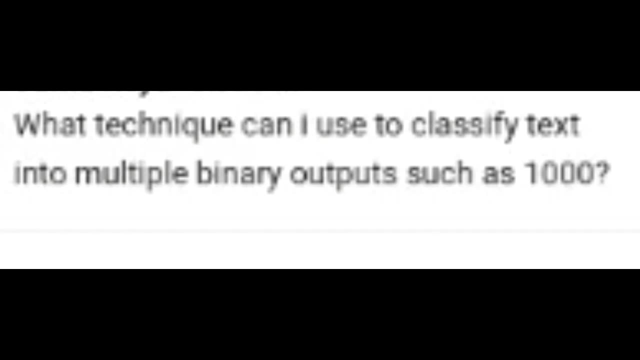 I was referring to a case where you have multiple, the outputs are labeled or the tags are labeled, such as maybe cancer. In case you have multiple labels, such as maybe cancer, you can talk of maybe cancer, diabetes, such like you can, not just 1000. 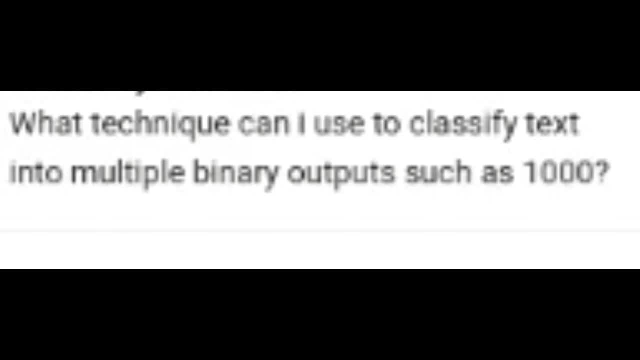 Yes, But one. In case it is present, then it's a one, If it is not present, it's a 00. Such like binary output. Okay, I get you. Okay, So you are asking a kind of a multi-label situation. 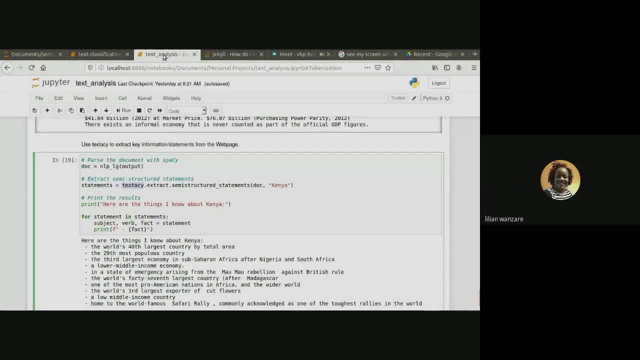 Okay. So, for instance, if I have a text, it is very okay for the text to be like, for instance, your classified emails: Okay, An email can be. it is not spam. Okay, The same email is a work email. 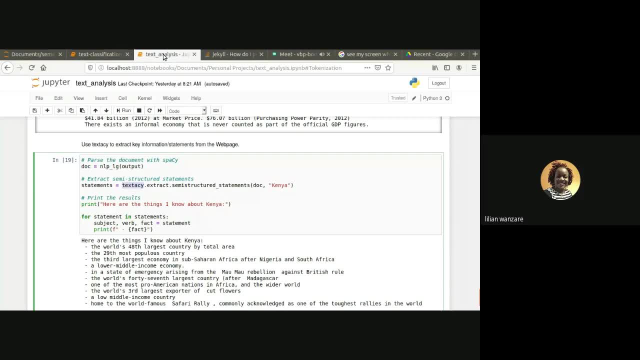 The same email is about I don't X topic, So this email has more than one tag. I'll get what you're referring to. Okay, We're trying to classify reviews. A review is about, let's say, uh, Safari com bundles. 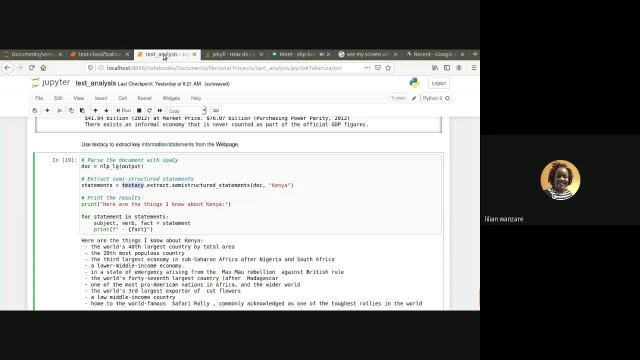 A review is positive. A review is, uh, um, urgent, So that means one particular text has many tags. Okay, I'll get the correct interpretation of your question. Okay, So that is called. So this, what I've done? is this a two class problem? 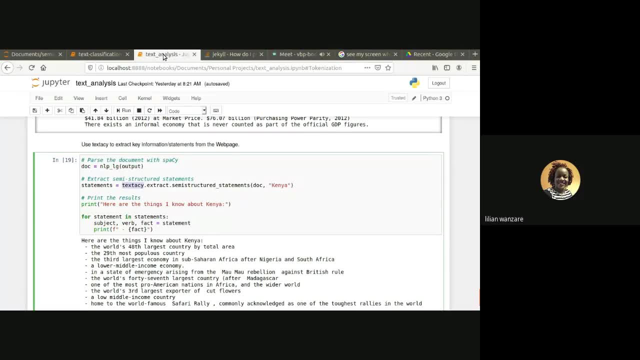 Okay, The true Positive: They are not for them, but in real life there are many things that have multiple water levels. The only thing that changes is is your, uh, how you pass it to your model. Okay, So in your modeling part you don't just pass one um, output one tag. 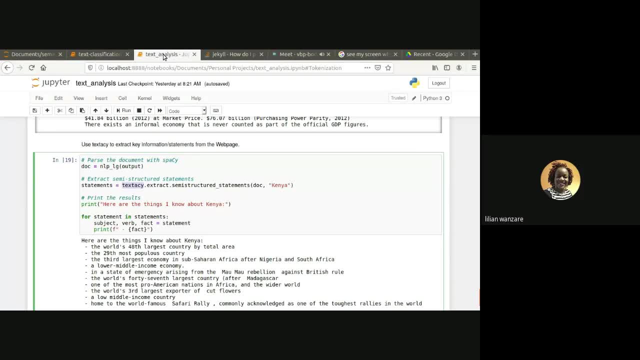 Okay, You pass several tag and there are different techniques. Okay, One of them is called one versus All or one versus rest. What it does is this behind the scenes: Okay, Instead of building one classifier, it builds 10 classifiers, depending on the number of classes. 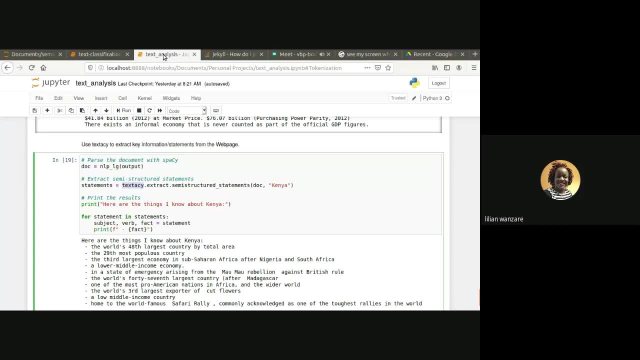 If you have 10 classifiers, every classifier gives a prediction for your data and the output becomes, for instance, one zero, zero, zero. It means that one is there. There was a lot of water there. I would be one zero, one, zero. 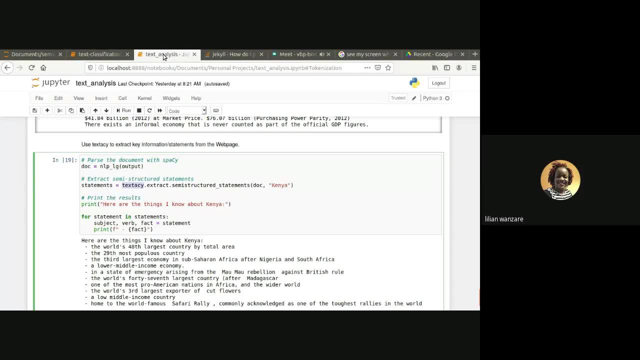 That means one and one are there. There was zero. There's a lot of water there, Okay. So, yes, what changes really is how you kind of define, uh, the model. Okay, That is called a multi-class, Okay. 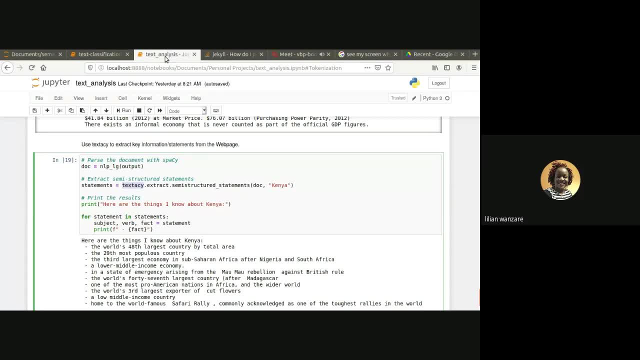 So there's multi-class and there's multi-level. So multi-class, it means you have many classes, but each data has only one level. Multi-level means you have many classes and every document has a possibility of having more than one water tag. 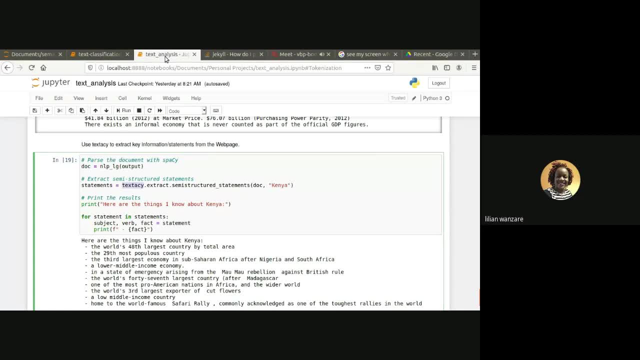 Okay. So if you're looking at the multi-level problem, it's more than one tag, Okay Okay. Okay. So you have many classes and then multi-class is just many classes, but every document has just one water. So, yes, there are tools for that, but are not covered in this, completely not covered here. 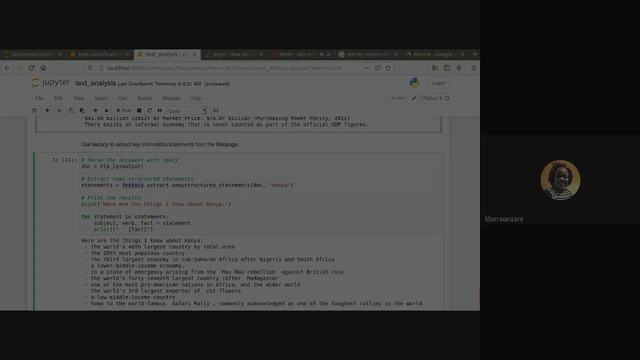 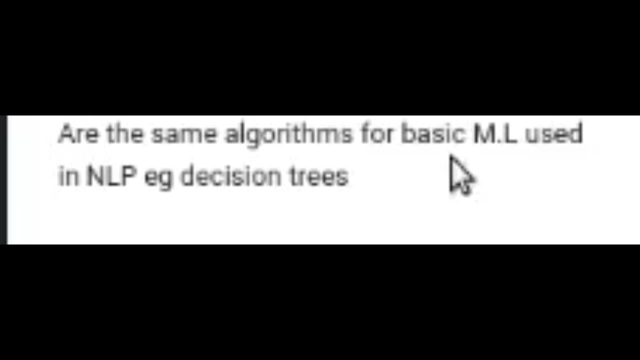 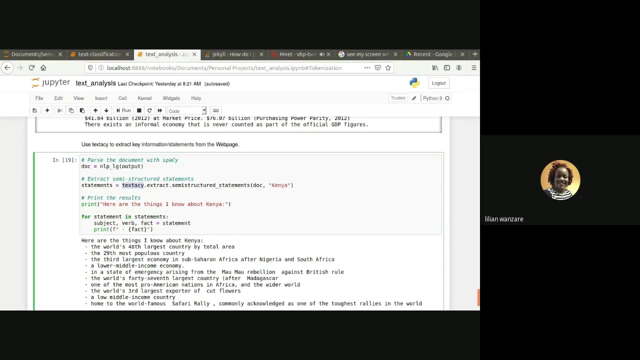 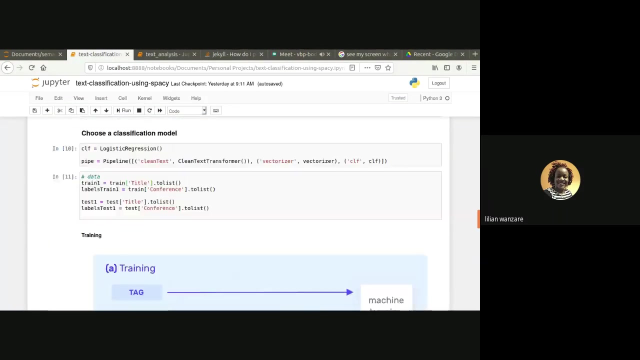 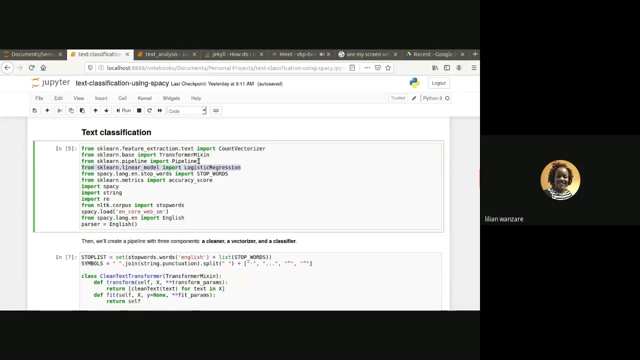 But they are there, Yes, Okay. Then Stephanie is asking: are there are there same algorithms for basic machine learning used in MLPEG decision trees? Yes, So like for example in our example. Yes, So like for example here when I do the classification. let me just show you here: when you're defining your model, okay, you go to split lines. you can actually replace this line in any model, a decision tree, a Bayesian kind of naive based model support vector machine. you know any model that is able to do classification? of course, not any, but within the classification model.